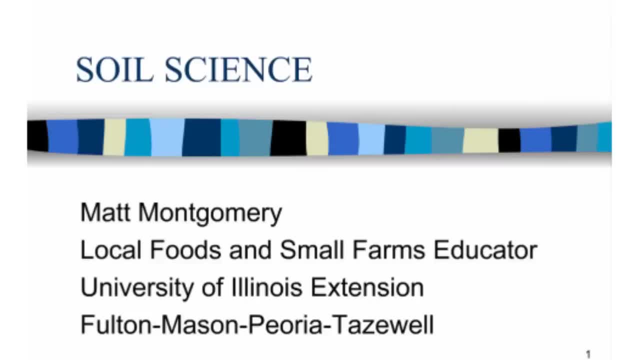 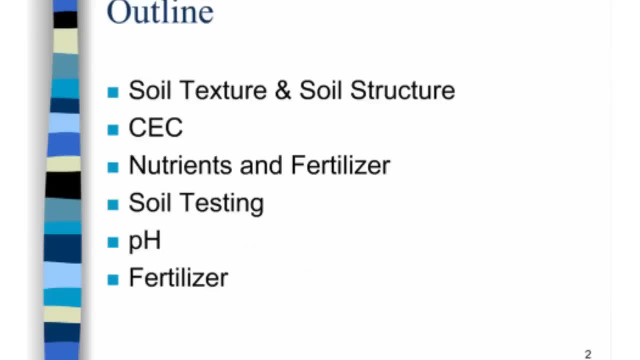 There may be a moment where you wonder: why are we talking about this, But I promise you the majority of this is going to be applied. Let's go ahead and advance to slide number two. If you're watching just on the computer, and this will be the outline for today, talk. 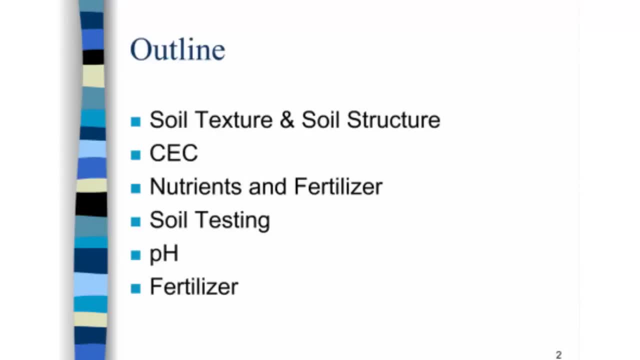 about soil texture and soil structure. We're going to talk about cation exchange capacity. We're going to talk about nutrients and fertilizer. We're going to talk about soil testing. We're going to talk about pH, And then that last point should be: we'll talk about some of 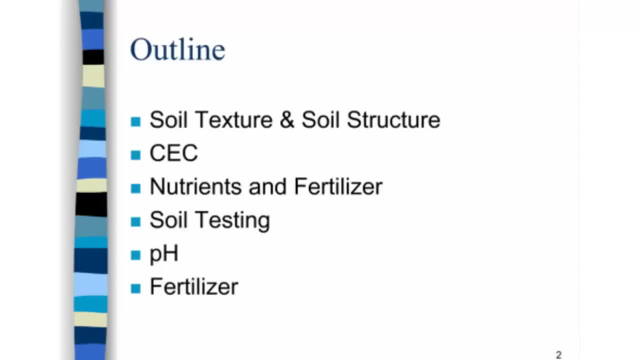 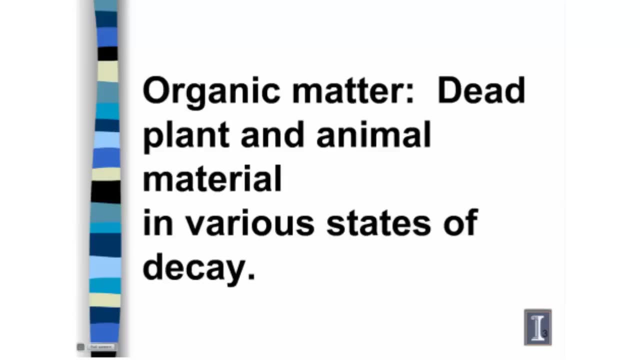 the pluses and minuses of organic versus inorganic fertilizer. Advance to the next slide, Slide number three, please. This is a descriptor that I think maybe you want to keep straight for today as we talk about soils, And that's this definition. 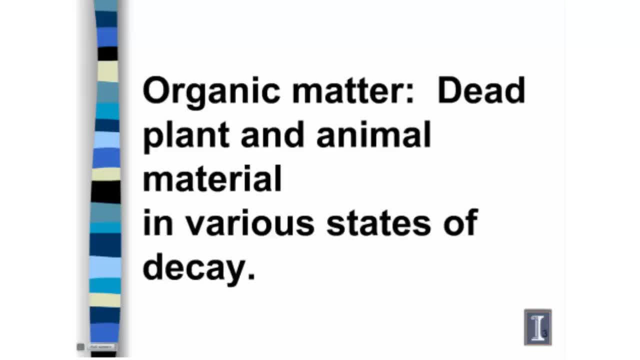 of a term we call organic matter. What I want you to remember today as we go through the presentation is that organic matter is just a fancy word for dead stuff. We like dead stuff in the soil, believe it or not. A dark colored soil has lots and lots of dead stuff. 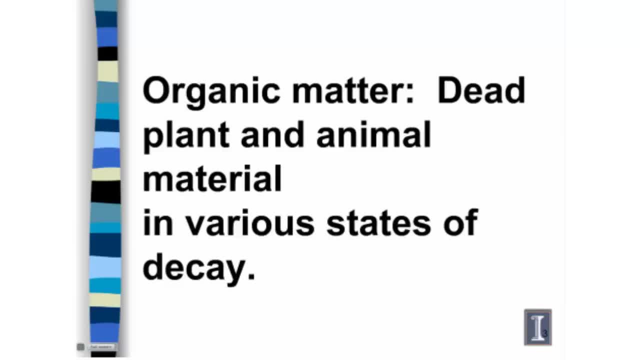 in it. That's really important. We'll talk about why here in a second. A light colored soil still has those little tiny pieces of dead stuff in it, but not as much as a dark colored soil. Let's advance to the next slide, please. At slide number four there's also a few other. 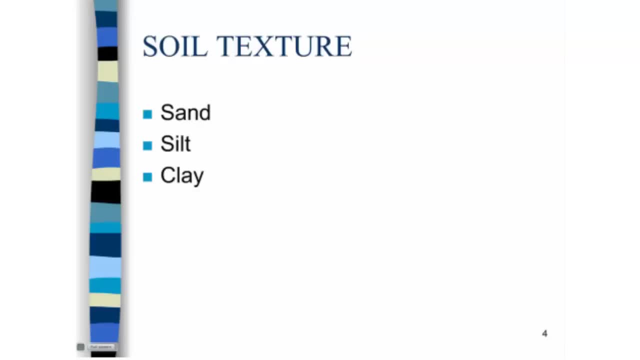 terms we need to get used to today. One term references particle size. So if you think about the different particles that make up our soil, remember that your soil is composed of both the living soil and the dead soil. If you're thinking about soil and land, and 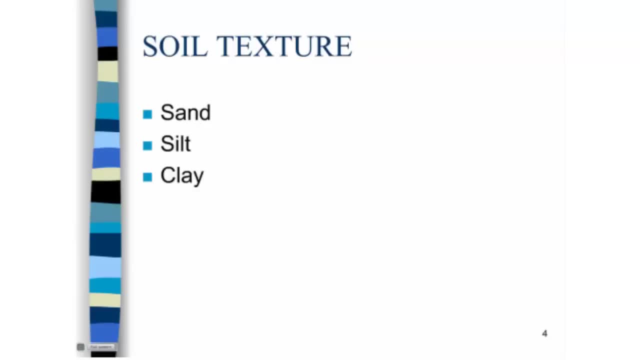 and non-living component. So let's talk about the non-living component here. Let's talk about particle size. We have three different particle sizes. We have what we call sand, silt and clay. Everybody's been at least somewhat exposed to those terms. I don't need to tell you that sand 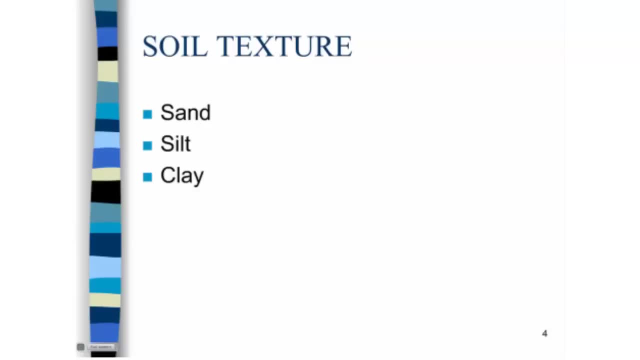 is the largest of the particles that are there. You can feel it, You can feel the grid of it when you move it through your hand. If you advance to slide number five, you'll see kind of my picture of that. You've got clay which is basically microscopic, and then you've got silt. 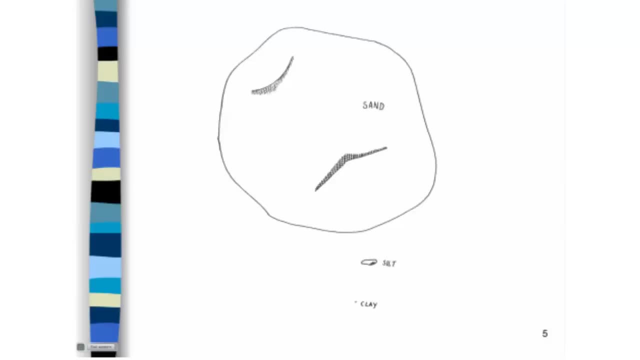 which is this intermediate-sized particle. Let's advance to the next slide. This is slide number six. There's a colleague of mine who's probably listening today from over in Quincy, named Mike Rogge, and Mike is notorious for asking a very important question. So what? Who cares? Why do? 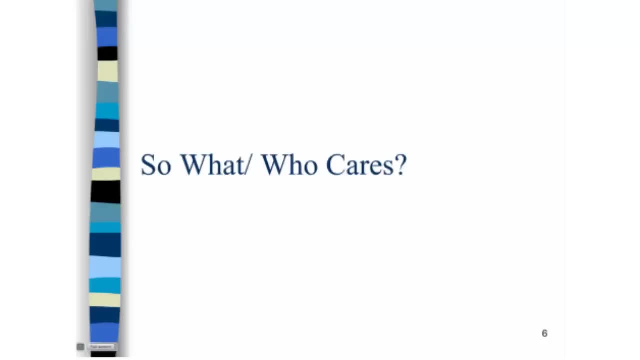 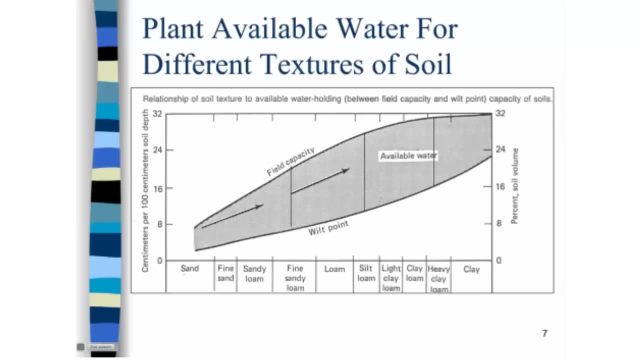 we care about organic material? Why do we care about particle size? Why do we care about particle sizes? Why is that even important at all? Well, let's advance to the next slide. And one reason that that gets to be important is that particle size influences water holding. 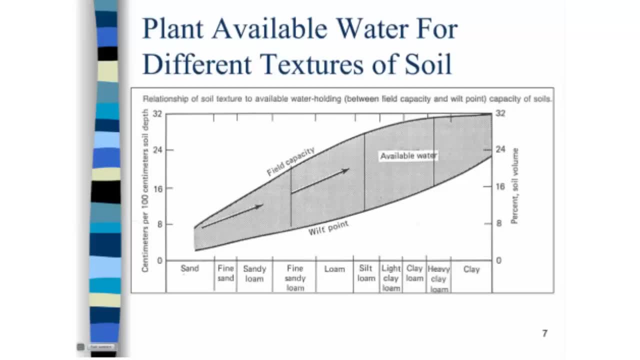 capacity, in particular plant-available water holding capacity. All I want to point out here is the dark-colored region on this graph on slide number seven. as it increases in width, that's an increase in the amount of plant-available water. As it decreases in width, that's a decrease in the amount of plant-available water. 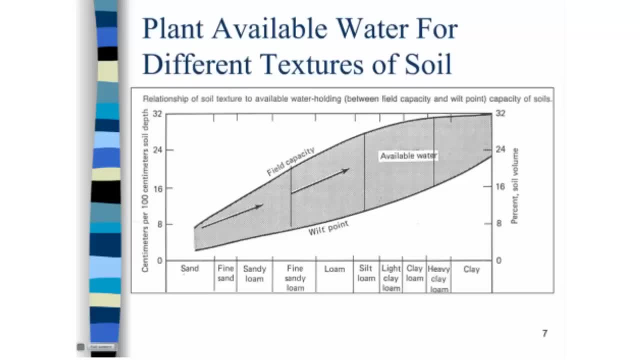 Now you look at this slide set and you notice something kind of an interesting trend that begins: We have very large particles, We don't have a lot of plant-available water, and that makes sense. I'm over here in Mason County. We have soils that are really sandy in nature As a 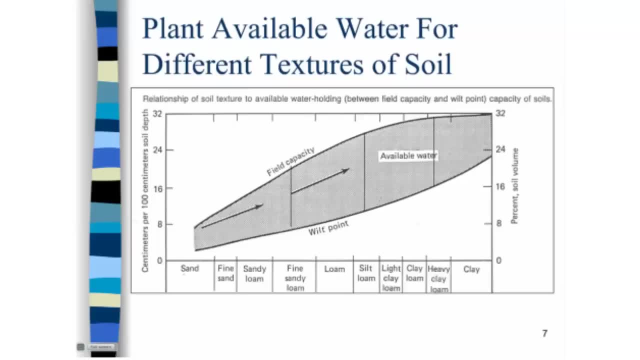 matter of fact, we just had an irrigated growers meeting this morning- our producers that raise on our sandy soils. over here We have a lot of soil that's really sandy in nature. We have a lot of water that's deposited- even irrigation water that's deposited on that soil actually percolates. 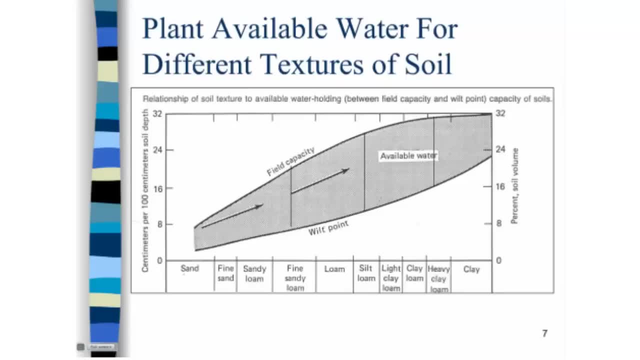 right down through those large pore spaces in between those sand particles and goes right back down into the aquifer- The Muhammad Aquifer is the name of the aquifer we have over here. Then you'll notice on this graph as those particle sizes decrease in size as we approach. 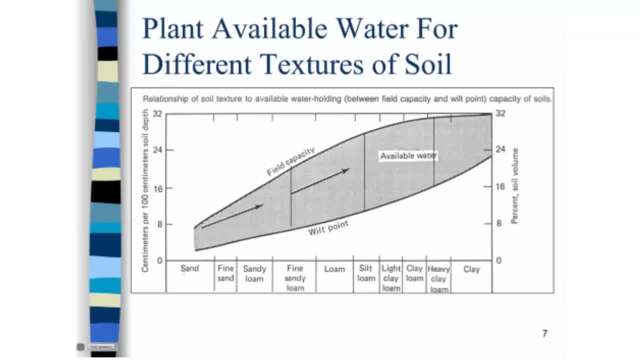 what we call a loam, which is basically an even mixture of sand and sand. We have a lot of sand, silt and clay. we have a whole bunch of water that's available to the plant, but then an interesting thing happens after that, as we get even smaller the amount of plant available water. 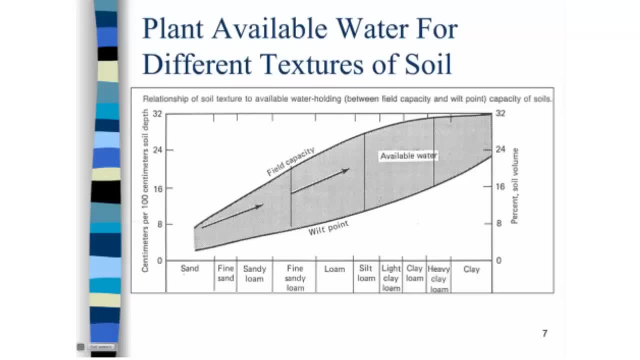 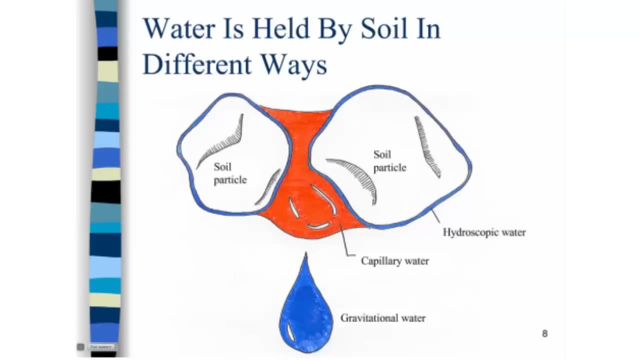 goes down now. why is that? let's advance to slide number eight, and that's because this is a picture i drew a few years ago that actually they included in the master gardener manual. that's because water is held by the soil in different ways are. so what's going to be coming up here in just a second? 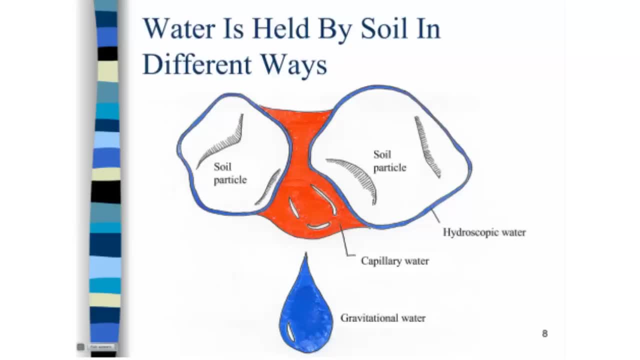 and i'll explain why this is important. we have gravitational water. that's basically the water percolating right through those sand particles and going back down into the aquifer, like we have here in mason county, in southern tatswell county. we also, though, have something called capillary water. 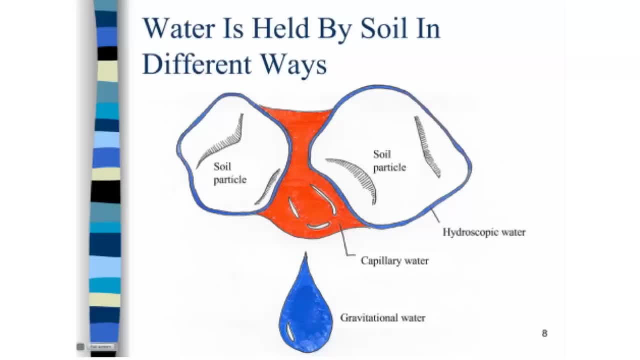 the electrical forces on your fingertip are actually stronger than the force of gravity. if you are, stick your finger and your two fingers in a glass of water. you can hold a bead of water against the entire force of the earth pulling against it by those little electrical forces. 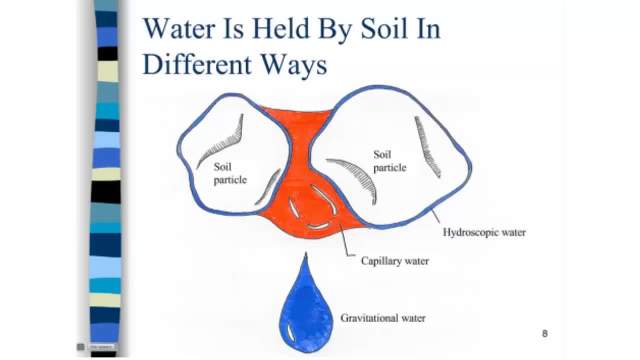 on your fingertips. that little bead of water is basically what happens in the soil. we have all these little beads of water held in between these little little pore spaces, and a root can go right in there and just suck that stuff right out. the plant can use that, it can tap into that and use that to meet its moisture demands. 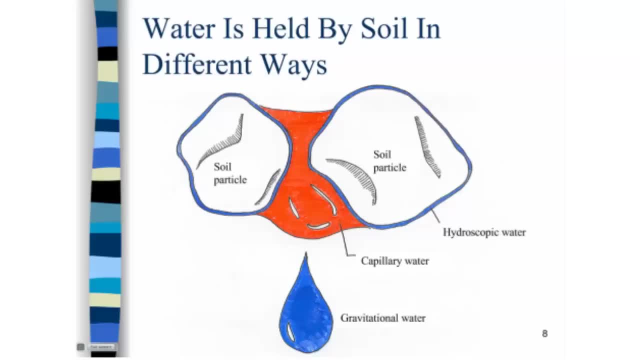 if you look at the other type of water, though, there's something called hydroscopic water, and that is a microscopic film of water so tightly held by those soil particles that you have to basically cook the soil to get this stuff off. as a matter of fact, you send in a soil sample to a 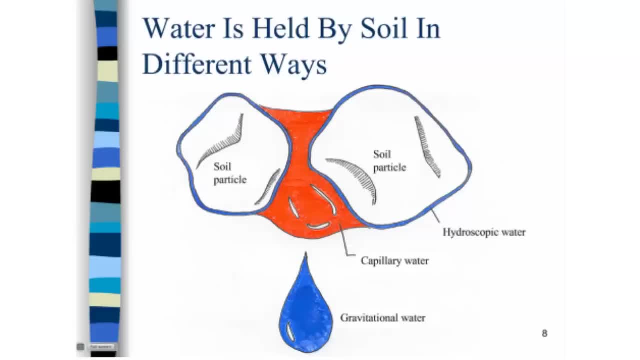 soil testing company. that's one of the things they're going to do. they're going to cook that soil sample to burn off all that hydroscopic water so they can figure out what the actual mass of that soil sample is. otherwise, they're going to have to cook that soil sample to burn off all that. 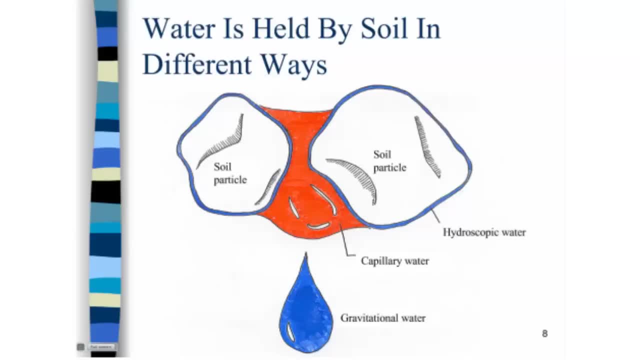 they'll get the mass of that soil sample plus this little bit of water that can't be pulled away. the thing i want you to remember about that is that this little microscopic film of water is so tightly held by those soil particles that a plant root cannot pull it away. that is plant, that is. 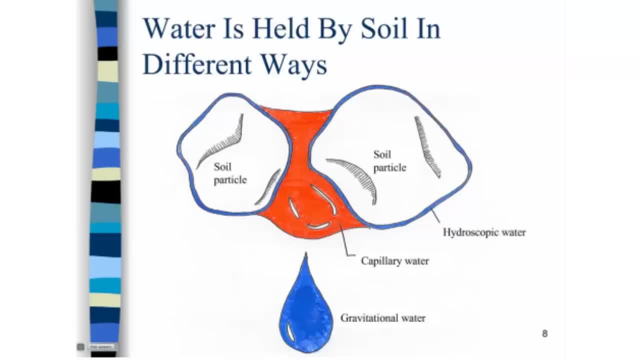 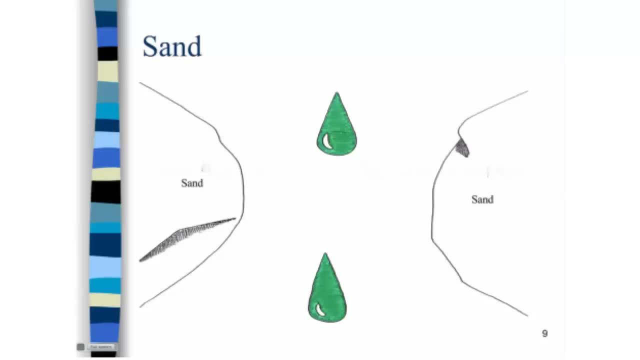 water that is not available to the plant. so if we advance to the next slide- slide nine- there's a picture of our sand, those large pore spaces, gravitational water right through it. advance to slide number 10. here's our capillary water and a lot of silty soils. we have a lot of. 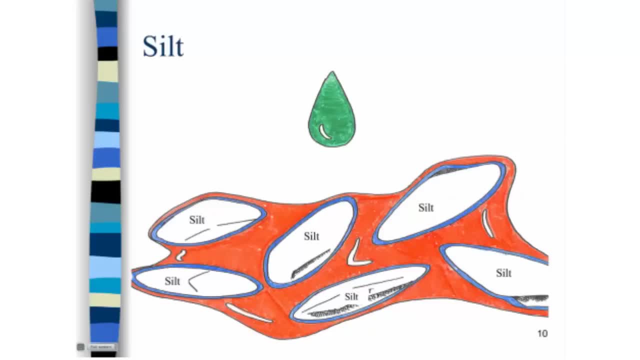 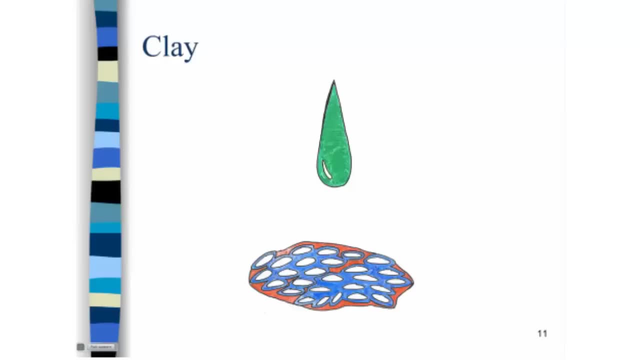 capillary water, these little beads of water that the root can tap into. and in slide number 11 we have a clay soil and those clay soil, those clay particles are microscopic and jammed together so closely that the majority of the water there are, these little thin films that are too tightly. 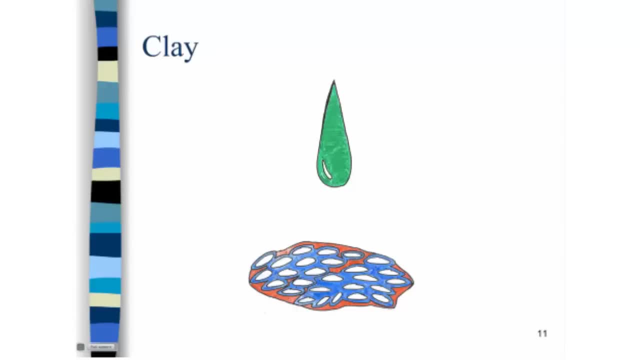 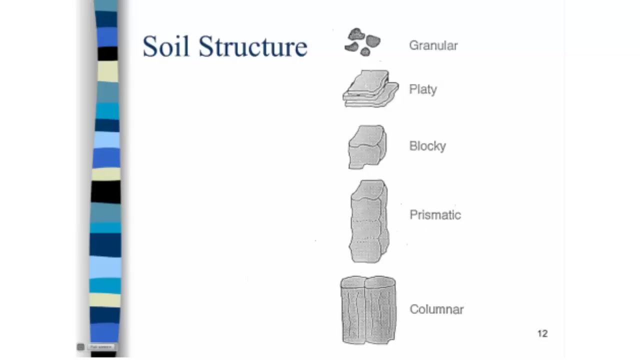 held by those particles. it's this hydroscopic stuff that the root can't pull away. so you can see how, for instance, a clay soil may have some moisture there, but those plants on a clay soil start to show stress. let's advance to the next slide. these little particles are arranged. 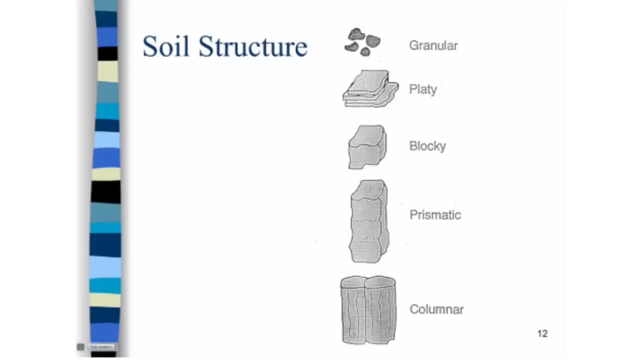 into much larger bodies. so think about these little particles as being bricks, for instance, and then we have something called soil structure and that would be the homes, the houses that are built out of these bricks. so we have these little particles- sand, silver clay- and they're arranged into these much larger structures, and you can see this. 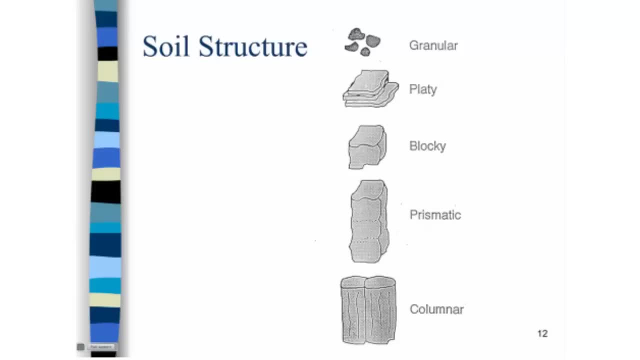 i think we all have a pretty good feel that topsoil- good topsoil- tends to be pretty granular in nature. a lot of pore space is really granular structure. then as we go into the subsoil we have these blocky structures that we see: prisms maybe that may form, or columns that may form. 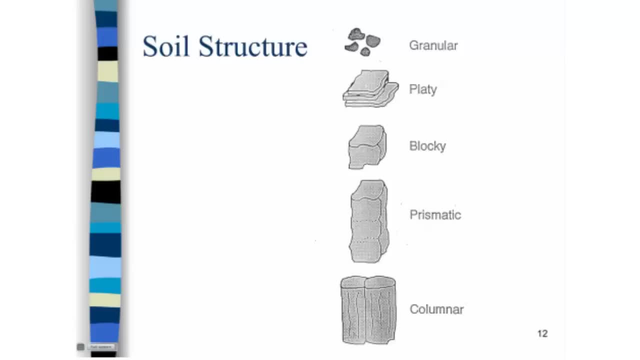 these blocks of clay that may form and you have these little jagged cracks within that, in the subsoil. we really, really, really like good soil structure. we like having these larger homes or houses that these small particles are arranged into. so let me flip to the next slide. this is slide number 13. so what, who cares? why do we care about? 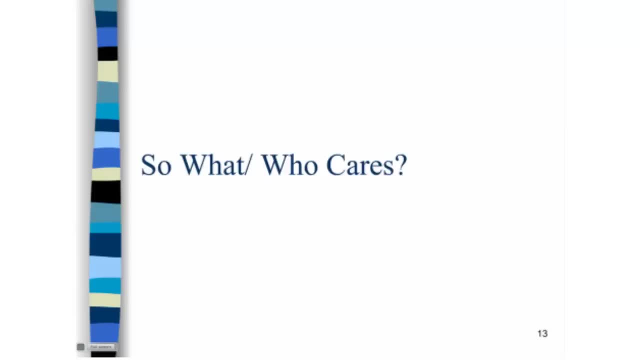 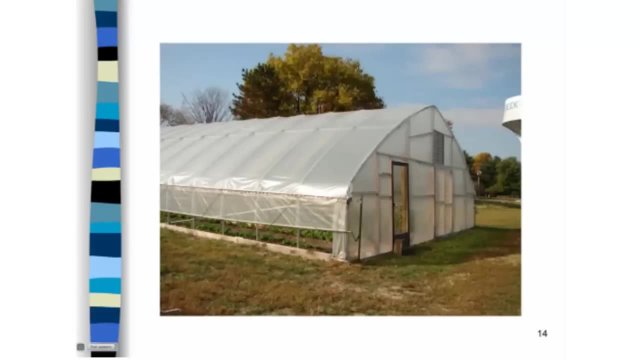 soil structure. why do we care about particle size? well, one reason is slide number 14. here you may have to click it twice at this slide, slide number 17, to see what it looks like to get that picture to show. for instance, here's a picture of my friend mike rogie, his high tunnel. 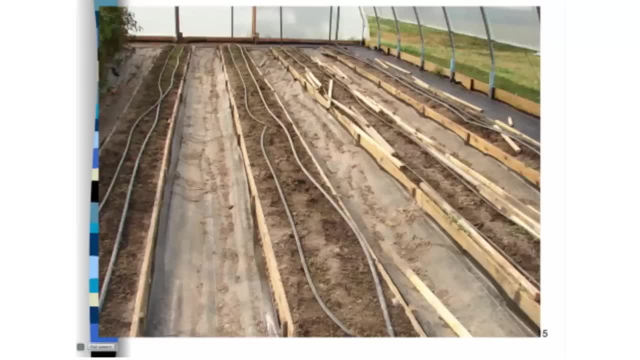 and one of the things you may notice in mike's high tunnel if you go to slide number 15 is that he has raised beds. now there are a bunch of different reasons for raised beds, but one reason people will look into raised beds is they may, for instance, have a soil type that tends to have lots. 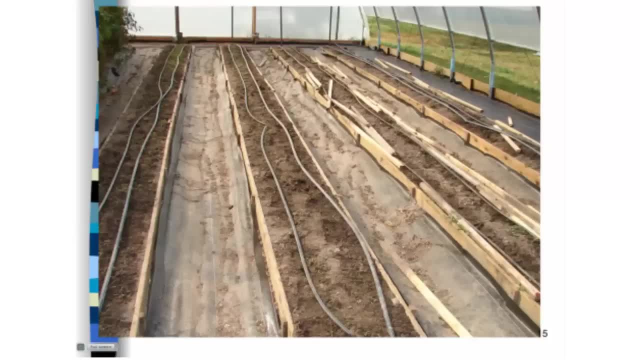 of clay, not lots of plant available water. so if they basically construct their own high organic matter granular soil there in a box on top of the ground but have a lot more water holding capacity than what they might otherwise plant available water holding capacity, There's other reasons that this is set up the way that it is. 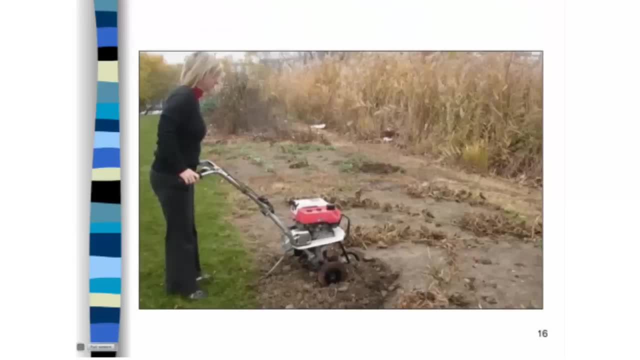 but that's one reason. Another reason: we care about structure here. slide number 16,. this is actually a picture that we used for a presentation at the specialty growers conference in January. This is just a picture of somebody rototilling their garden. It's incredibly important, as many of you know. 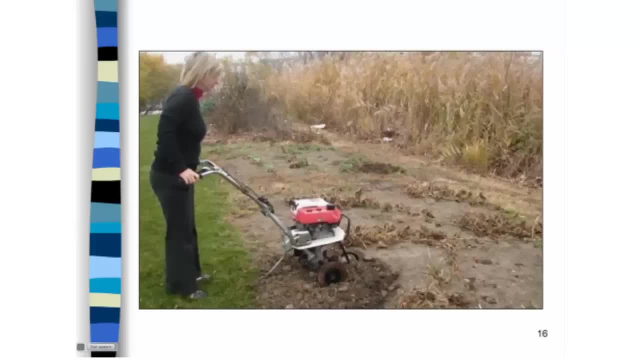 that we go out when the soil is in the right condition. So if we go out there when the soil is too wet, we start churning that stuff up and it becomes compacted, doesn't it? Compaction is basically a lack of structure. So as 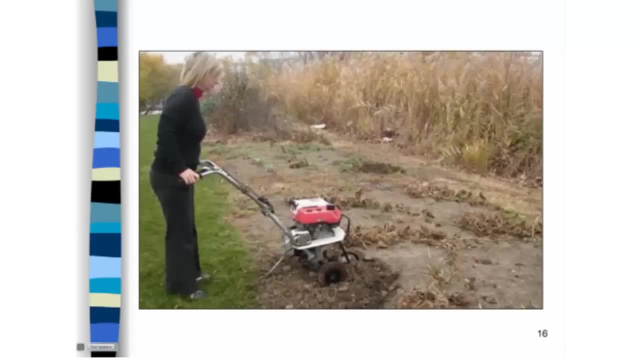 I work that soil with that rototiller when it's wet. I'm getting rid of all that structure, all these natural little cracks and fissures, and I'm just cramping that soil. I've got to get rid of it because I've got to do a lot more work. 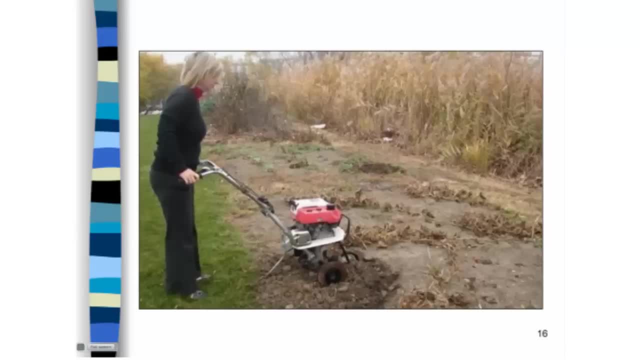 All these natural little cracks and fissures And I'm just cramping them on the other side, those soil particles together, and I'm forming concrete. This is why it gets to be important that we know about things like this, because it helps us maybe be a 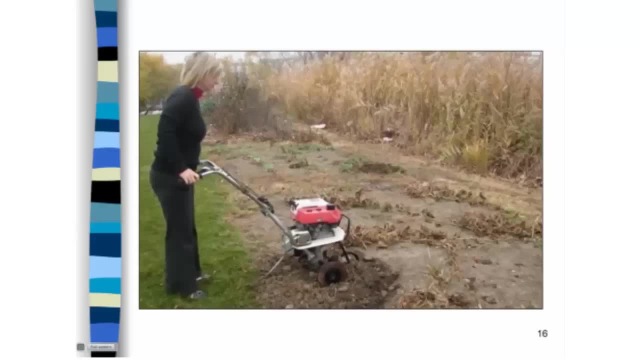 little bit more conscious of what we're doing that might compromise this desperately needed structure that helps roots penetrate, that helps water penetrate, that just really does a good job at gas exchange and those kind of things. We go out there we mistreat the soil, like in a case like this, where 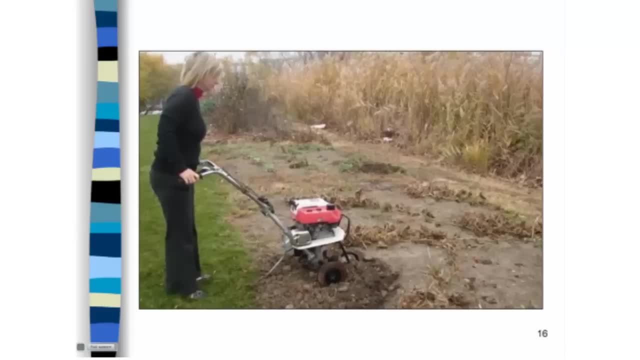 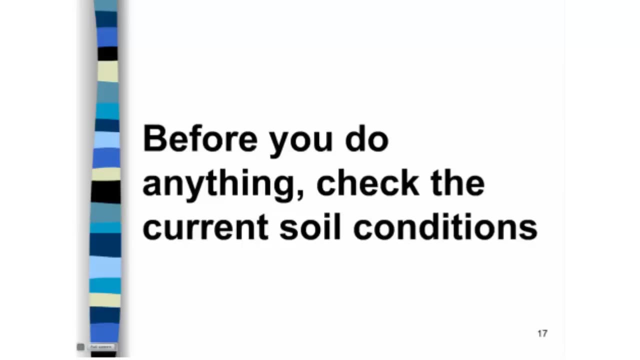 maybe we're going out when it was too wet. we're going to cram those particles together and form concrete. Next slide, slide number 17.. So that's just a good reminder, as we all know that before you do anything, you check the current soil. 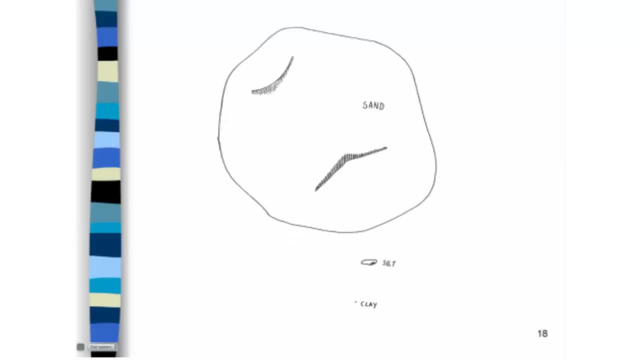 conditions, Slide number 18,. now I said just a second ago that it's very important that we know a little bit about soil particle size. I gave you some reasons why. I said, for instance, that clay might hold well for the soil to absorb in quickly. and I'm not saying that, but it is. definitely going to absorb and permeate in quickly, but it still needs a little bearing on the soil and when it does, in a sheltering and then a calaverde as exact effect, the soil gets in. So I was told, for instance, as a juniper closer to different. 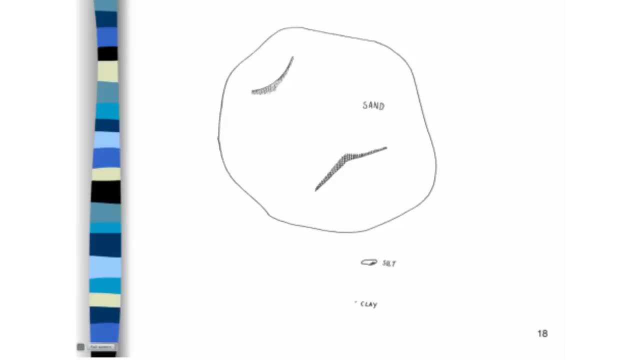 water in such a way that maybe roots can't pull that away as easily, And so maybe those plants will be under moisture stress a little bit more easy, And maybe that means that we need to pay attention. We can raise crops on a soil like that, but maybe we're paying attention if it's an area that we can irrigate. 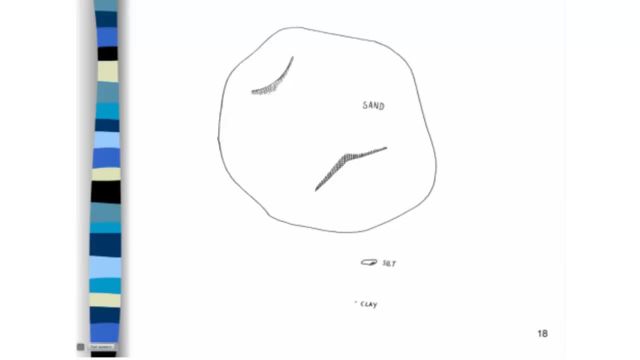 We're paying attention to the water needs of plants on that high clay soil a little bit more. But let me give you another reason. that's important: that we know something about particle size, In particular, that we know something about clay. Let's proceed to slide number 19,. so what? who cares? 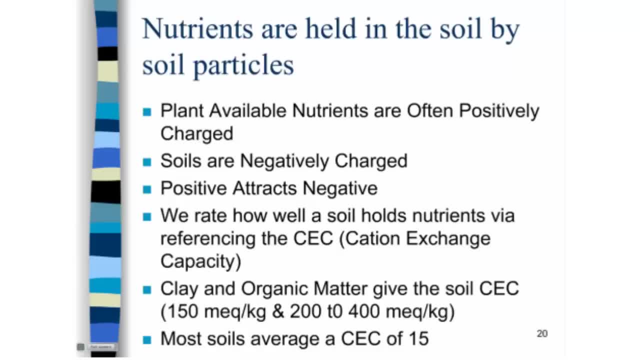 Slide number 20,. well, one of the reasons that something like clay is important is that clay, along with organic material, is really what gives the soil our ability to latch onto, to hold onto many of the nutrients that we like. Soils tend to be negatively charged in nature, right. 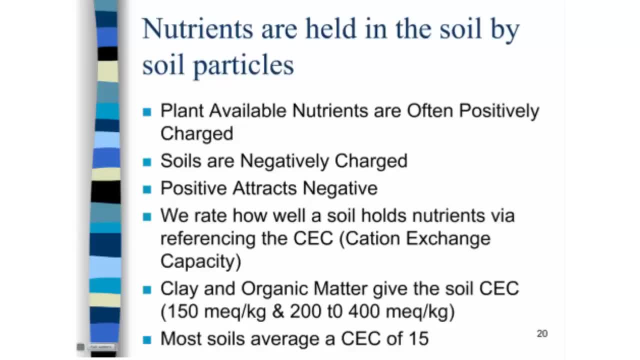 The little particles in there tend to have these little negative charges. a lot- not all, but a lot- of the nutrients we like tend to have these positive charges and it's like a magnet: Negative attracts positive, right, Those two are attracted to one another. 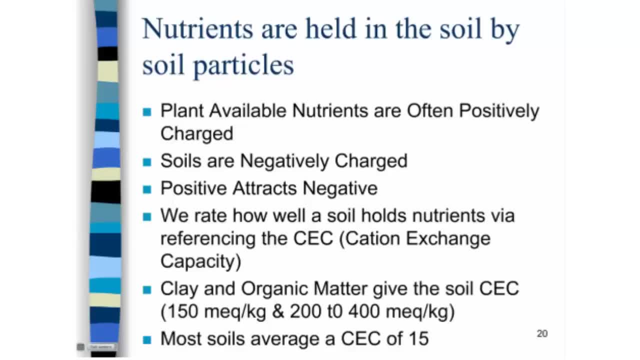 So these little negative sites that organic matter and clay contribute to the soil give the soil the ability to hold onto many of these nutrients that you and I like, And actually they grant the soil something that we rate called cation exchange capacity. Cation exchange capacity is basically just a representation of how many little negative spots are. 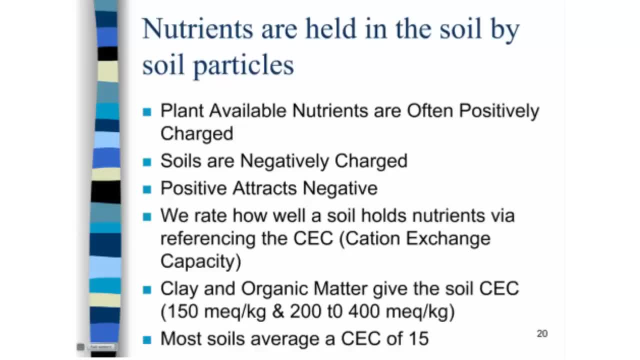 in that soil to latch onto nutrients. So clay and organic matter give the soil lots of cation exchange capacity. So one reason we like dark soils that have a lot of organic matter, a lot of dead stuff, is those soils can latch onto a lot of nutrients. 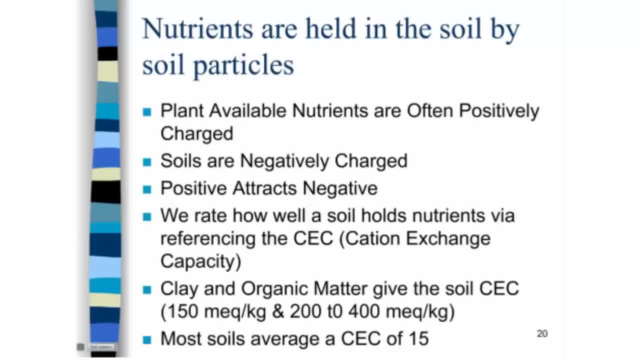 Also, we like organic material because as it decomposes it releases nutrients as well. But organic matter, it's not just organic matter. Organic matter and clay add this ability, because sand and silt don't really do that. We wind up with an average that kind of pulls our soils down to a CEC of about 15.. 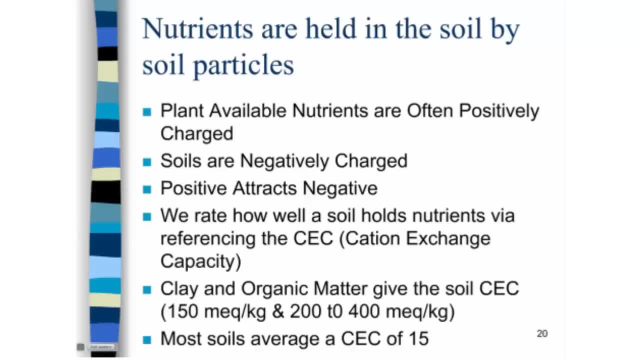 So you look at a soil test and you see a CEC rating on there and you remember this number 15.. It'll give you an estimate for maybe, where your soil is. Is it one that has lots of these little negative spots in it? 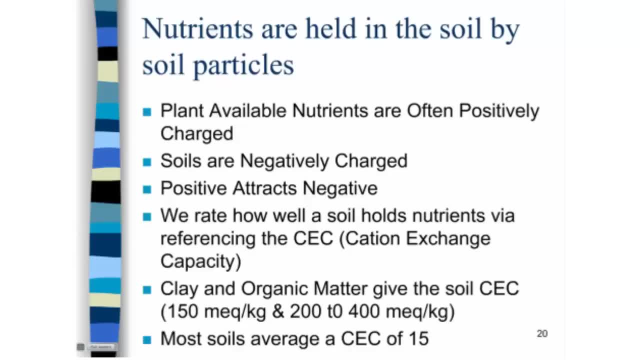 Is it one that doesn't have lots of these little negative spots in it. For instance, a lot of the soils over here in Mason County will have CECs less than 8, for instance. They don't have a lot of those little negative sites because they don't have a lot of organic matter and clay in them. 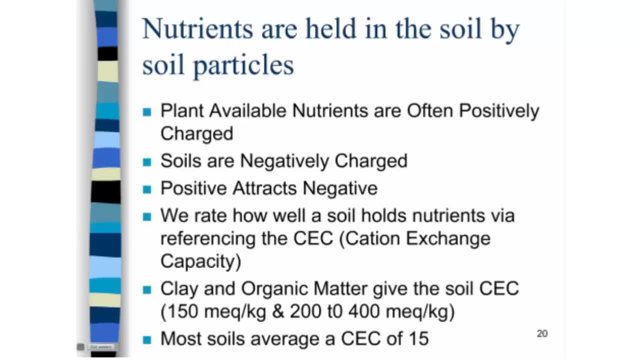 That doesn't mean that you can't raise things off of it. It has some other implications we'll talk about down the road. But let me kind of give you a description here, graphically, of what CEC does, And this will start to answer some questions now that we might have about soil tests, for instance. 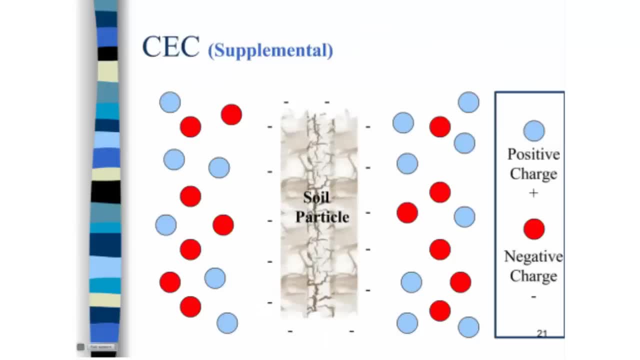 So I want you to proceed to slide number 21.. And on slide number 21 here we have an imaginary little soil particle And you can see the little negative charges all over that soil particle. That's the CEC stuff we were talking about. 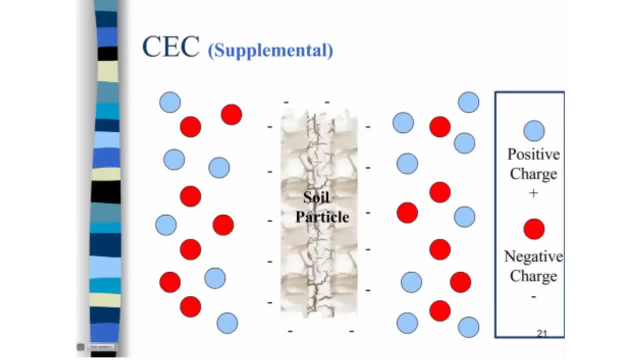 And here in this soil we also have positively charged stuff. Let's say, that's a nutrient we like, And then we have negatively charged stuff. Let's proceed to slide number 22, and you can see, we just point out those little negative charges. 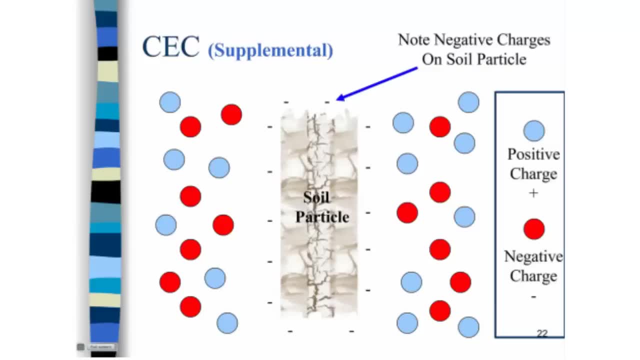 Let's go to slide number 23.. Now, for those of you that are not following us on Meeting Place, what I'm going to have you do is proceed very quickly from slide number 23 to slide number 32.. We have slide-by-slide animation that we're going to show here, and it's going to show those particles being drawn into the soil particle. 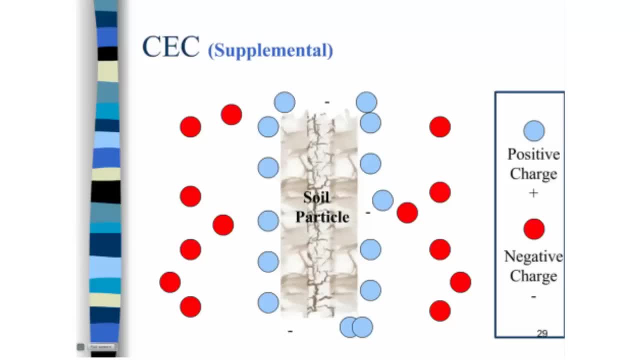 So slide number 24 and so on, I'm going to wait just a second to make sure that all of our locations- I give them enough of a time delay here to show that happening- But you can begin to see what I just talked about. 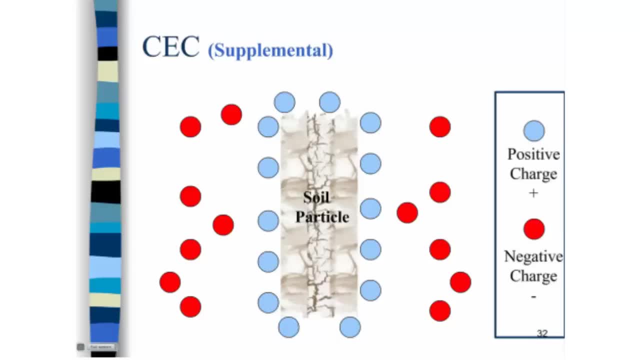 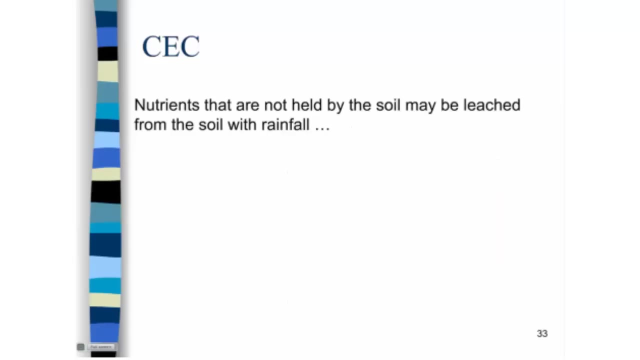 These little negative sites on the soil particle are drawing in those little positively charged nutrients and latching them to that soil particle. And now you can imagine what might be at risk for those little negative charged particles. Let's proceed to slide number 33.. 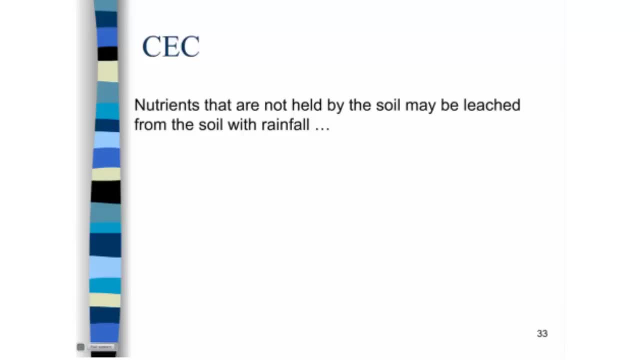 For instance, if we have those little negative charged particles sitting there floating in water or sitting there floating around in the soil and water starts to run through, you can see how basically they can be washed out, leached out of the soil profile, And that happens sometimes. 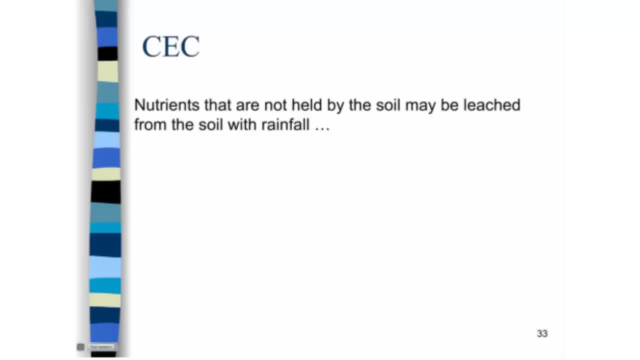 For instance, in Mason County, we will have nitrogen. We'll talk about nitrogen in a second, But we have nitrogen That sometimes is washed out into the aquifer. More often, though, what happens is- let's look at slide number 34,. 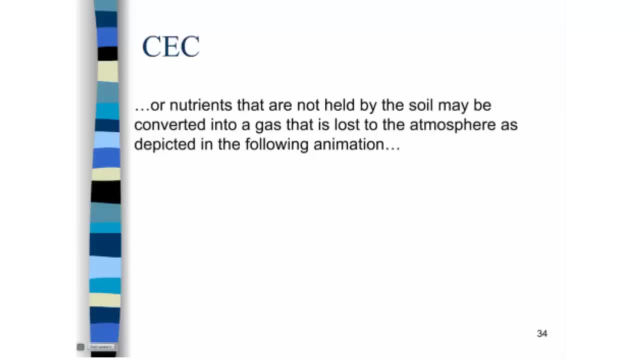 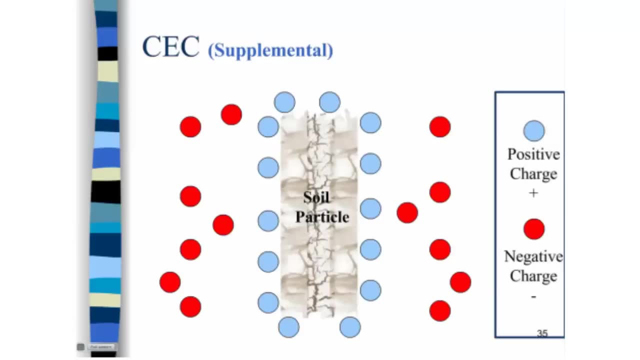 that a lot of these little negatively charged nutrients are then converted into a gas, And so let's flip to slide number 35. here We're going to do slide by slide animation. again, I want you to proceed- those of you that are clicking through this- from slide number 35 to slide number 48.. 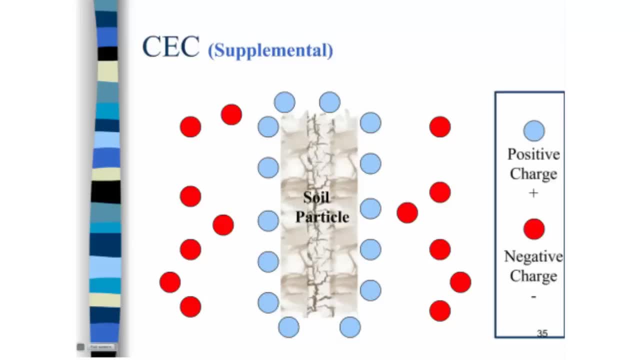 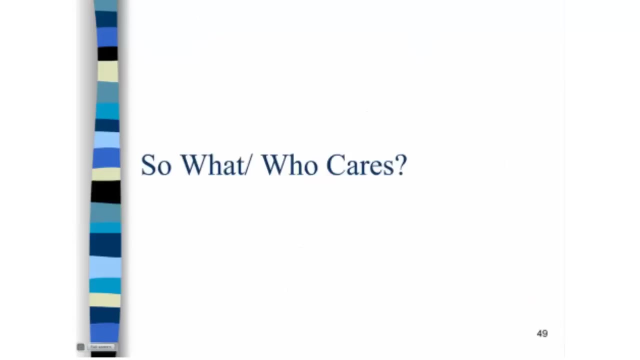 What you're going to notice is, in my little way I'm saying: these particles inflate like balloons. They change into a gas- the best way I could describe it- And they basically volatilize, float out of the soil. So let's go to slide number 49.. 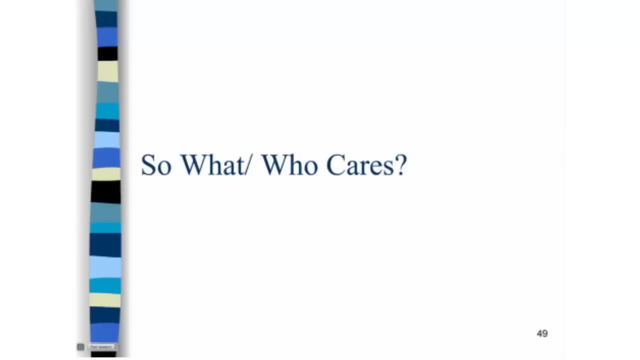 So who cares? Who cares that this happens? Why is this important? Well, it explains something. That's why it's important. It gives us a why. So let's flip to slide number 50.. Some of you are more familiar with this. 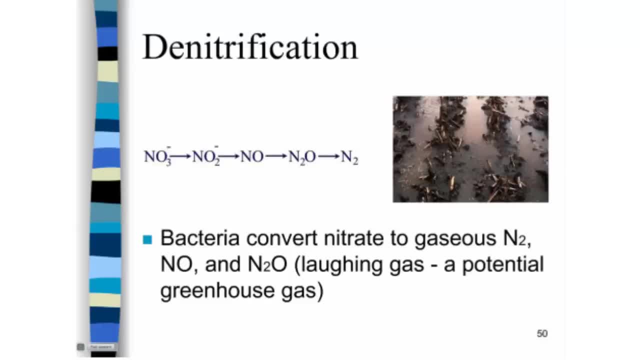 This is a slide. Some of you are more familiar with this than others, But if you look at a soil test, you'll notice phosphorous listed. you'll notice potash listed. you'll notice pH listed, but you aren't going to notice nitrogen listed. 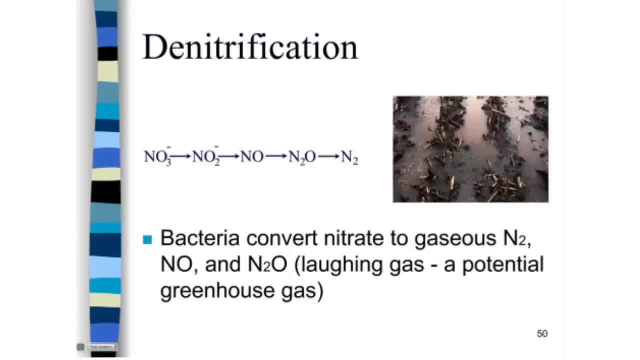 And there's a very good reason why We have something happen that's called denitrification. When we put nitrogen into the soil, at first it kind of starts out positively charged, But these little microbes get a hold of it and they start to change it into a negatively charged molecule. 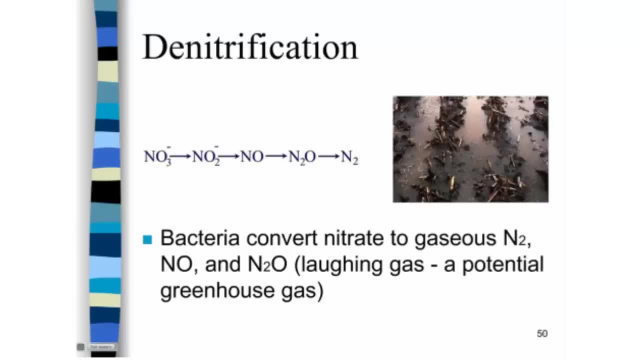 That eventually is converted into a gas- Actually into laughing gas- and is lost into the atmosphere and that's a greenhouse gas. So we lose nitrogen very quickly from the soil profile. So the amount we have here today may not be the same in just a few weeks' time, or just a couple weeks' time. 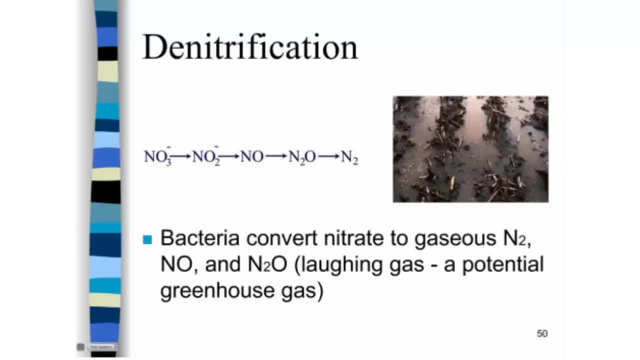 It may have actually disappeared, changed, floated out of that soil. That becomes important, because therefore, we don't mention it on a soil test, because those numbers really aren't that reliable. Another reason that becomes important, though, is you and I now have this concept that nitrogen just doesn't stick around very long. 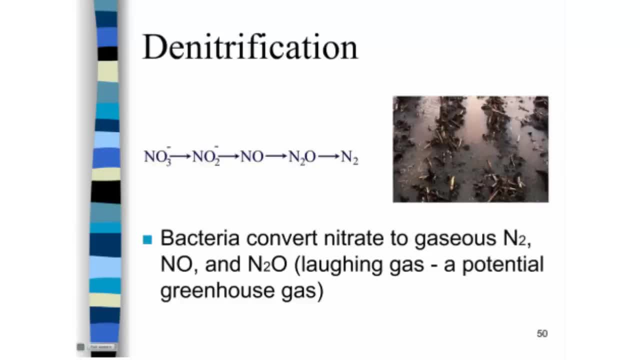 So when we talk about applying nitrogen, and we talk about applying it close to the time that the plant actually needs it. now you understand why We're applying it close to the time that the plant needs it, because it just doesn't stick around that long. 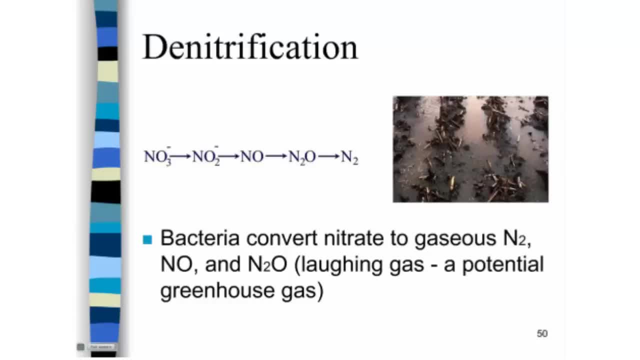 It goes to this negatively charged thing, It's converted into this gas, It's lost into the atmosphere. So we break up all this. We break up, oftentimes, our nitrogen applications to make sure we get the most bang out of that as possible. 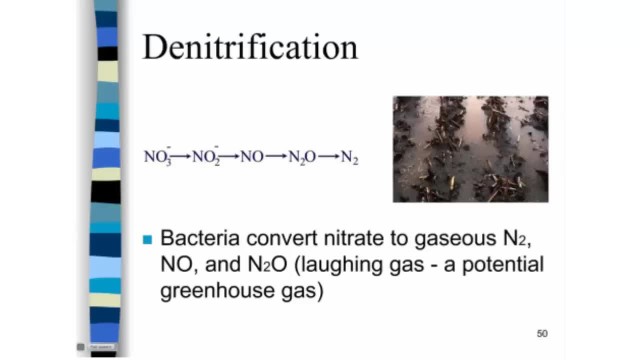 We don't want to put on a ton of nitrogen, then have that nitrogen get converted and have the majority of that lost to the atmosphere where it causes environmental problems. but it also costs us in our pocketbook. Let's proceed to slide number 51.. 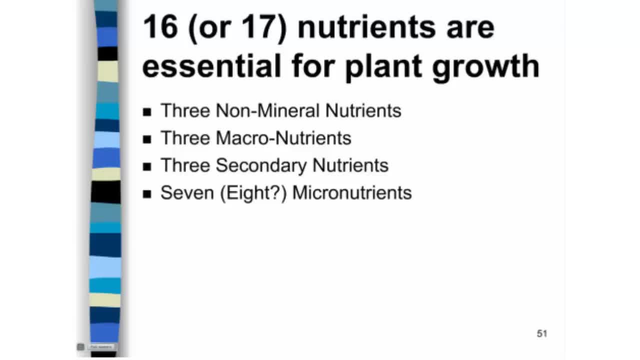 Okay, So we hinted at this. now. We talked about nitrogen. We know that's an important nutrient for the plant. If you've done anything garden-wise For a while, you know that nitrogen is pretty doggone important. but there are other nutrients that are important as well, and this is kind of a contested subject right now. 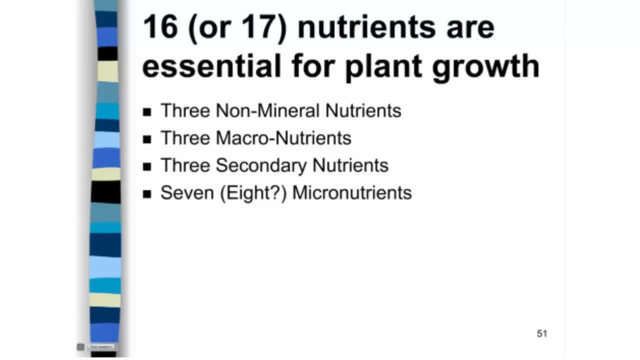 Some people say there are 16.. Other people say there are 17 essential nutrients for plant growth. We need to go through these, maybe so you become familiar with them, but also so you maybe can make some wise decisions when it comes to fertility, as you're trying to raise something. 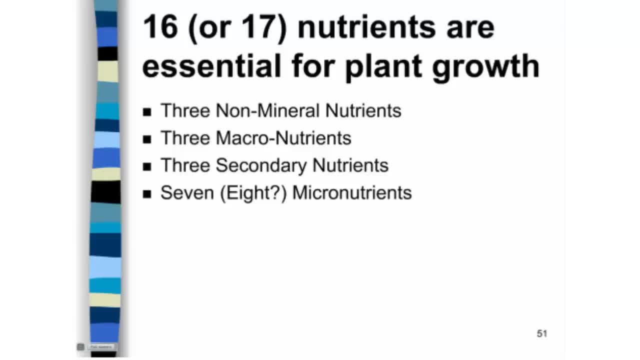 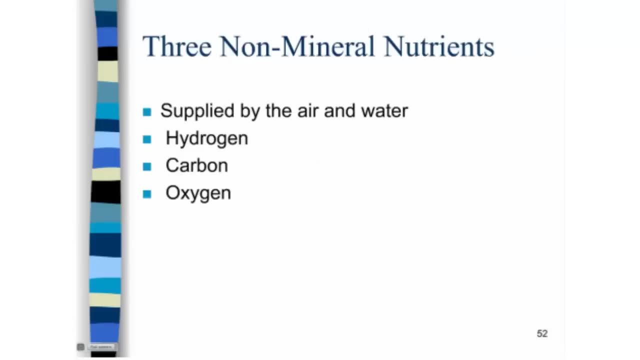 So we start out with three. We have three what we call non-mineral nutrients. We have three macro nutrients, three secondary nutrients and seven or eight micronutrients, The three non-mineral nutrients. let's flip to slide number 52, that's carbon hydrogen and oxygen. 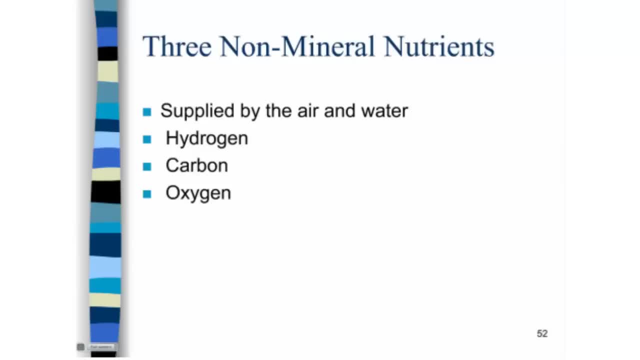 And we never fertilize with these. but if you think about it, the plant's pulling in oxygen. It's pulling in carbon dioxide. It's pulling in water. Hydrogen carbon and oxygen are in the soil. It's pulling in water. 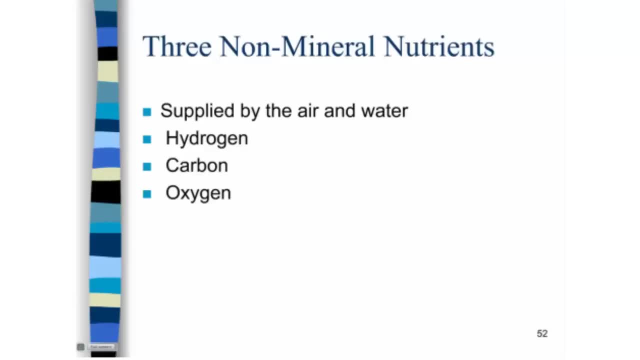 Oxygen are in some cases a part of all of those, or maybe not a part of all of those, But CO2, H2O, pure oxygen, O2, those are all pulled in And, believe it or not, the plant uses a lot of this stuff to make up its weight. 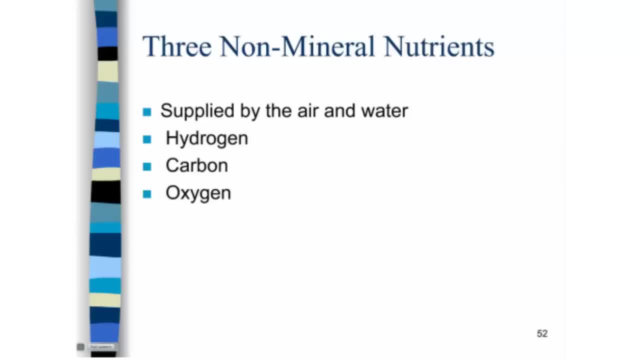 I think it's something like 95%, 90% to 95% of that plant's weight is actually this stuff that it got out of the air, that it got out of water, And so we don't worry about fertilizing for this. 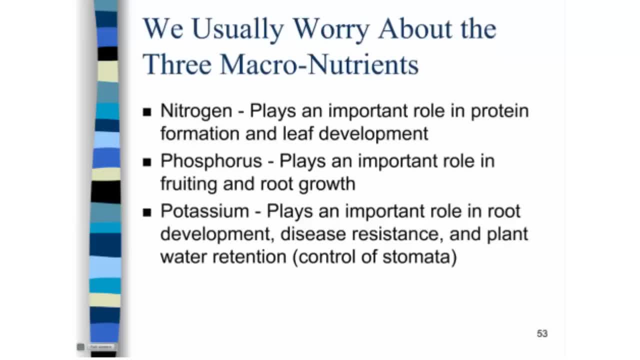 What we do worry about fertilizing. for, though we look at slide number 53, are N, P and K And you and I know- or maybe you don't and you will now- that those are the three numbers listed on the fertilizer bag. 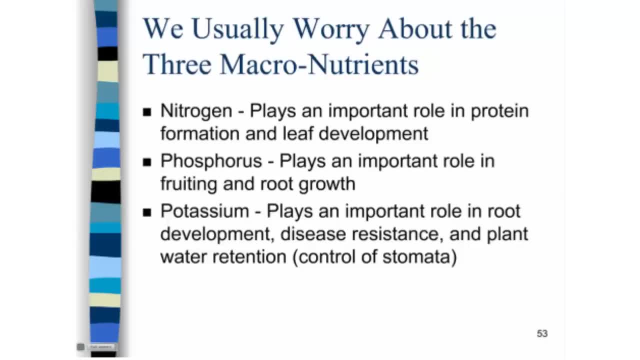 You look at the fertilizer bag, it says 10-20-10.. That's a reference to the percentage by weight of that nutrient in that fertilizer bag. Why are they important, though? Why do we worry about N, P and K, nitrogen, phosphorus and potassium? 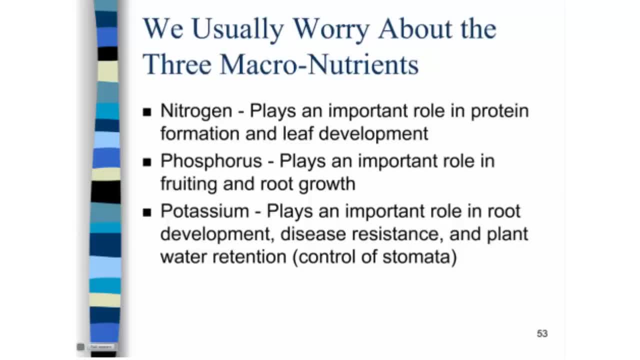 Well, number one: we worry about nitrogen because it basically helps us make building blocks. It helps us make proteins, and proteins are the building block of about just everything in that plant. So it's not going to surprise you, I don't think, to find out that nitrogen of the nutrients that aren't acquired by air or water. 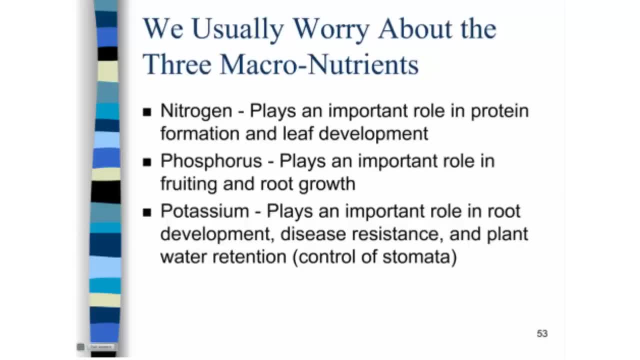 nitrogen is one of the most prevalent in that plant. I think it's somewhere close to 5%, if I remember correctly. Phosphorus becomes really important Because it plays an important role in that ability to form fruit and ability to grow roots. 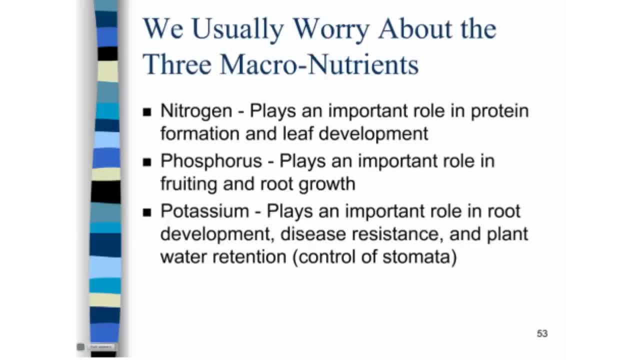 So we talk about starter fertilizers being high in phosphorus, But another reason phosphorus is important is that phosphorus helps that plant take the energy from the sun and put it into a chemical battery we call sugar. It's important to this photosynthetic process that helps us create yield and plant parts and all this. 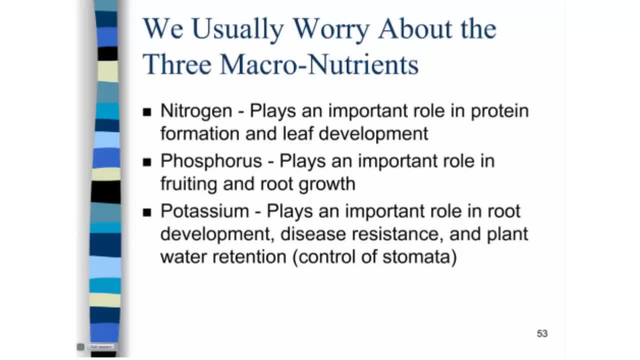 It also helps us harvest the energy out of those sugars So that the plant can stay alive, And we'll depict some of this in a second. Potassium is important. It's important in root development. As a matter of fact, I think it's the second in most crops as far as percentage by weight. 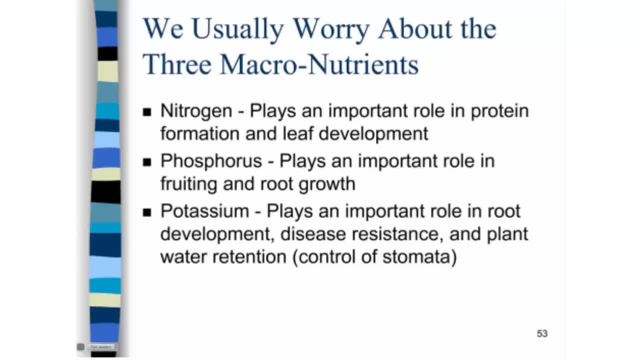 Somewhere in the order of 4% of that plant's weight is actually potash. during the vegetative stage. We don't see a lot of harvested material real high in potash, unless we're looking at something like a root crop, like potatoes. 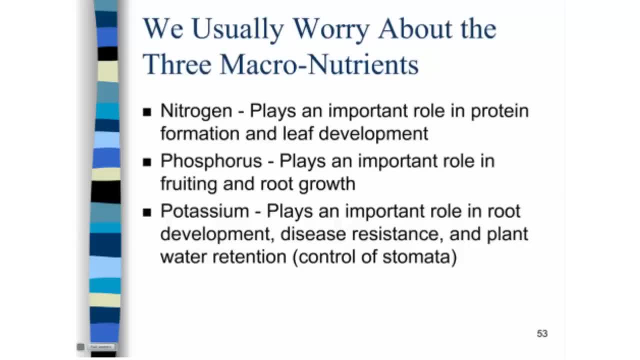 And in potatoes potash will actually make up most of that, More of the mass of that plant than it does in maybe some of our other crops that we think about, So it may pass up nitrogen. Potash is important in disease resistance. 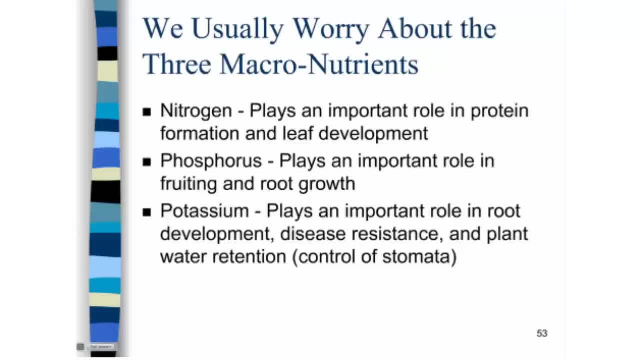 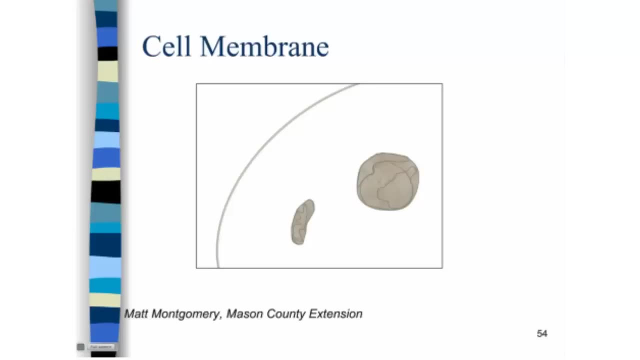 It's important in the ability of that plant to retain water. These are three very important nutrients in the plant, So let's find out- maybe a little bit better description- why. Let's proceed to slide number 54.. This is Matt Montgomery's crude representation of a plant. 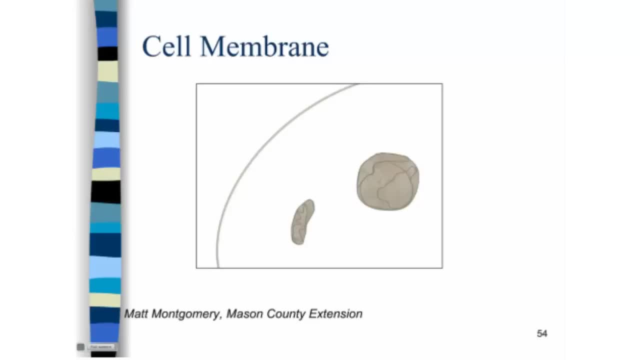 This is a cell on slide number 54 here. So you have that great big glob that's just kind of off center right. That's, I guess, the nucleus, the brain of the cell. It tells the cell what to do. Then we have the mitochondria. 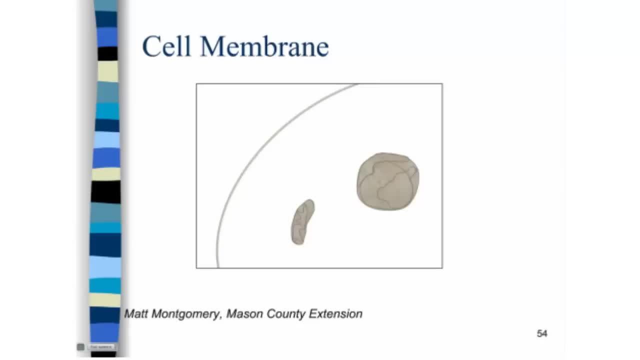 That's basically the little structure in that cell that pulls energy out of sugar to keep the thing alive. And then we have that little around the outside that we call the cell membrane. And the cell membrane is very high in phosphorus, And I'm going to show you that. 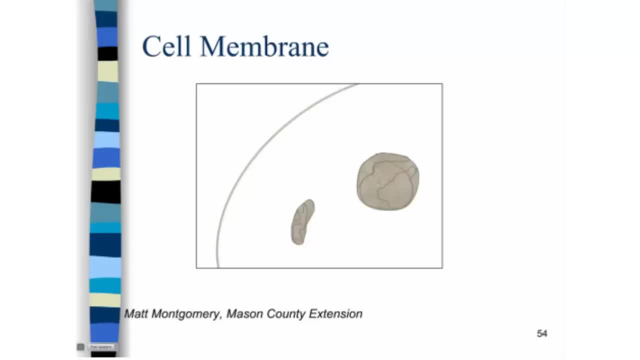 What I'm going to do. for those of you that aren't following along with me, I want you to go from slide 54 to slide 69. And I'm going to advance slides now. We're going to zoom in here on the cell membrane. 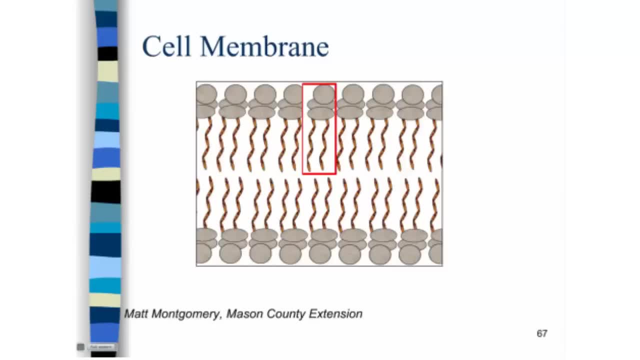 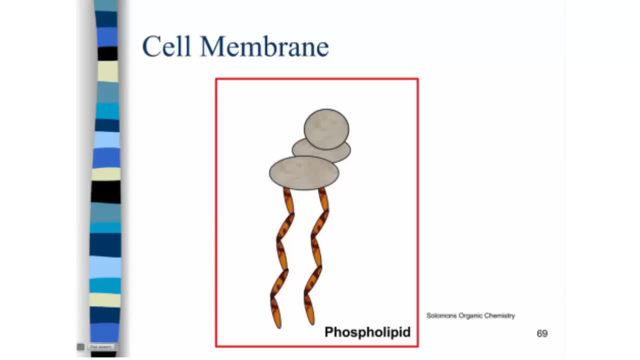 We're going to magnify it And we're going to look at these little building blocks that make up the cell membrane. And the thing you should start to notice as we're zooming in on this cell membrane is, like everything in us, the cell membrane is a lot more complicated than what it looks at face value. 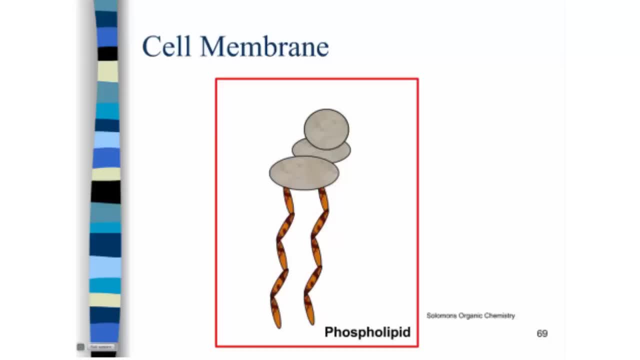 It's made up of a bunch of these little things that we call lipids. I don't think you need to remember all this. What I want you to remember, though, is look at the title of that little building block. It's called a phospholipid. 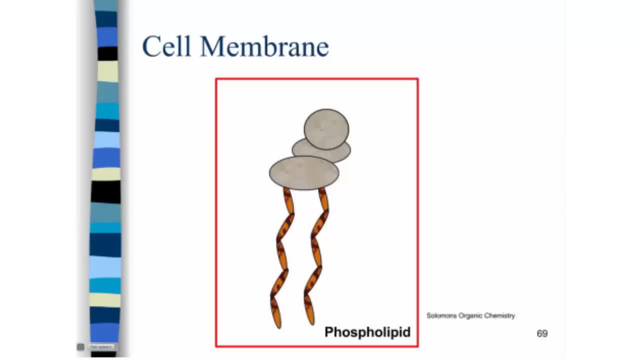 It's made up of phosphorus, And that means that if you don't have enough phosphorus, you aren't able to really crank out the cell membranes the way you need to. You aren't able to produce this. You aren't able to produce the cells the way you need to. 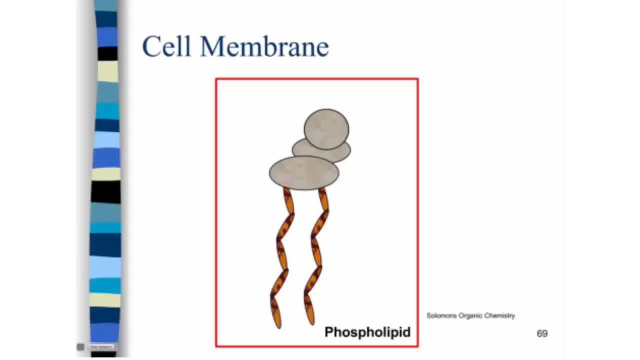 And this begins to paint a picture, I think, of why phosphorus is so important. So let's proceed to slide number 70,, 71, and 72, and 73.. So phosphate makes up the top of this thing called a lipid. 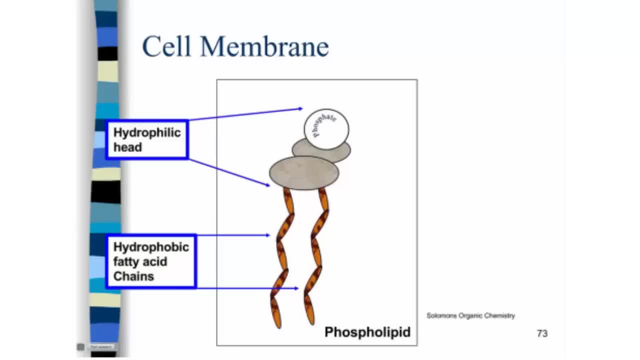 All I want you to remember: you've got to have phosphorus to make that cell membrane. If you don't have enough phosphorus, you aren't going to be able to crank out cells the way you need to. You aren't cranking out cells the way you need to. 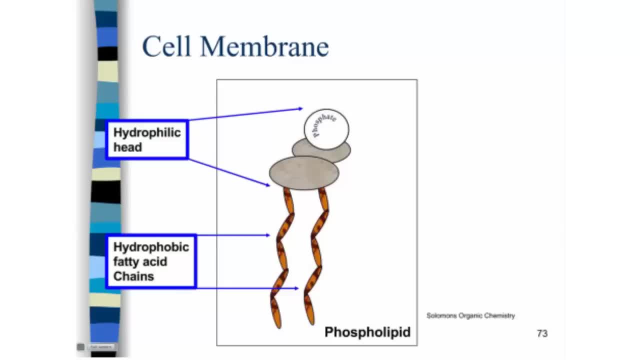 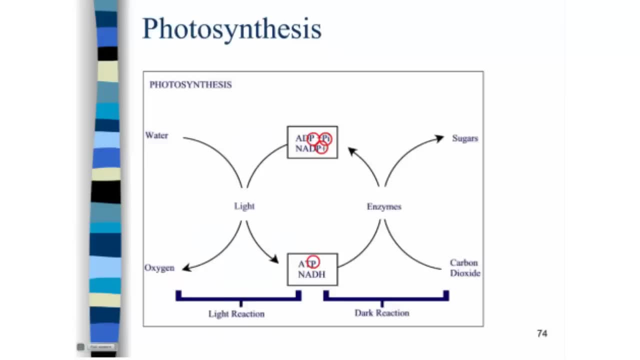 You've got big problems for that plant. This paints the picture for why phosphorus is so important. Slide number 74,. this is a picture of the photosynthetic cycle And I don't know anybody in their right mind who would try to go through that cycle right now. 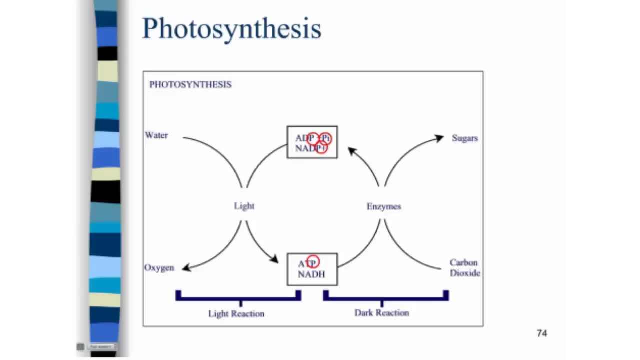 All I want you to notice is what I've circled here. The letter P is all over that thing. Phosphorus is intimately connected to the ability of that plant to take sunlight energy and make it into sugars that that plant ends up producing. 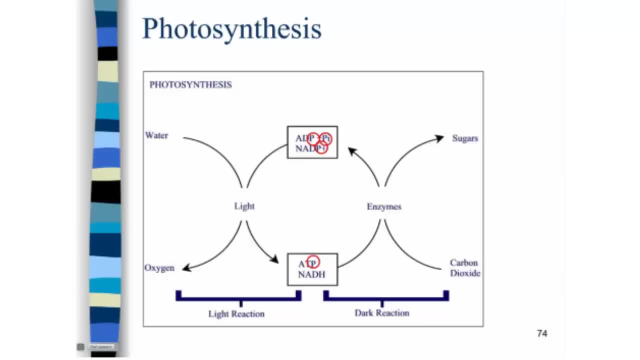 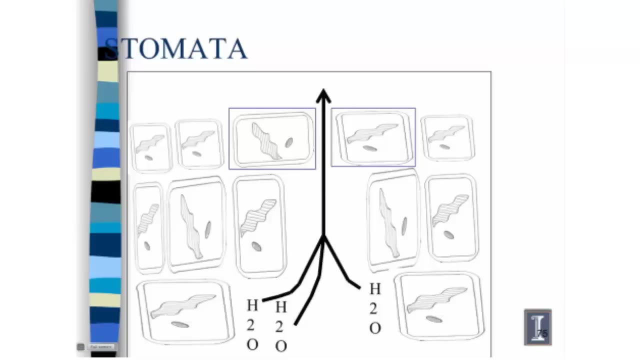 You start to rob the plant of phosphorus, you're going to have problems with it growing and you're going to have problems with it actually being able to produce sugars the way that it needs to to produce yield Slide number 75.. Okay, let's talk about potash. potassium K. 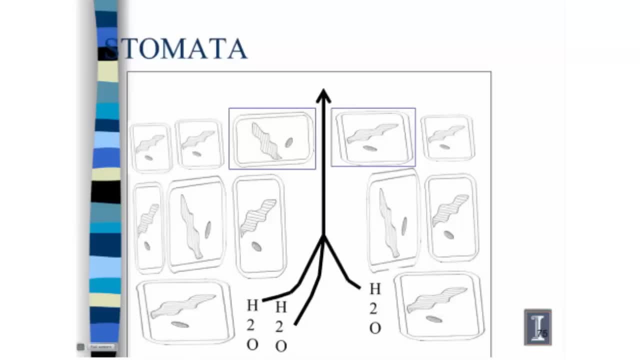 One thing I said is that potash is really important to the ability of that plant to hold moisture inside. You know, a plant basically wilts because it's low on water pressure And it's basically like a garden hose. You know, you turn off the tap on the garden hose, it becomes pretty loose. 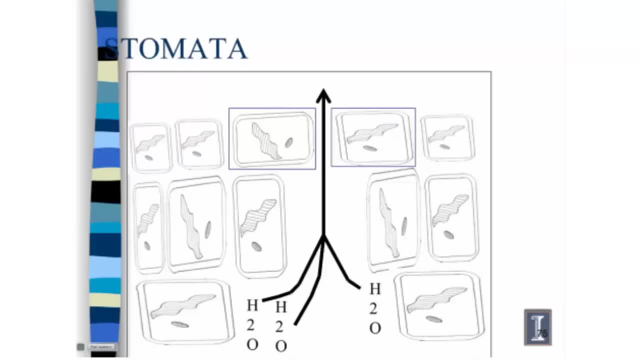 You crank on the tap on that garden hose and it firms up. You restrict the size of the opening on that garden hose and it firms up. And potash is actually loaded in little cells around openings in the leaf that act like the regulators for a little garden hose inside that plant. 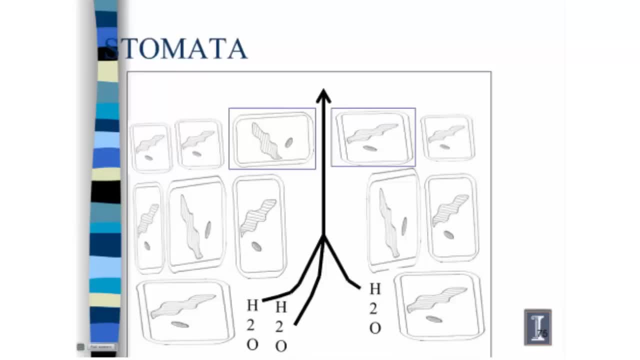 They regulate water pressure. The size of the hole regulates how much water pressure you have. Slide number 76, I think it is. It just shows how that cell pinches off. It constricts the size of that opening, keeps the water pressure up. 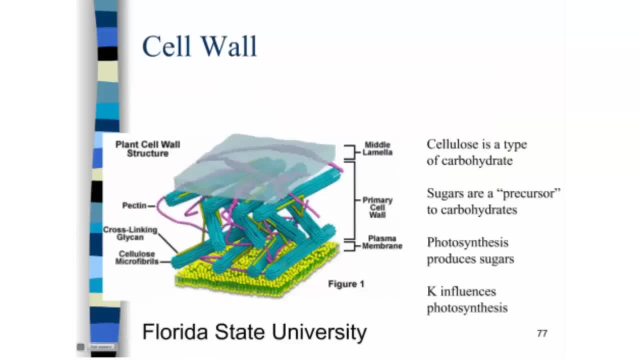 Let's look at slide number 77.. One other thing you should know about potash Potash. when you look at harvested material there's not a lot of potash actually in harvested material. most harvested material- Actually a lot of potash eventually leaks out of that plant back into the soil. 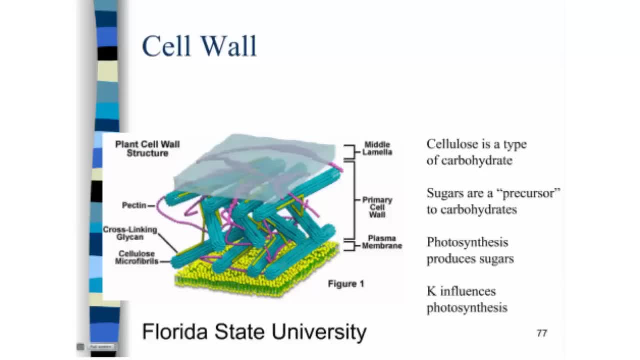 We have lots of potash floating around in it, but it doesn't make up a lot of the plants we might say that are harvested. It is important, though, for the ability of that plant. It plays a role. We're not going to describe why now. 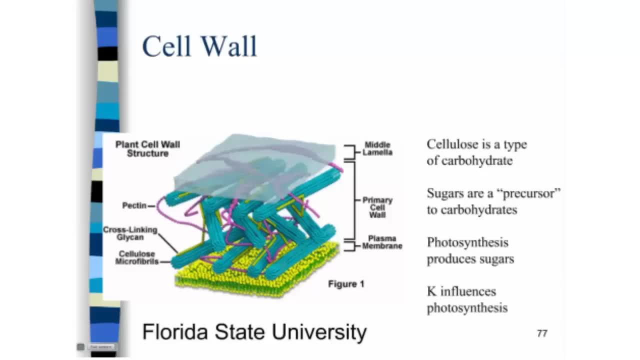 It plays a role, though, in the ability of that plant again to conduct photosynthesis. It plays a role in the ability of that plant to crank out sugars. Well, sugars wind up becoming things called carbohydrates. Those wind up becoming cell walls. 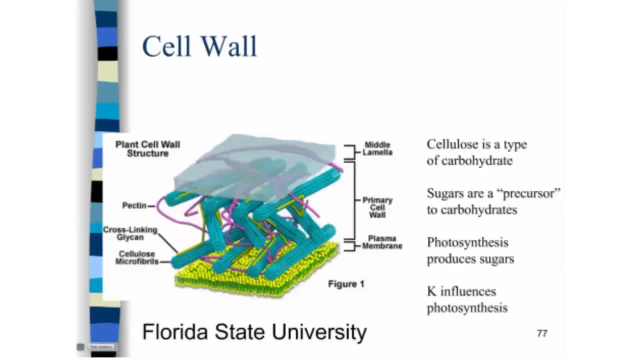 All I want you to remember is you don't have enough potash and the barrier that keeps disease out of the cell- this blue-colored barrier on slide number 77, that ends up getting compromised. You aren't able to produce the stuff you need to make this thick cell wall that keeps the bad guys out, and all these little bad guys are suddenly able to wander inside and decimate that cell. 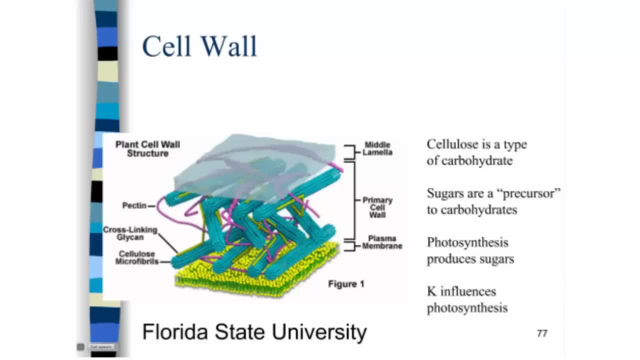 That's why potash is intimately connected to disease. We start to skip on potash, we start to see disease go up, and that's another reason why we talk about plenty of potash. It also acts like a little train carrying sugars around in the caboose, or something like that, if you want to think of it. 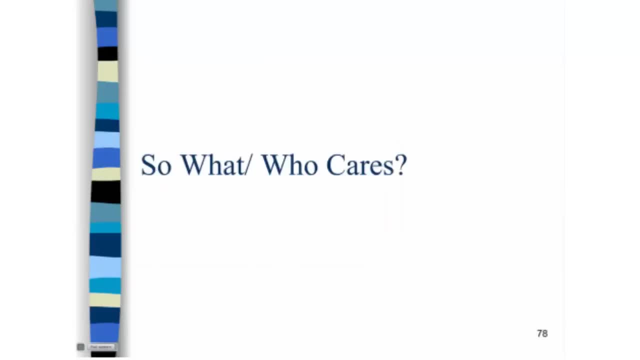 Slide number 78.. Okay, you kind of gave me Matt some so what's. Why do we care about P and K? So what, You went through all this stuff on P and K. Well, I think the so what's is the so what's. 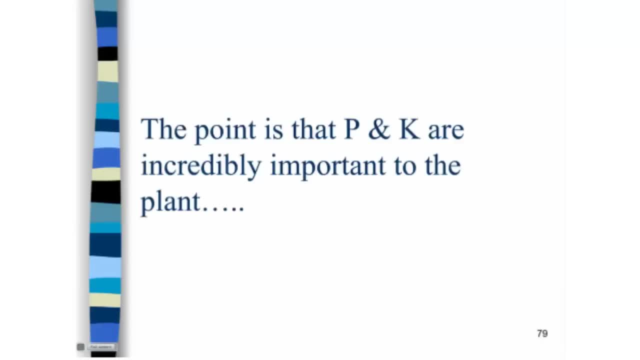 It's the so what's. I think the so what here is, like I mentioned before, phosphorus and potash and nitrogen that we mentioned earlier, but phosphorus and potash are incredibly important to the plant. Go to slide number 80.. 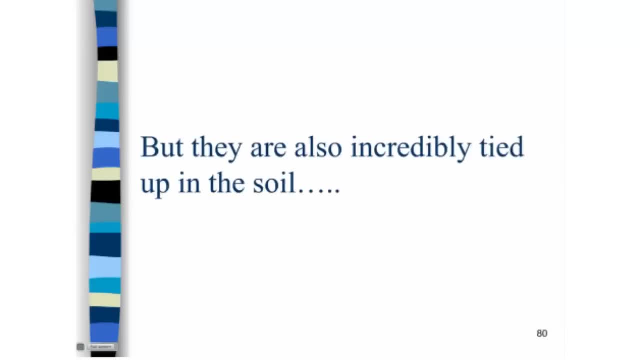 But they are also incredibly tied up in the soil. When you put on phosphorus, it has a rapid reaction with other things in the soil and it will become a coating on that soil particle. There's a lot of potash in the soil, but it's wrapped up in minerals, and also a lot of the stuff that we apply, or a lot of the potash and phosphorus that's there, gets locked up in what I call the clay sandwich. 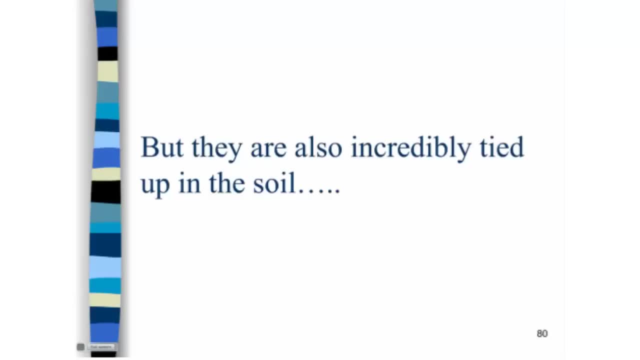 It'll get locked between layers of clay and if you think of it, it's just like a sandwich. You can't get to the meat in the center of the sandwich when the bread's there, can you? You've got to tear away at the bread to get at the meat and that's a problem for the root. 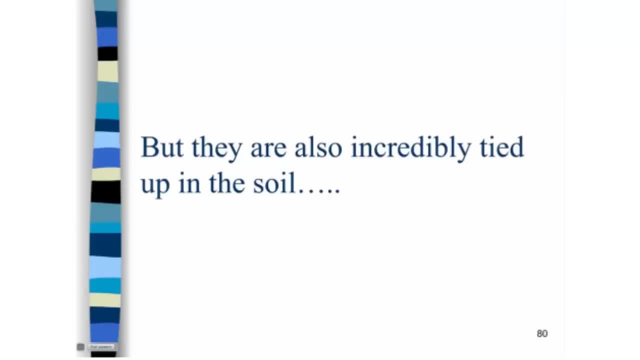 You've got to get through that clay to get to that stuff, so it's of no value in some cases. It just can't expose the root to that. It's locked it up inside this clay structure and it ends up making it not as readily available. 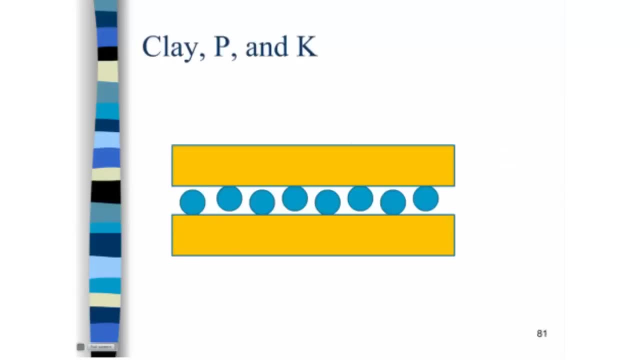 Let's look at slide number 81.. Here's a picture of my clay sandwich. That could be phosphorus or that could be potash between these layers of clay. What I want you to do, for those of you that are advancing slide by slide, I want you to proceed all the way to slide 93.. 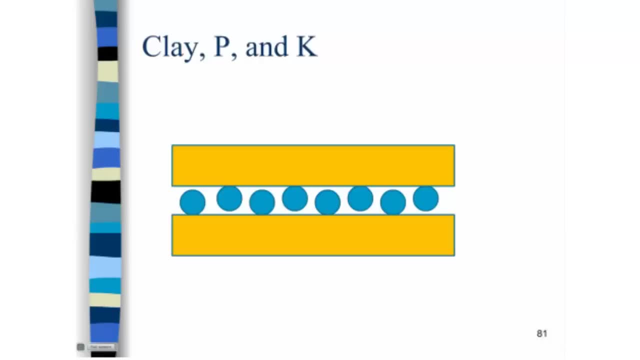 We're going to see as we do this that sometimes that clay wears away. Actually, what happens is through freezing and thawing, the clay kind of bends back. It exposes some of that phosphorus and potash so that it can be used eventually by the plant. 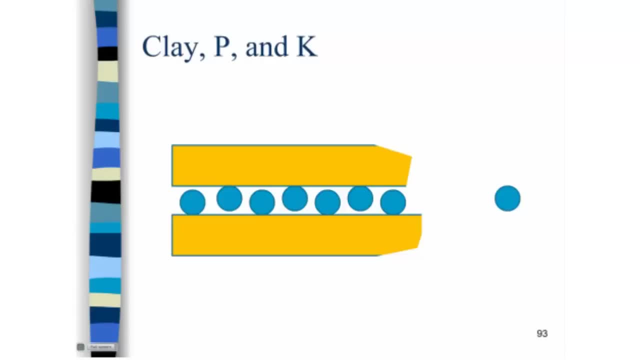 It releases it into the soil, water and all that kind of stuff where the plant can tap into it. The point here is that that's a very slow process. It takes a lot for that clay to release Phosphorus and potash. 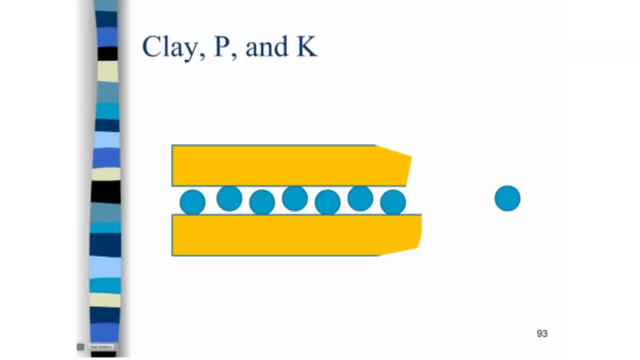 It takes a lot for minerals to degrade and release phosphorus and potash. It takes a long time for that to happen, so there's not lots and lots of this stuff floating around in the soil. Actually, one of the most prevalent nutrients in our soil is calcium, and phosphorus and potash aren't as prevalent. 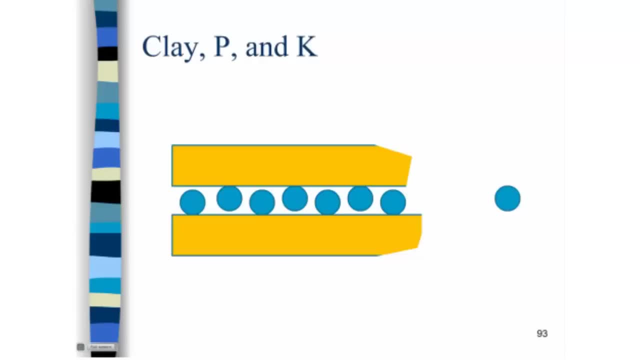 They even don't move very far. We put on P and K and they don't move but fractions of an inch from the point of location. They just don't move around in that soil very much. Because of that, we've got this interesting problem. 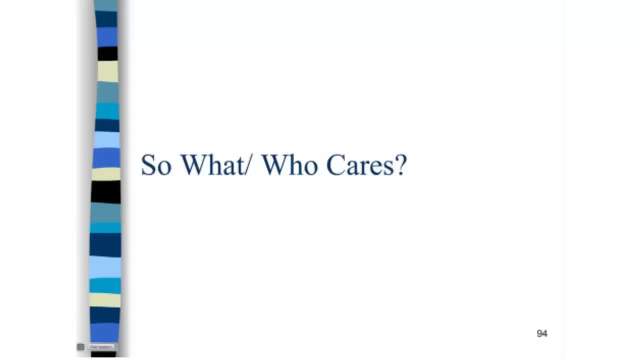 Let's look at slide number 94.. So what? Who cares? Well, the plant desperately needs potash and K, right, But I said it's also not really available and it's hard to find a little bit. So you've got these roots that desperately need this stuff, but they're having a hard time tracking it down. 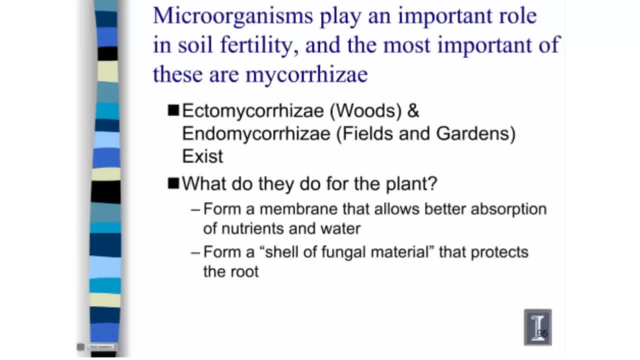 Well, that's why we like the idea- if you'll proceed to slide number 95, that's why we like the idea that the soil is actually the living and nonliving component And that's why we like the living component sometimes in that soil. 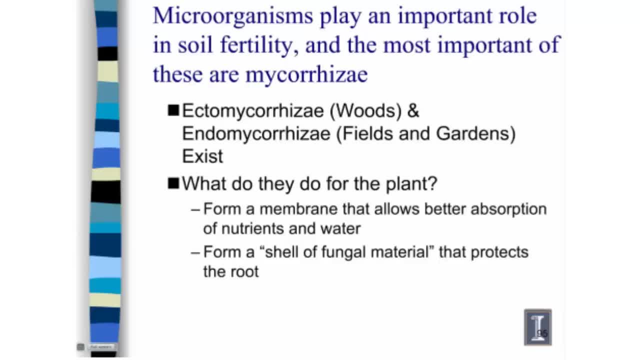 because things like mycorrhizae, little microorganisms, cover that root. They're little fungal infections of the root. basically cover that root. Yeah, they act like a protective sheath over it. keep that root safe from disease. 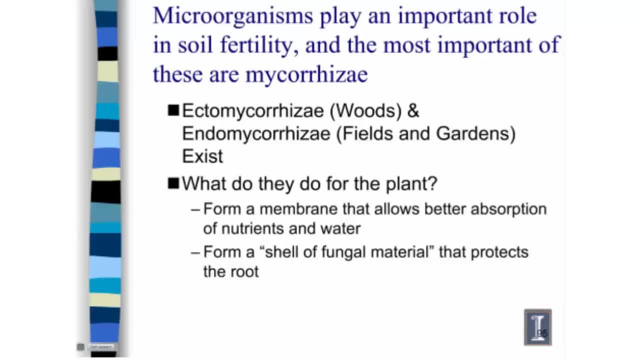 but they also branch out into the soil and they act like extensions of the root and they help that root- Yeah, Help the root- get a hold of phosphorus and potash better. So potash and phosphorus are hard to get to. 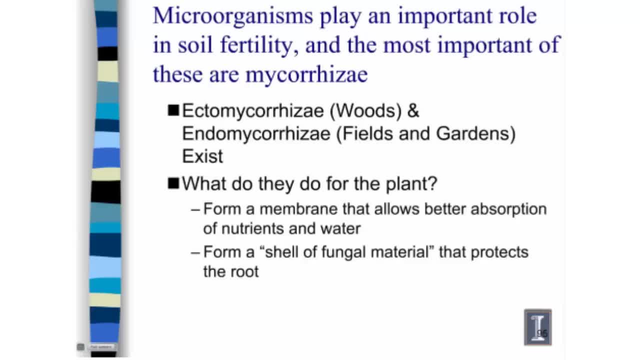 These little mycorrhizae stretch out there and act like little extensions of the root, help the root get a hold of it better. That's a good deal, And this is one of the reasons why sometimes people argue for organic amendments to the soil. 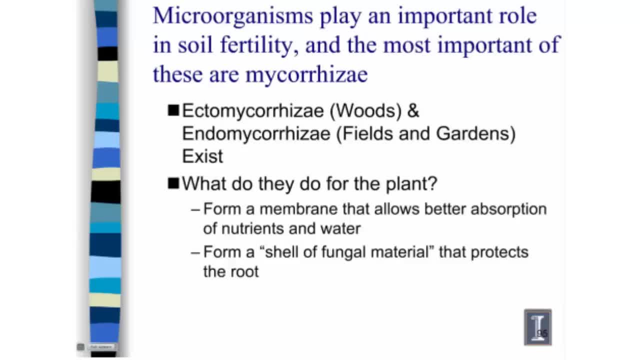 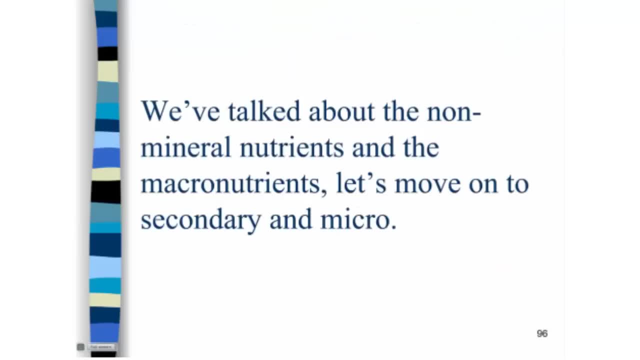 You put stuff that's dead in the soil, it tends to cultivate these microorganisms that help us out. Let's proceed to slide number 96.. So we spent a lot of time talking about the non-mineral nutrients. You'll remember that's carbon, hydrogen oxygen. 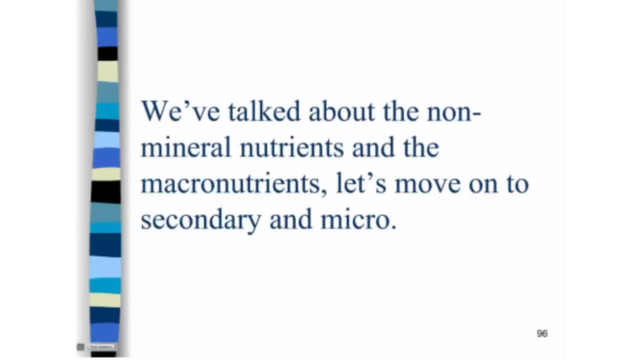 We talked about the macros. Those are the three important ones, right, N, P and K. What about the secondary nutrients? What about the micronutrients? Do we, in most cases, get worried about those? Well, let's proceed to slide number 97.. 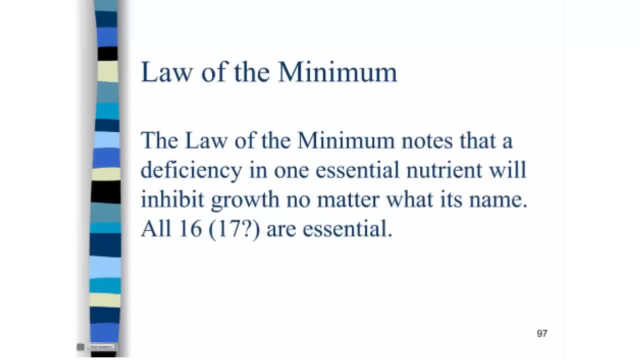 Something I want you to remember here- And we go through this when we talk in Master Gardener training- It's something called the law of the minimum. I don't want you to remember the law of the minimum. I want you to remember this. 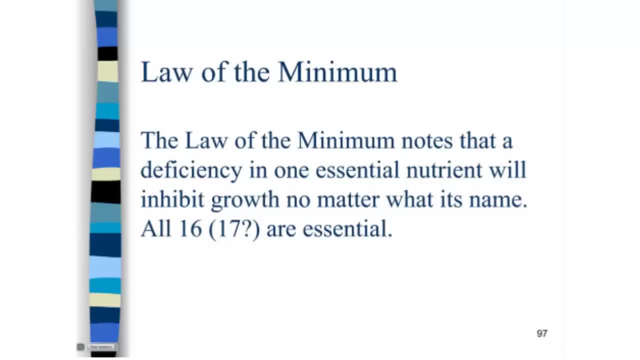 Every single one of those nutrients are important. You can hear terms like macro, secondary, micro, And you can think that that means some aren't as important as others. They're all important. If any of them are deficient, you're going to have a problem in that plant. 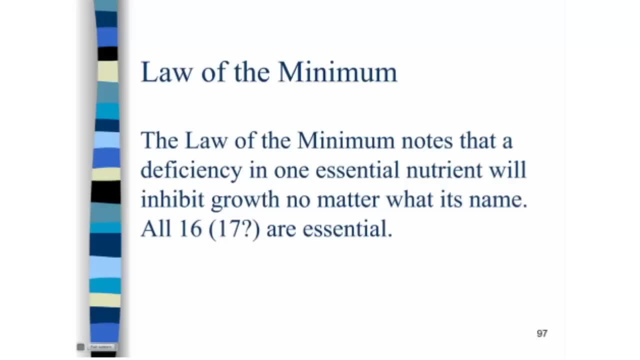 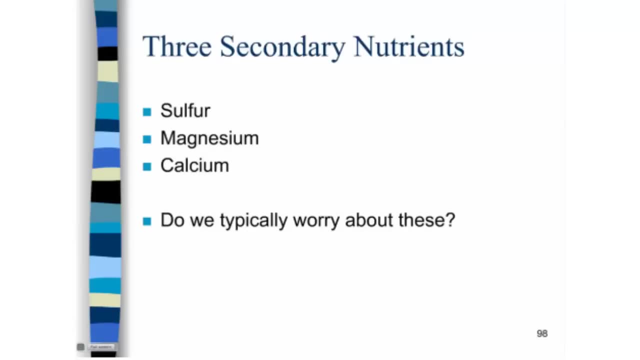 You need to have all of them. Let's proceed to slide number 98.. So what about sulfur, magnesium and calcium, our secondary nutrients? Do we typically worry about these? And I'm going to talk in generalities today, I'm not going to be talking about specific cases. 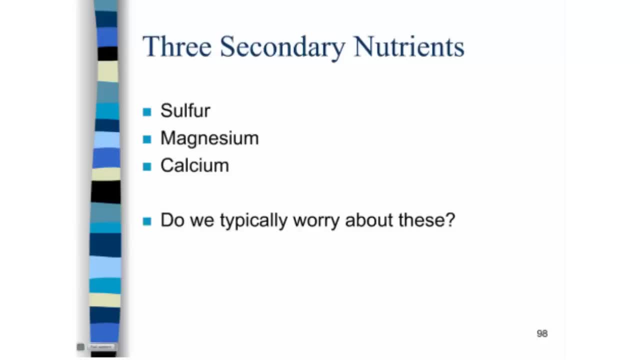 I'm talking about in most soils. do we get wound up about sulfur, magnesium and calcium? Well, remember what I said a little bit earlier. I said that calcium is probably the most prevalent nutrient in the soil. Most of our soil is derived from a limestone base. 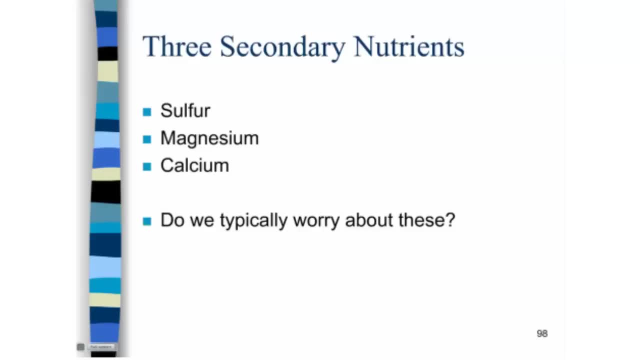 Limestone is calcium carbonate And that means there are oodles of these little calcium ions floating around, these calcium cations floating around in the soil profile. There's a lot of calcium, probably plenty of calcium in most cases, Occasionally- like for instance over here on our sandy soils- 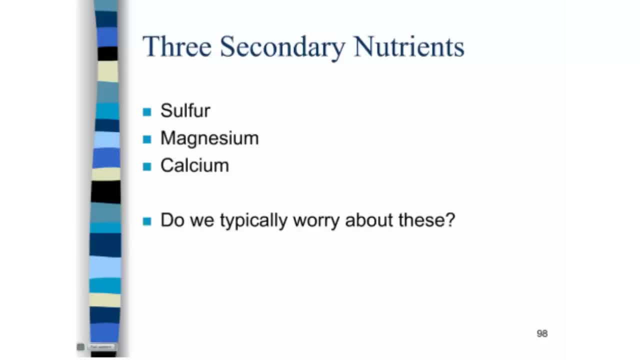 I might have an incidence of cat face on my tomato plants where the tomato puckers up. It just doesn't look quite right because it doesn't have enough calcium because of that sandy soil, And so I have to add a little bit of calcium in cases like that. 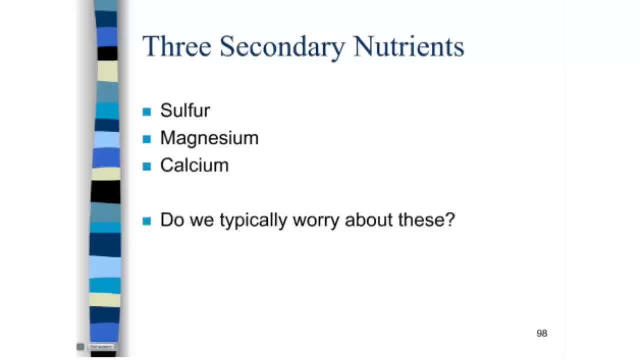 so that I get plenty of cells. Calcium is really important to cells. I get plenty of cells and I get nice-looking fruit Calcium, though in most cases we aren't worrying about applying Magnesium- Magnesium do we usually fertilize for magnesium? 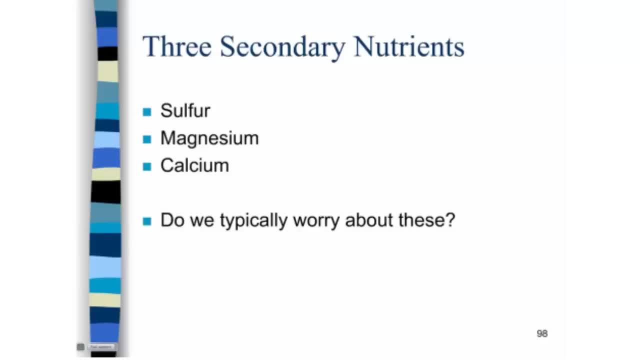 Anybody who puts on limestone basically fertilizes with magnesium. Limestone is calcium carbonate, but there's usually a contaminant in it called dolomitic limestone. That's magnesium carbonate. It also neutralizes the soil, Magnesium carbonate basically. what we mean with that, then, is that when we lime, 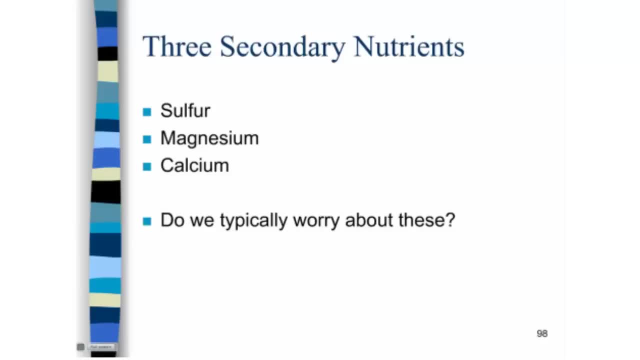 we're also putting on a little bit of magnesium. We usually don't get real, real wound up about magnesium. What about sulfur? Well, let's think about sulfur. You know, until recently, we would all get really wound up about acid rain. 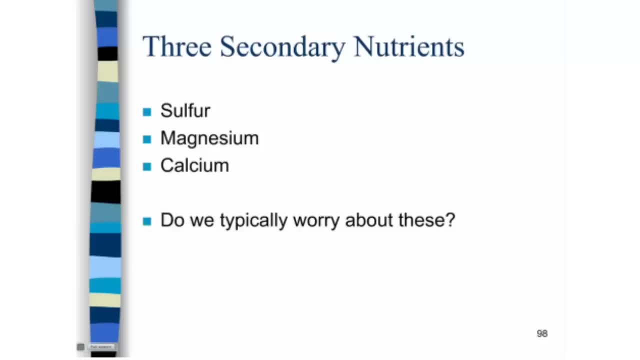 I think we still get a little bit wound up and worked up about it- rightfully so, But the environment maybe doesn't have as much of it as what it used to. There's still a fair amount that happens, though. So we have acid rain, and if you know anything about acid rain, 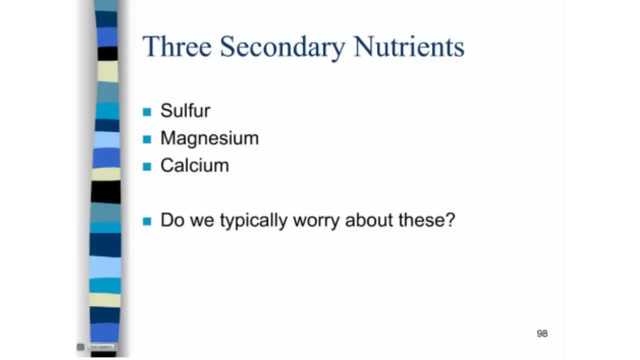 acid rain basically has sulfuric acid in it. We may apply some sulfur compounds to help out some pH, some soil acidity problems that we have. That soil needs to be acidified to get it back to neutral. We might worry about that, But in most cases as a nutrient. 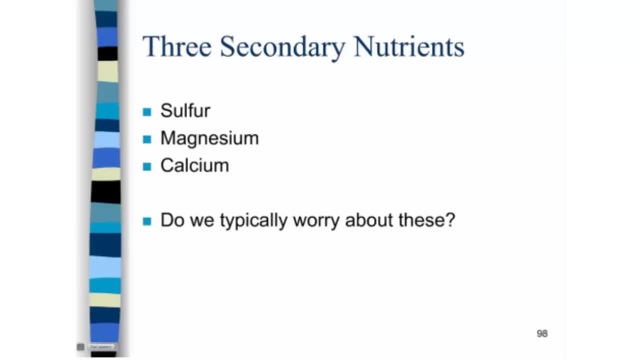 we aren't really getting real wound up about sulfur in the state of Illinois, So you can save money in most cases on the sulfur, magnesium and calcium. Let's proceed to the next slide, slide number 99.. These are the seven or eight micronutrients. 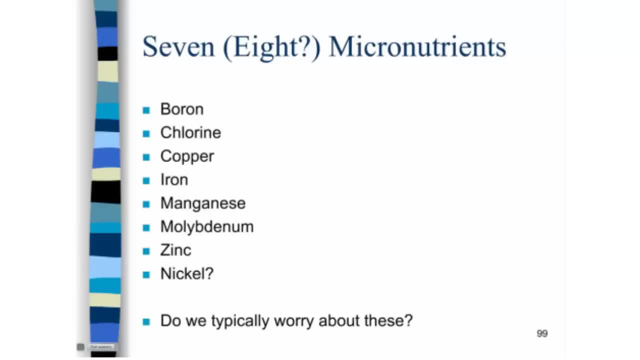 Do we typically worry about these? Well, they're all important. We just said that right. Every single one of those nutrients is important to the plant, But we usually can maintain these at adequate levels by keeping the soil's acidity at just the right level, by keeping the pH right. 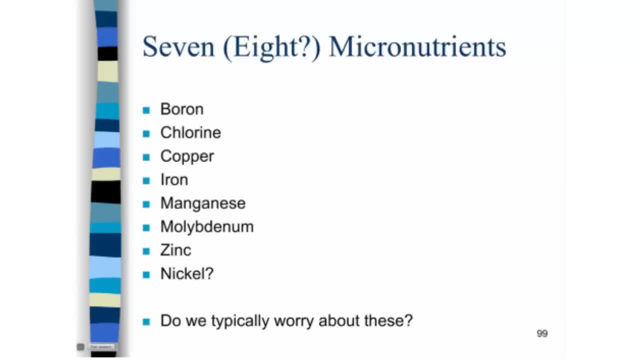 So we'll talk about pH here in just a second. We usually don't worry about a lot of micronutrient fertilizers in most cases. There are some cases Where we might do that. we usually say to keep pH right where it needs to be. 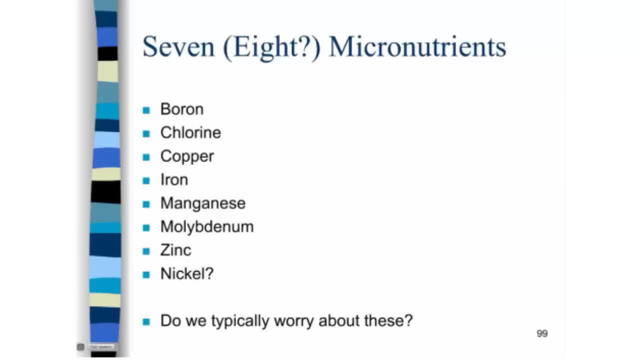 The supply of all these will be pretty reliable. The other thing is that these numbers will appear on a soil test But most people don't put a lot of credit towards those numbers because they tend to fluctuate. Those micronutrient numbers tend to move around from one sampling session to the next. 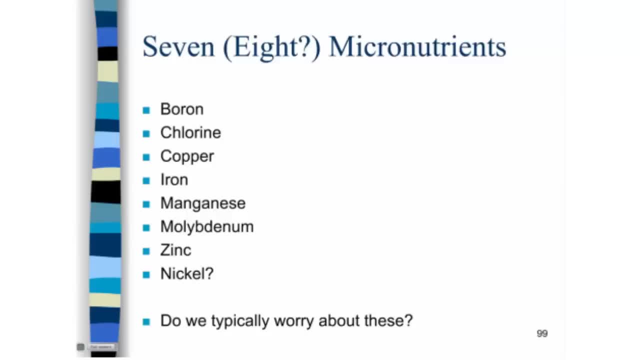 and maybe don't have the reliability that some of our other nutrients do. Let's proceed to slide number 100.. So what? Who cares? Well, this whole thing that we just went through on nutrients explains why soil tests are the way they are. 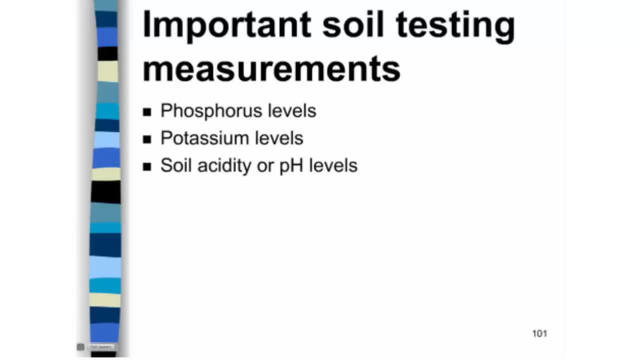 Slide number 101, important soil testing measurements. We said nitrogen's not going to stick around, So you aren't going to see that, even though it's important. What we're usually going to see on that soil testing chart is phosphorus potash. 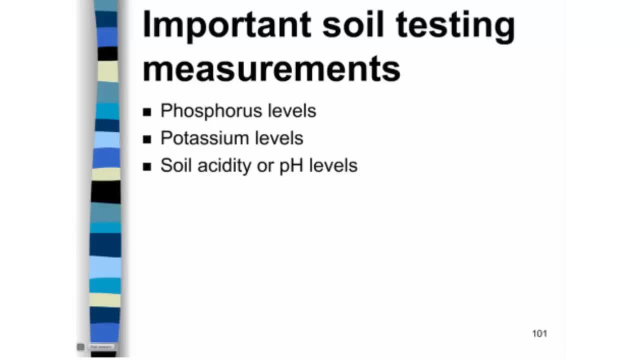 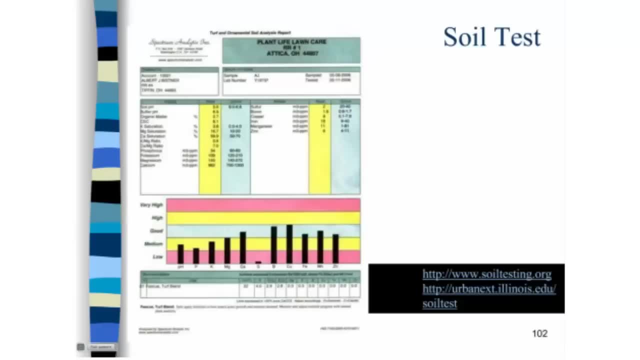 and then we're also going to look at pH. And why are we looking at pH? Because it affects the availability of all these other nutrients. Slide number 102,. this is actually off of the slide presentation again that we did for the Specialty Growers Conference. 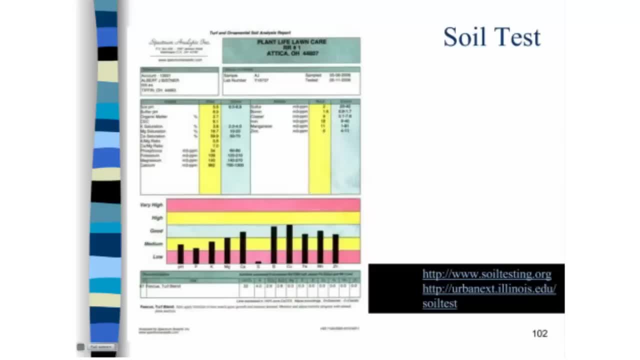 And this is just a picture of a soil test. You want to work with a soil testing company. It's the best way to figure out what's really happening with your soil nutrient-wise, with your soil pH-wise. It's all private in the state of Illinois. 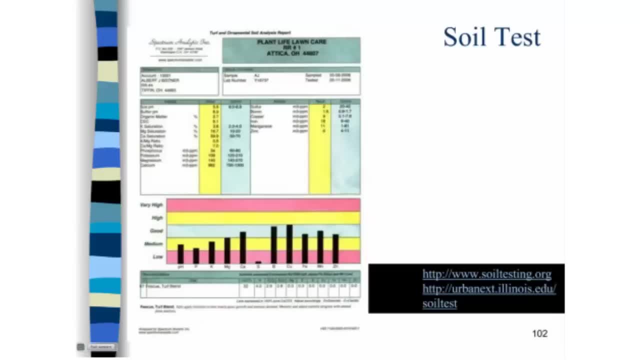 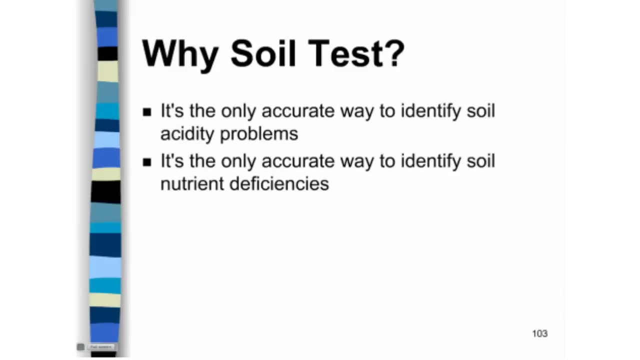 So you can go to some of these websites that are listed to reference that. One thing I would mention: when it comes to soil testing, it's very important that when you collect those samples you try to get them into the soil testing company very quickly. 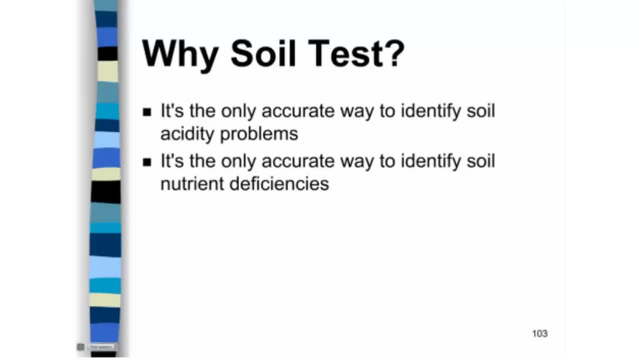 You don't want them to sit out there very long And it's important that you make sure that soil testing company can deliver it to the soil testing company directly or through an intermediary, like some of the fertilizer dealerships will send it off for you. 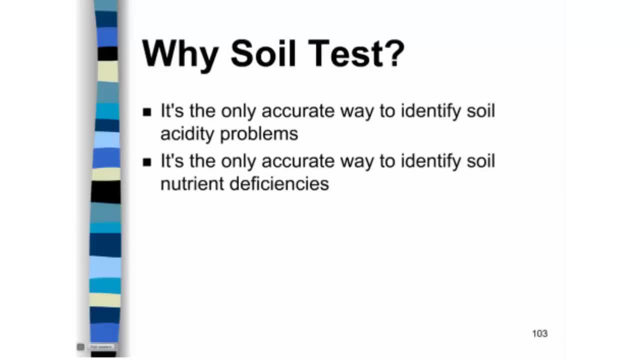 Make sure that they understand what the purpose is for that soil test. Is it for garden? You want to spell that out. Is it for vegetable production? You want to spell that out? You want to do that because otherwise you get results back that tell you how to grow corn and beans. 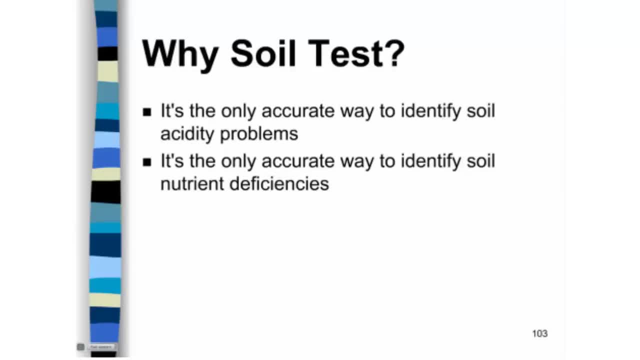 on that piece of ground. It's probably not what most of this audience is looking for. So slide 103,. like I said earlier, the reason we get worked up about soil testing is it's the only accurate way to tell us what's going on. 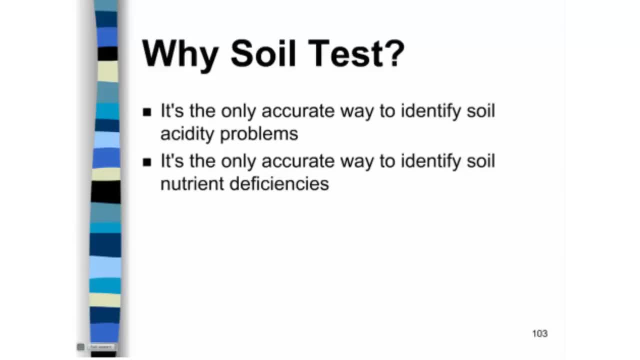 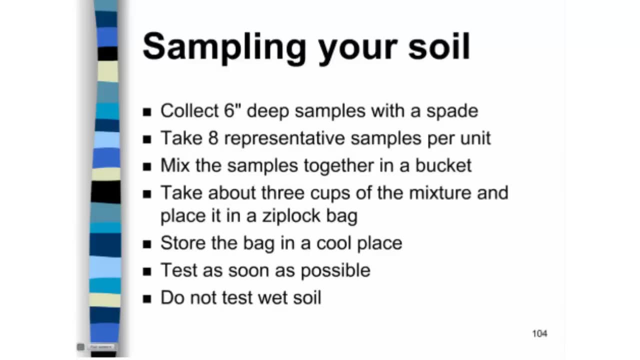 If we start doing stuff blindly in the soil we're going to create some real big problems. Slide 104.. So how do you sample your soil? Basically, we want to look at the root zone. Why do we want to look at that six to seven inch layer? 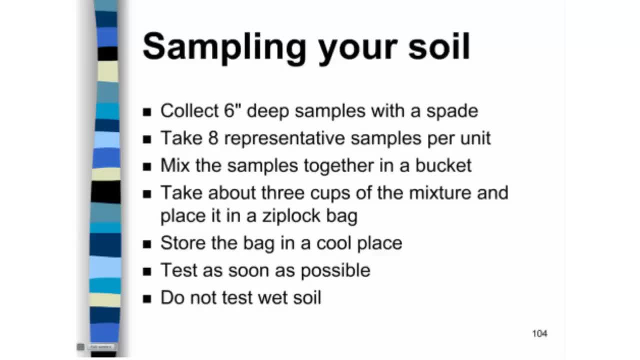 Because that's where the bulk of the roots are. That's where they're going to be getting their nutrient supply. So we want to find out what it looks like there. So six inch deep samples in the majority of cases, maybe eight representative layers. 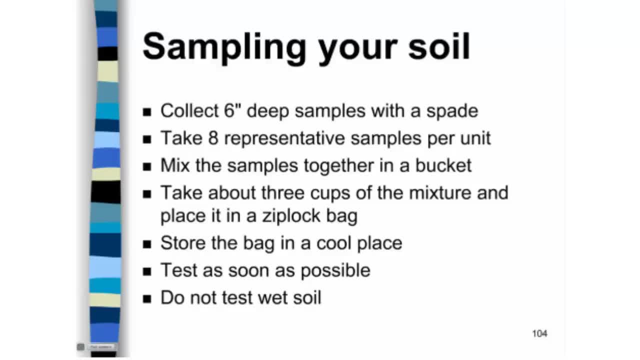 eight representative samples per unit. What I mean by that is you want to take those samples in a way that best represents that unit of area. If there's a little leg of the yard or field that sticks off in a direction, you want to pull it from that leg. 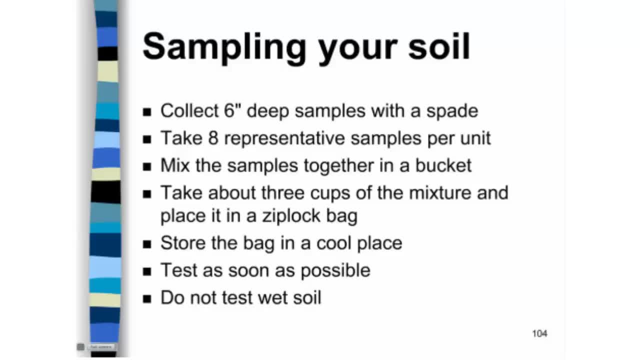 You want units separated individually. So you got a garden. you want that separated maybe from your flower garden or maybe front yard, backyard or your vegetable production for this commodity versus your vegetable production for that commodity. Mix those in a bucket together. You're taking about three cups of that. 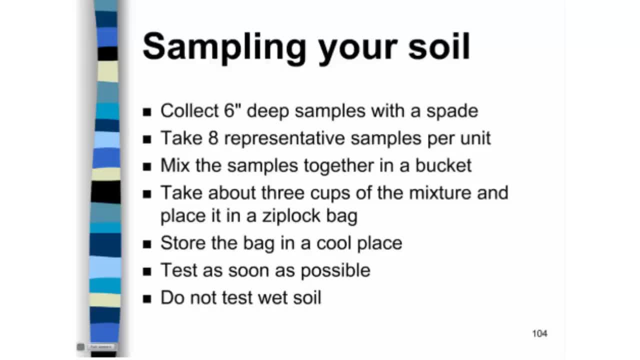 and, like I said, you're making sure you get that in to the soil testing company quickly before microorganisms can start chewing around on stuff in there and change some of those numbers. Let's look at slide 105.. Like I said earlier, you want to choose a company. 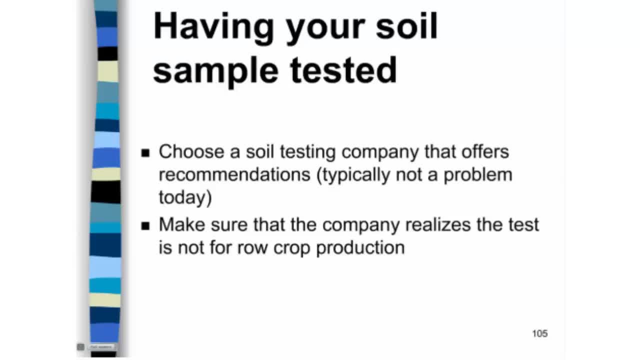 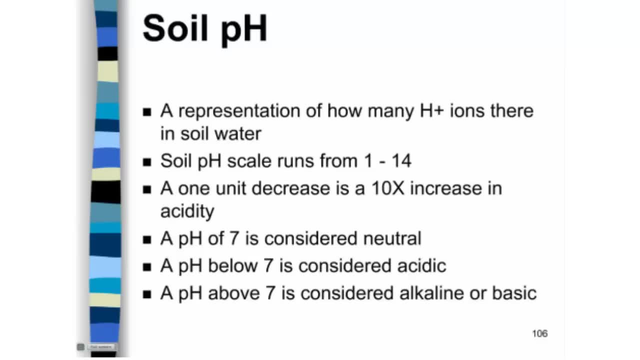 that'll give you recommendations for the crops you're looking at. Most of them will give you recommendations. You just want to reiterate the purpose: Slide 106,. we haven't talked about pH yet and we probably need to talk about pH. 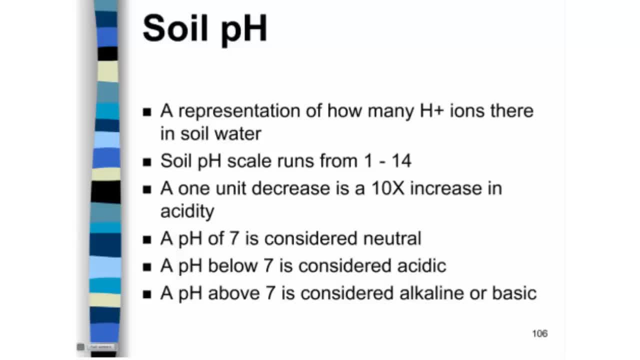 What makes the soil acid, or little hydrogen ions floating around in the soil, in the soil water in particular. We get a lot of those and that can be a problem. The point you need to remember about the pH scale today is that it runs from 1 to 14.. 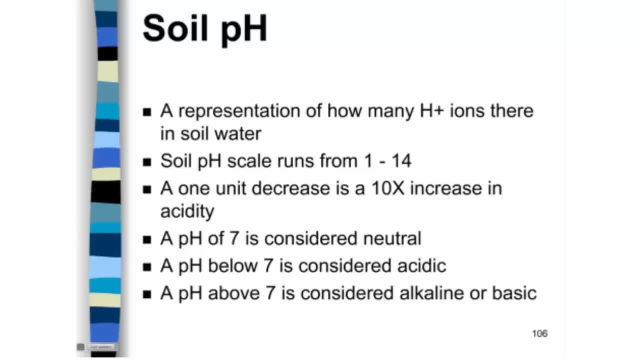 As you go down it's more acid, As you go up it's more alkaline, And either extreme is bad. We said we want neutral or around neutral. Around 6.3 to 7 is what we really want to shoot for. 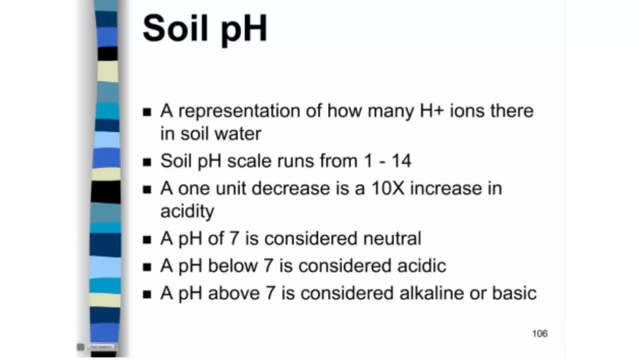 Slide 107,. so what, who cares? Slide 108, it's just reiterating that point I just made. We want a soil pH that's around 6.3 to 7 because, as I mentioned earlier- slide 109, things like micronutrients are greatly influenced. 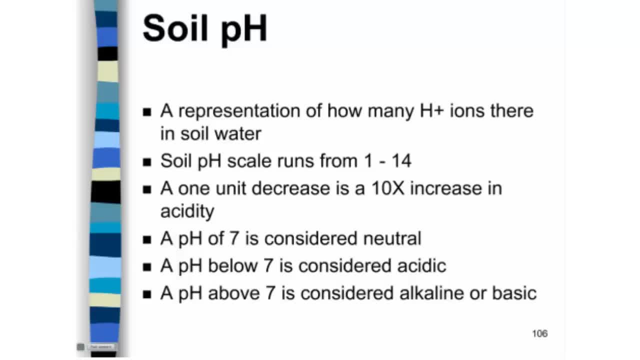 by acidity of the soil. Slide 110 just demonstrates that with a graph. This is a pretty standard graph that we've used at the university for quite a while and Master Gardener training and other places. The wider that band is, the more available that nutrient is. 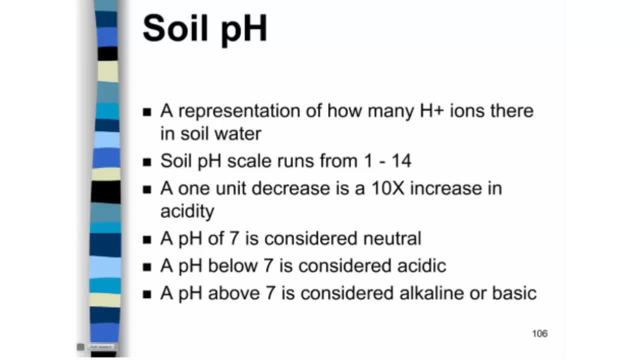 The more it thins up, the less available it is, And what you should gather from that is that sweet or sour soils, either extreme acid or alkaline, is a problem. We want 6.3 to 7 in most cases because that helps us get. 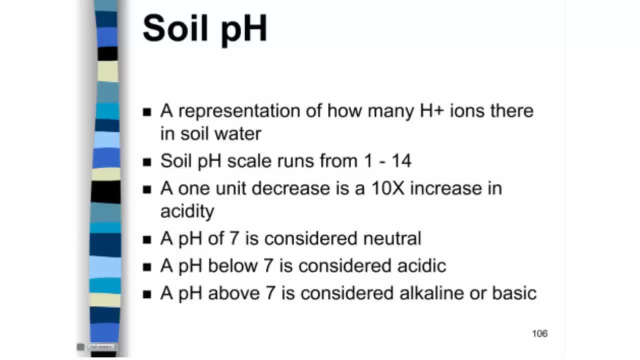 the broadest swath of availability for most of these nutrients. So pH, like I said earlier, is basically a representation of how many of these little hydrogens float around in water. I don't think that's incredibly important for you to remember, but it does help to explain something that is important for you to remember. 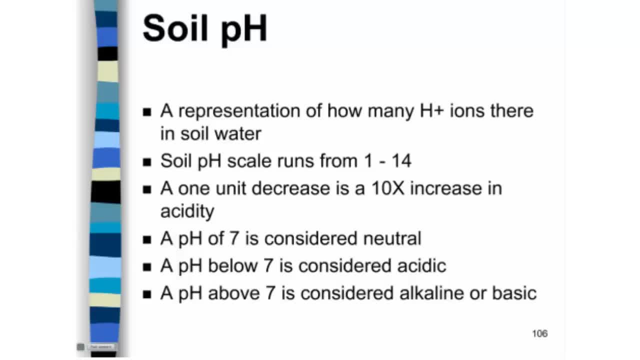 Can I go into the store? just forget the soil testing company. I'm going to go into the store and get one of those little pH test kits. I'll figure out how acid or alkaline my soil is, and then I want to pay the soil testing company to do that. 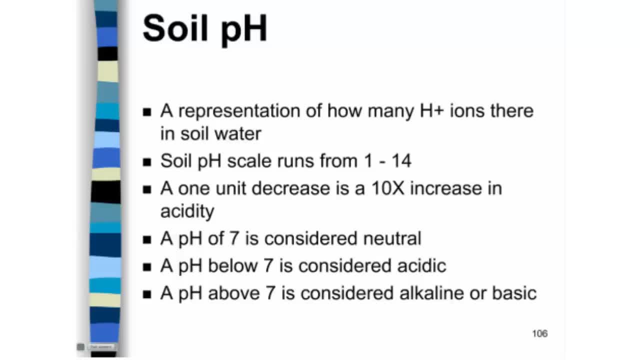 I'll solve this problem myself. Well, it will tell you how acid or alkaline that soil is, but you can already think about one problem right. One problem is then: what? What do I need to do after that? That gets to be kind of complicated. 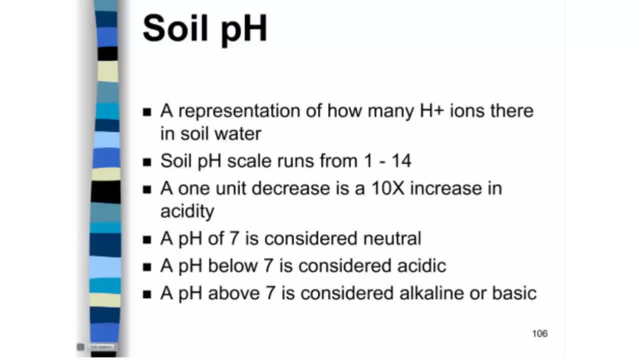 but the other thing is. the other thing you need to know is that reading the pH with that little meter isn't enough. You need another bit of information. That's that cation exchange capacity we talked about earlier. You need those two numbers together to tell you how much lime. 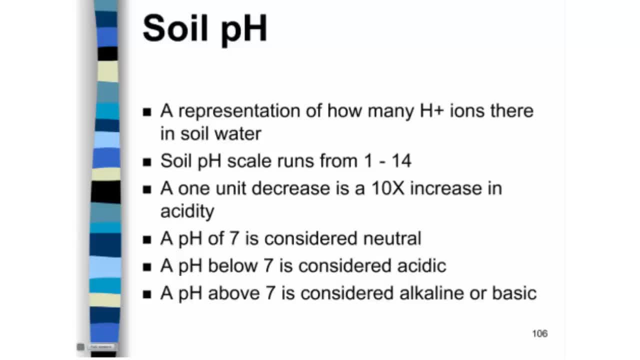 for instance, you need to apply- I'm not going to explain why this is. It's too complicated really for today- because you have little hydrogens in the soil that bounce off and take other hydrogens in the water to their place. 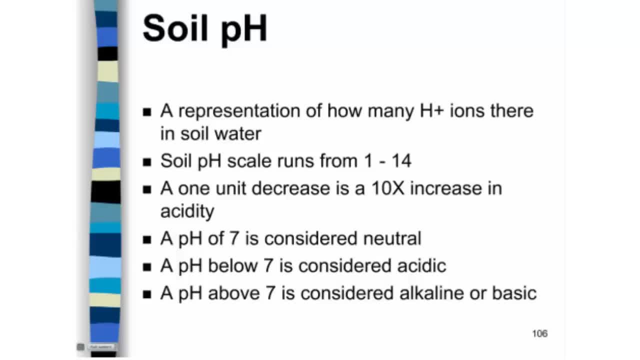 and all that kind of stuff. that can really get us confused. But what I want you to know is this: A dark-colored soil and a light-colored soil can both be at the same pH. You can stick that pH meter in both and they will both read the same pH. 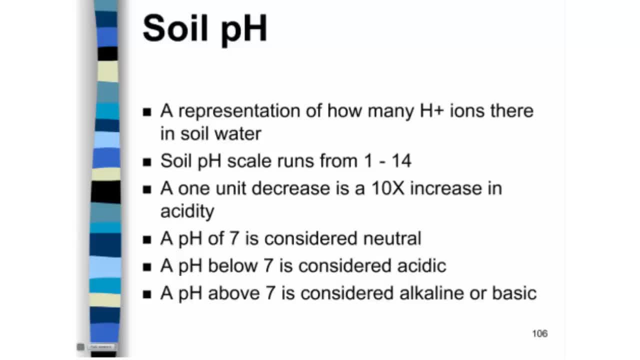 And maybe you need to put on some lime and get them back to neutral. It will take more lime on the dark soil than it does the light-colored soil. You'll be able to get that light-colored soil to neutral rather quickly. The dark-colored soil will take a lot more lime to get it there. 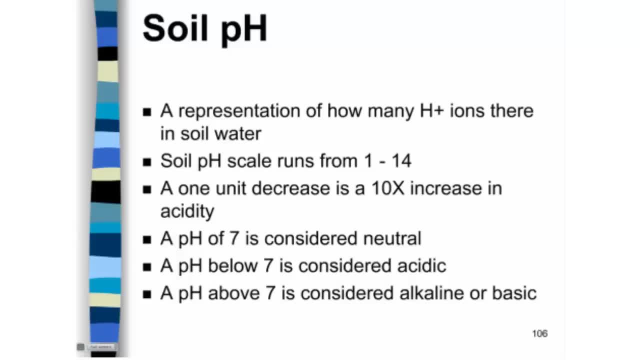 And that's because CEC- how many little negative spots are in that soil- comes into play here. Long story short, you can't just buy the meter at the store. You've got to have that pH reading and CEC. That's why we hire the soil testing company. 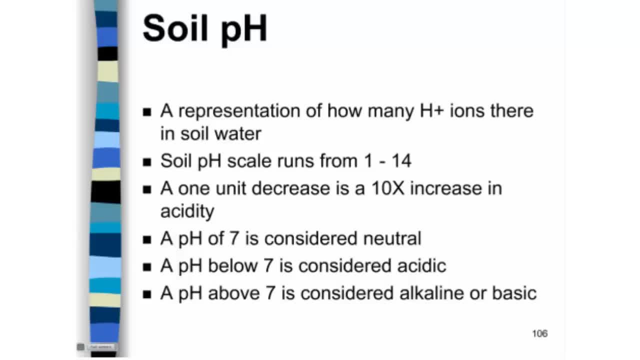 They'll figure out what CEC is. this is really why they find out CEC, to begin with. They'll figure out what it is, figure out what pH is, and then they've got little graphs that they can use to tell us how much limestone. 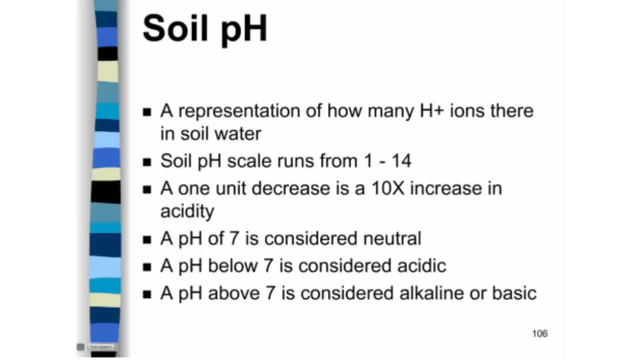 or, if we need to acidify it, how much sulfur we need to apply. Well, I'm going to take a second, and I know you probably aren't real, real crazy about knowing this, but I'm going to tell you why limestone works. 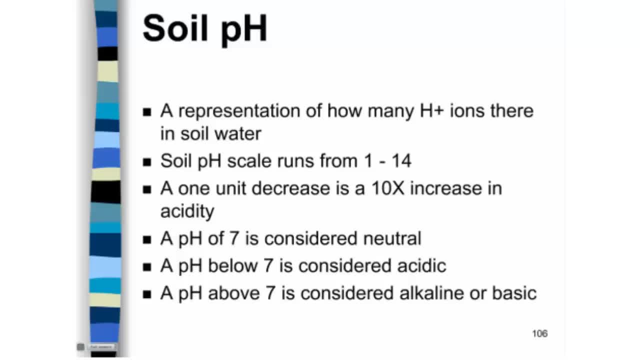 You remember, on our earlier slides we talked about hydrogen is what causes acidity. Here we have these little hydrogens stuck on a soil particle and they're causing the soil to be acid. We want to get rid of that, right, So we put limestone on that's calcium carbonate. 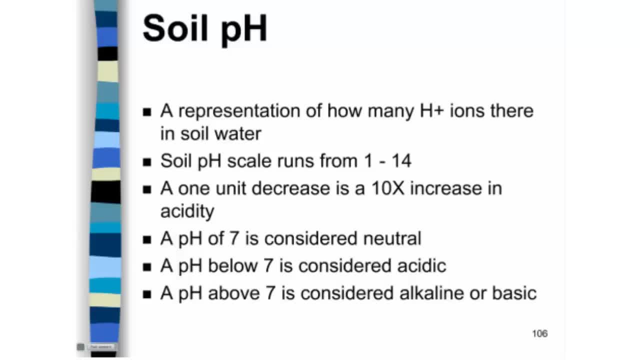 and the calcium carbonate basically bumps the hydrogens off there, and then those little hydrogens combine with carbonate and they're eventually transformed into water and carbon dioxide. We eliminate acidity by transforming that acidity, so to speak, into water. Now, why did I mention all this? 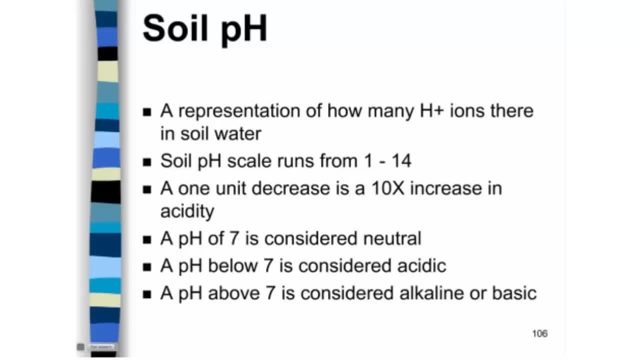 You cannot have followed anything, but what you should be able to spot is that carbonate is incredibly important to our ability to lime Carbonate's. what does the deal? It wasn't really calcium that did anything. It just moved the hydrogens around, right. 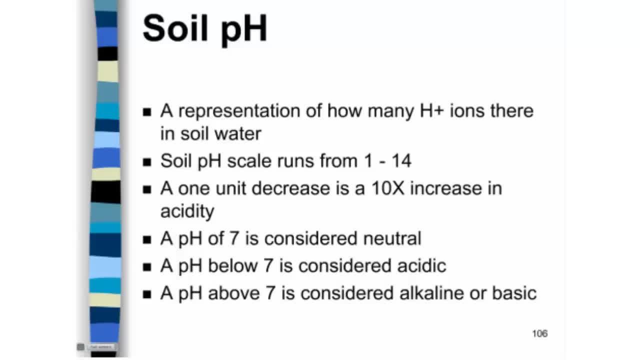 It's the carbonate that limes the soil, that eliminates that acidity. Well, this answers a question: What about gypsum? Do you apply gypsum as a liming material? Gypsum, if you're familiar with it, is basically drywall, basically chalk. 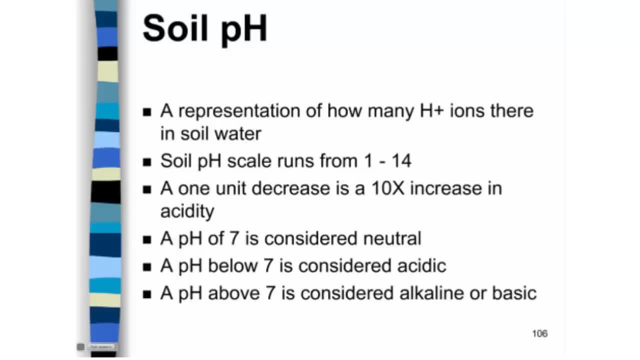 and it's calcium sulfate. Well, the calcium part of that sounds good, doesn't it? But it's missing that critical carbonate component. So we talk about it in the state of Illinois. to be honest, in most cases, gypsum's not going to do anything for you. 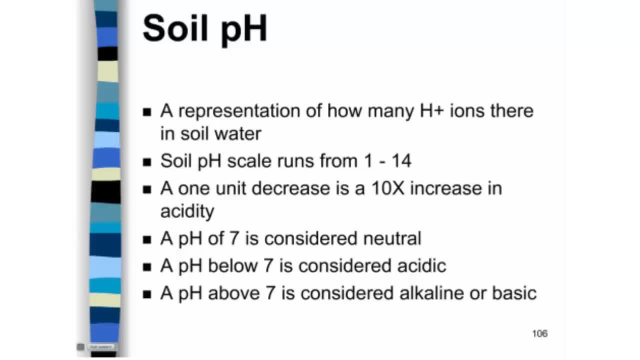 especially not on the acidity side. It's not going to act as a liming agent. Now there might be cases where the calcium is beneficial to raising some kind of fleshy fruit or something like that. In most cases, though, I said, calcium's readily available. 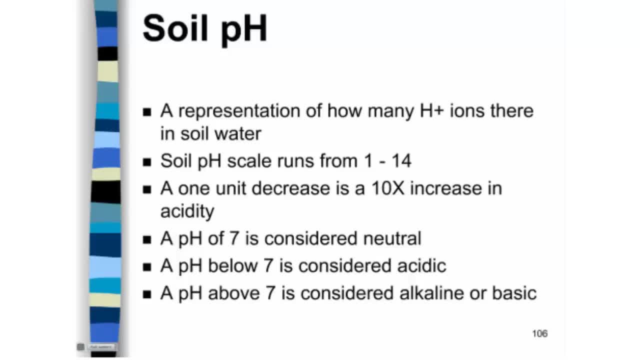 There's plenty of it in most soils. We said. sulfur kind of gets deposited by acid rain. It becomes hard in the majority of cases to really point towards gypsum being the need. There might be some special cases where that is so, But the take-home message from this would be: 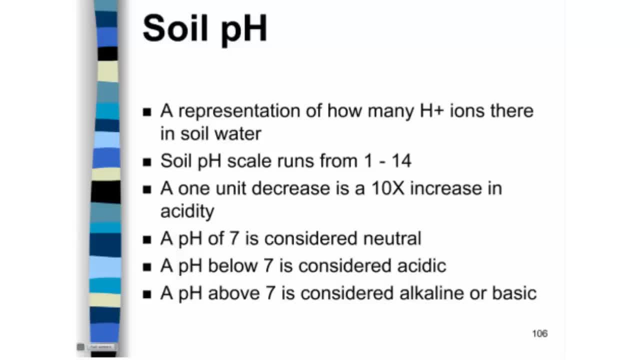 for you. it doesn't have carbonate, It's not going to lime. The other two nutrients are really supplied In most cases. you can probably save yourself some money. Let's flip to the next slide, slide 118.. I mentioned just a little bit ago 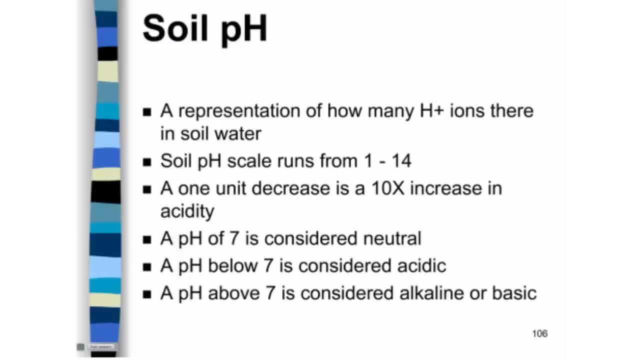 that N, P and K are the macronutrients. They're outside of carbon hydrogen and oxygen. The highest in the plant by weight, maybe 4% or 5%. for nitrogen and potash maybe like a half a percent, 0.4%. 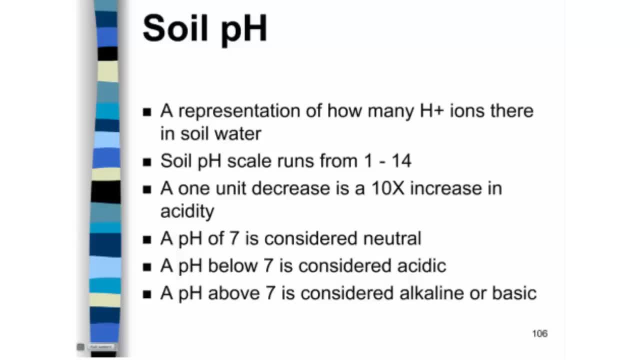 for fiber And they're represented on that fertilizer bag, as I mentioned earlier, by three numbers: that 10, 20, 10.. 10 stands for 10% nitrogen, 20 stands for 20% phosphorus. We'll say today it stands for phosphorus. 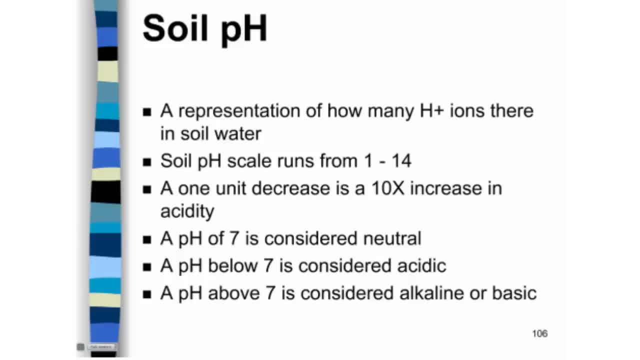 It actually stands for something a little bit different, but phosphorus is a good way to keep track of that. And then 10% potash. We'll say it that way for today. More or less. what we're saying is 10% of the weight of that bag. 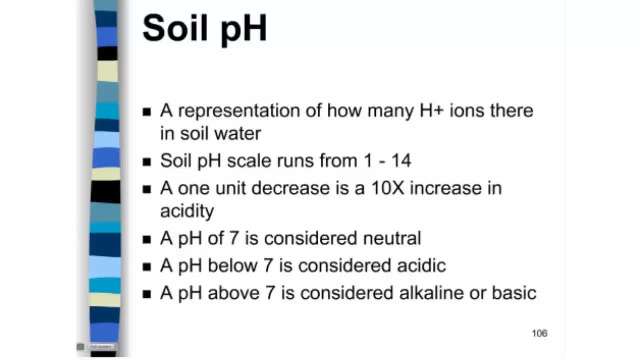 is actually nitrogen. So out of every 10 pounds of that fertilizer you have one pound of nitrogen that's actually in there. Out of every 100 pounds of that fertilizer, 20 pounds of that is actually phosphorus. So it lets you know kind of how you need to tweak things. 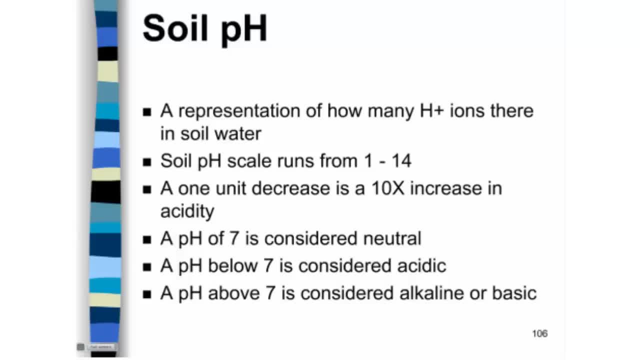 to apply the right amount of N, P or K. This is a little bit more agricultural row crop, agricultural in nature, but it does kind of fit in with the production of fruits and vegetables. You know, when we talk about a fertilizer recommendation. 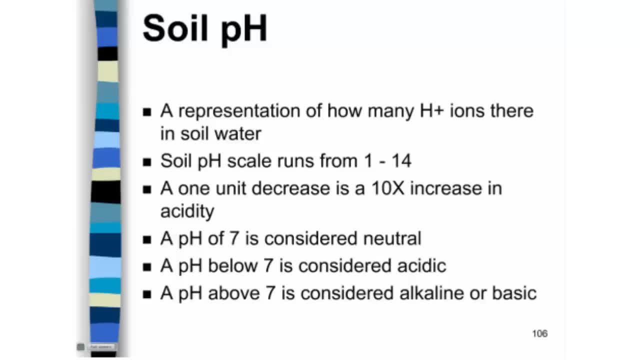 for an area even that we're growing vegetables in. we kind of want to elevate the soil to a critical level that we think it needs to be at for P and K, for phosphorus and potash, And then we call that buildup. But then the other thing is, we'd like to put on. 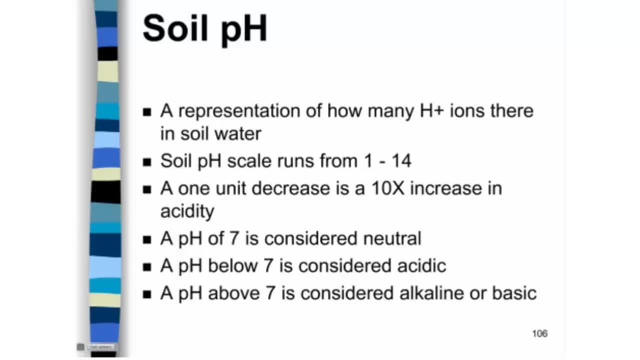 what we take off. right, We want to keep all things even. We want to replace what we harvest off in the form of fruit or yield and want to kind of keep that even So, one of the purposes, not the only purpose. 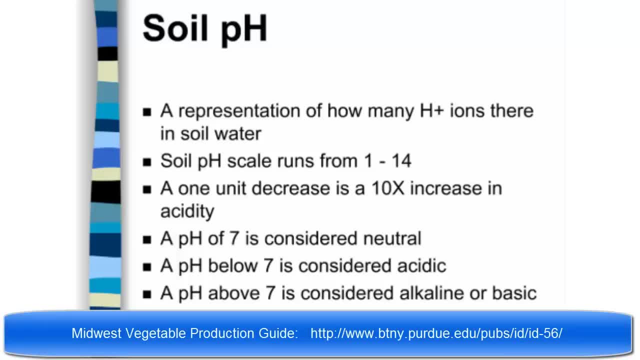 one of the purposes. if you look in a Midwest vegetable production guide, some of those numbers that talk about you need to put on this much phosphorus or this much potash when you're raising that crop. one of those is: yes, get that plant up and moving. 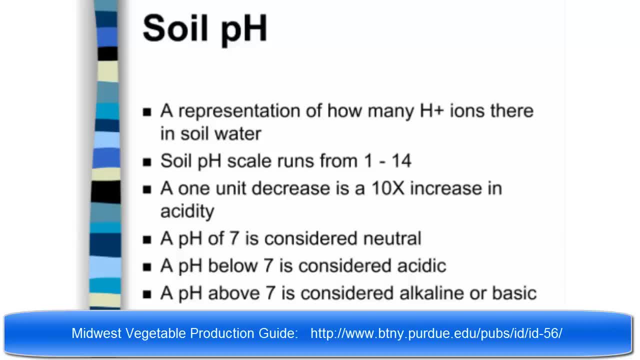 do some other things for that plant, but it's also to kind of replace some of the stuff we're going to harvest off, to keep that soil even right where it is, to make sure we don't leach it down, dilute down. 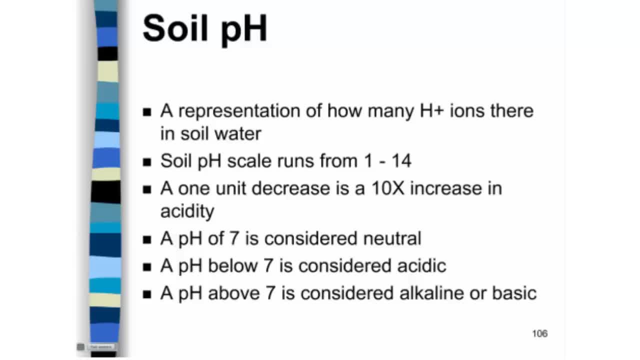 dilute down the availability or the amount, I should say, of that nutrient. So let's get a little bit into this organic versus inorganic question. There are organic amendments. These are a couple organic fertilizer rules of thumb. One thing is that leaf material 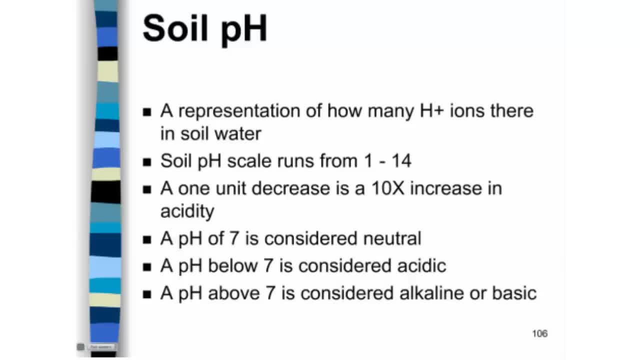 tends to be pretty acidic in nature. So if you have a soil that's very alkaline, very sweet, and you need to get it back down to neutral, leaf material can help you do that. Now, one of the problems is that you and I both know it's going to take some time. 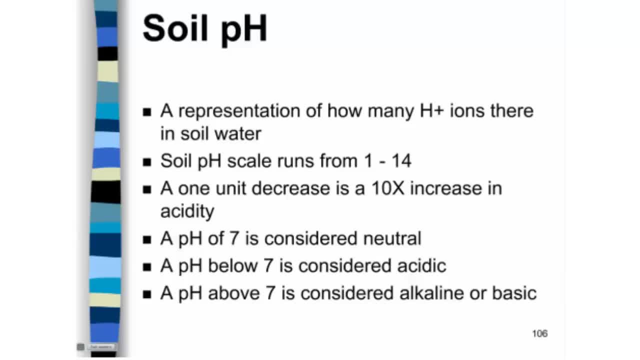 for that leaf material to degrade, to make that happen, and that gets to be one of the issues sometimes people have with organic. but it can do it. It is a source of acidifying. It's an acidifying agent, I should say. 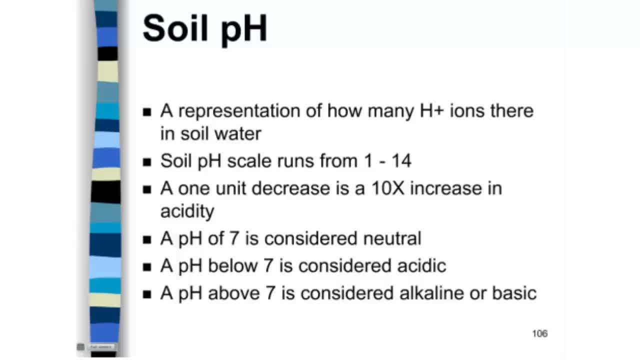 Blood meal, dried blood and manures tend to be a great source of nitrogen. That makes sense. There's lots of protein in that right And I said protein Nitrogen helps make up that protein, So those materials tend to supply a lot of nitrogen. 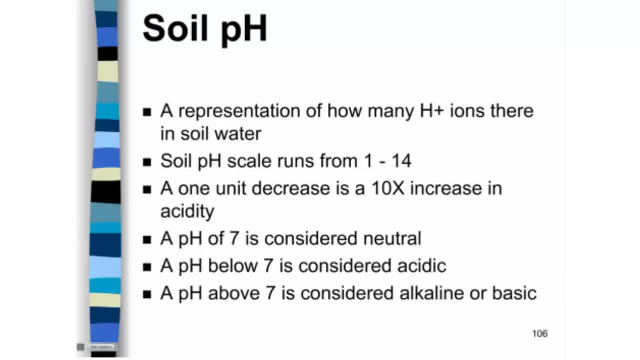 Again, there'll be variability in the representation of that. We might not be able to point at that product and say it's exactly 10% nitrogen. It may be a range that we talk about Bone meal, steamed bone or charred bone. 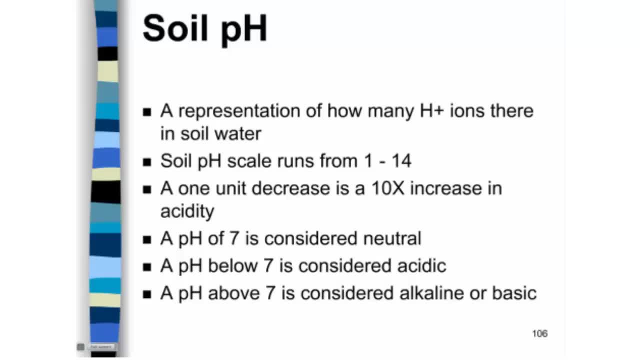 tend to be a great source of phosphorus. Now we think of that being a great source of calcium and I guess there's probably plenty of calcium in there, but that's not why we're really applying it right. We said there's a lot of calcium in most of our soils. 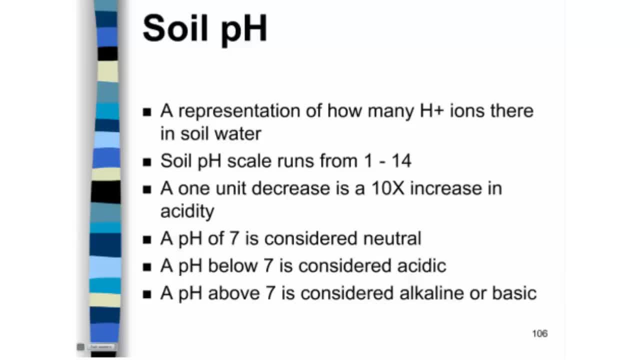 so amending calcium really isn't our goal. It's more phosphorus that we're shooting for, And things like bone meal can be a source of that Potash. you know why do we call it potash? One of the reasons wood ashes was kind of the way. 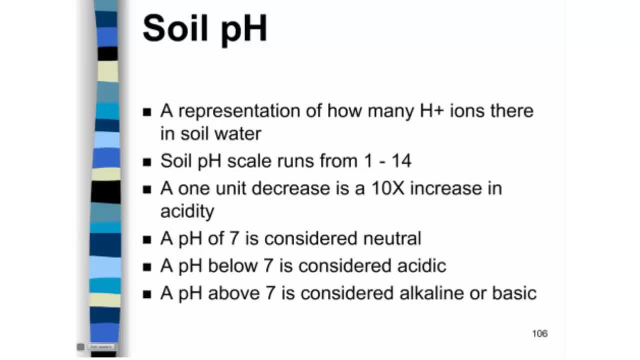 we used to talk about supplying potash. Wood ash is a great source of potassium, And then something else to keep in mind is that potash can also be supplied by manure as well. You lay out manures for too long. a lot of the goody gets leached out of them, though. 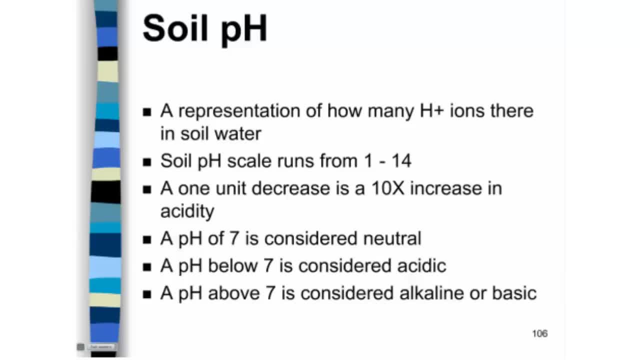 and you need to be careful of that. One thing we also should probably mention, since we're talking a little bit about organic fertilizers or even inorganic fertilizers. with some of these products, we may want to put them on a few weeks ahead of time. 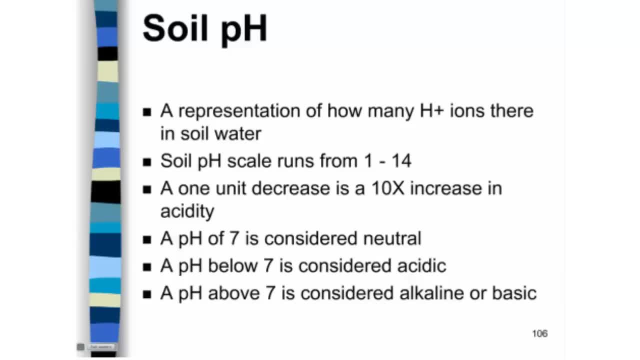 or several weeks ahead of time, just to make sure that we, if it's the case of an inorganic fertilizer, we're getting that in there to where it's actually going to be of use: to the plant or organic, in particular, The longer end of the spectrum. 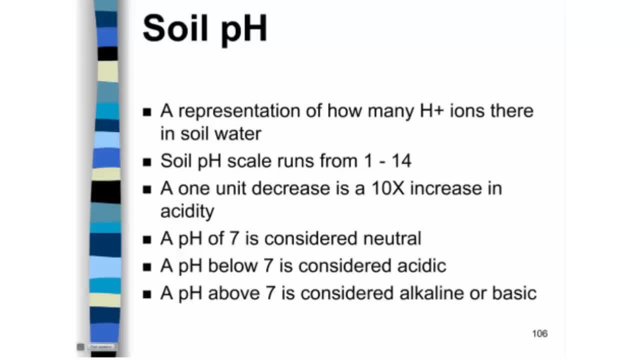 we want to give it a chance to break down and release those nutrients that are stored within The organic material is basically slow-release fertilizer. As stuff decomposes, it's going to slowly release these nutrients that the plant needs. We actually today at our session here, had something on tillage radish. 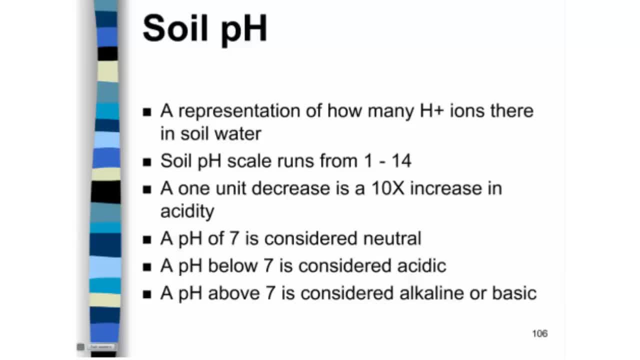 and they were talking about how the tillage radish is a radish you can throw out in the field to help out with some other issues. It can absorb some of those nutrients, act like a storehouse and then slowly release those as it decays. 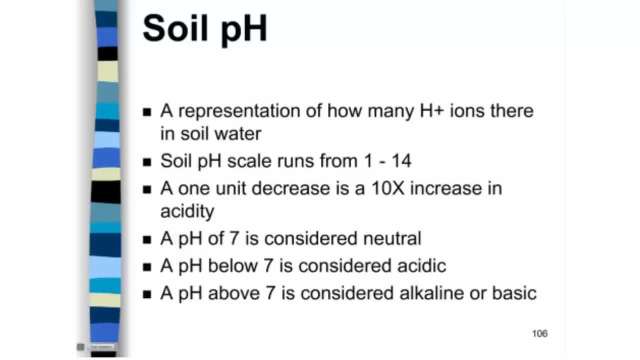 Organic matter acts like a slow-release fertilizer. As it decays, it releases a lot of that nutrient. Why do we care? inorganic versus inorganic, What's the big point here? Well, I don't know that. my role today is to preach inorganic versus organic. 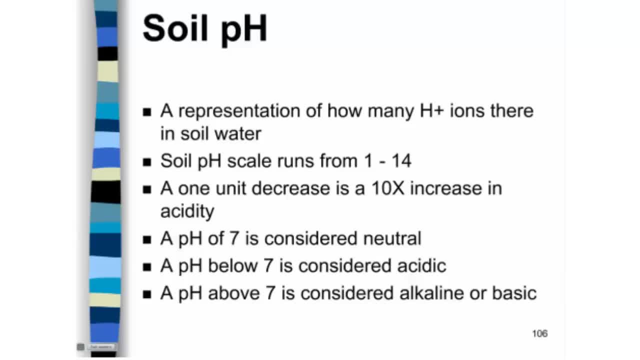 I think my role, as it usually is in Extension, is to show you the pluses and minuses and you can make a decision from there. Let's talk about some advantages and disadvantages of organic. One thing is that organic definitely gives some improvement to soil tilth. 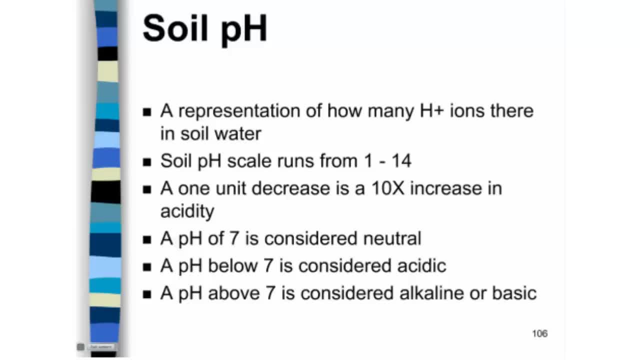 It gives some springiness, some recovery ability to that soil. It can help us resist the trend towards a lack of structure, for instance towards compaction. It can help us ward that off. It can give us some springiness back to the soil. 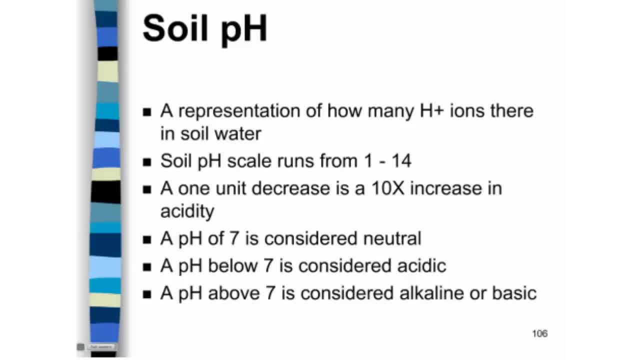 Organic we mentioned earlier also fosters soil microorganism growth. Things like mycorrhizae can be promoted to a certain extent by applying organic amendments. Organic can be very expensive, right? We aren't just producing the good stuff. 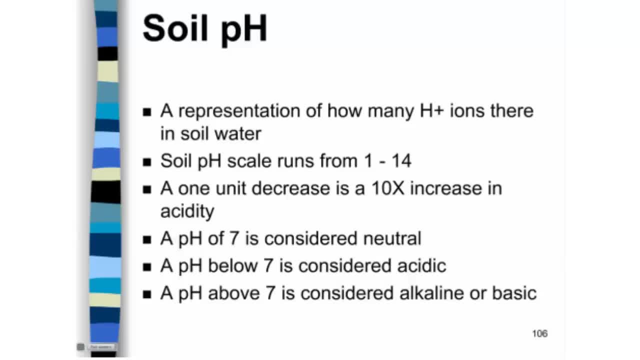 We've got good stuff plus a lot of this other larger package that we're applying, So it can be expensive. sometimes, Like I said, it releases nutrients slowly. That can be good or bad. If you want the nutrients released slowly so that something. 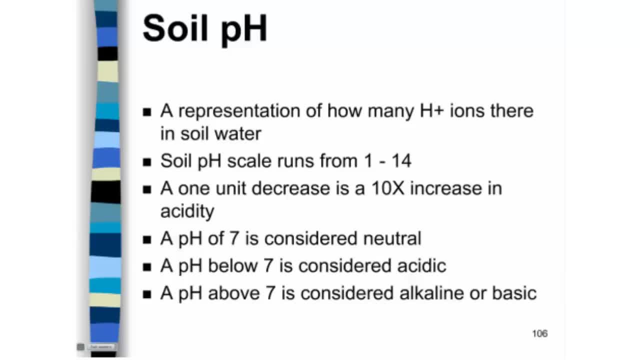 for instance, like nitrogen is being released right as the plant needs it. great. If you have a nutrient deficiency, though, organic material might not be the way to solve that right, It's going to take a while for that stuff to break down. 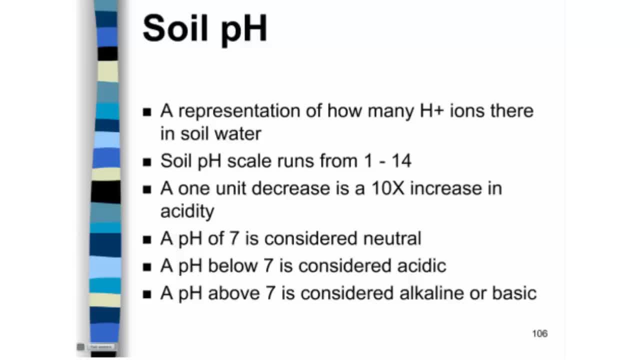 supply those nutrients to correct that problem. There's not going to be the quick fix with a lot of organic materials. These I really don't think about being that great a concern. health concerns I know people have talked about. we never use manures that are too closely. 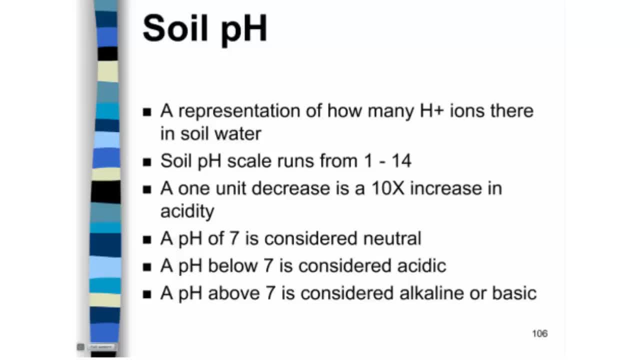 I think, related to things that are connected to us. For instance, you're not going to use pet manures or anything like that. And then also we have to be careful that there's not too much salt and those kind of things. Let's talk about advantages and disadvantages of inorganic 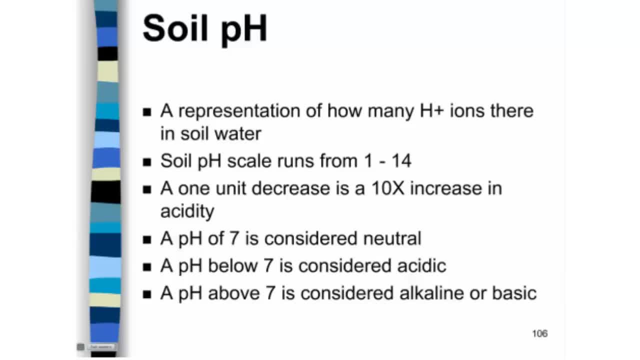 Well, you know, inorganic is pretty doggone inexpensive. in most cases It's produced in bulk. And because it's produced in bulk at a factory they can really decrease the fixed costs associated with that and the costs for you and I therefore decrease. 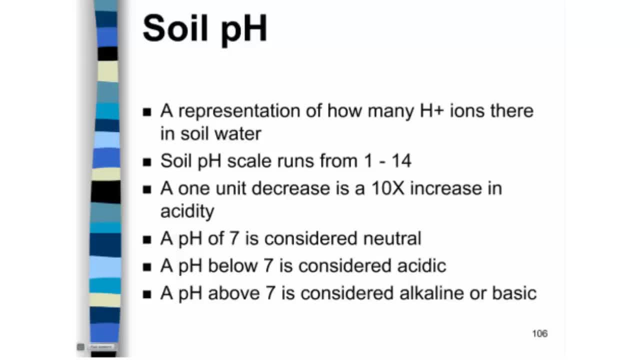 It's quickly released. That can be good or bad, right. If you want something slowly released like nitrogen, you may have to explore sulfur-coated products or something like that to decrease the release of that nitrogen. But it is quickly released. That can be a benefit if you have a nutrient deficiency. 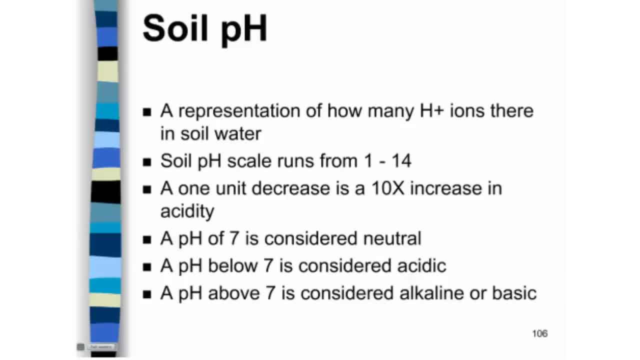 and want to quickly correct that. And inorganic does not do a lot to improve soil, tell You know we're not doing anything that's going to foster microorganism growth. We're not putting in any of these little organic glues that appear. 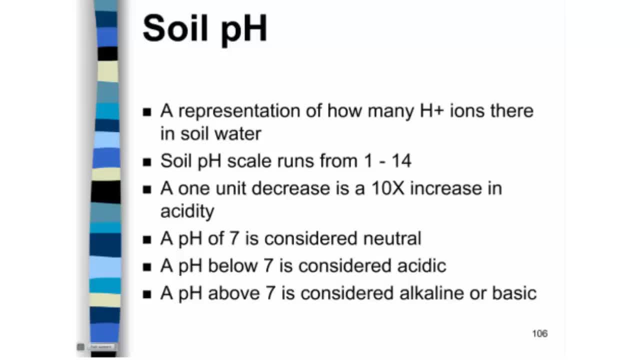 as things decompose. We're not doing any of those type of things that are going to maybe help out soil structure, that are maybe going to help out soil organisms, So it really doesn't do that. Next slide, please, Slide 124.. 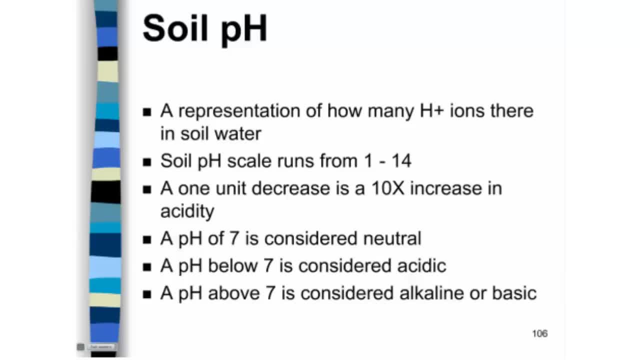 So here are just a couple rules of thumb. Rules of thumb for how maybe you could apply corn cobs or sawdust, or wood chips or leaves or some of these other things. You'll notice, for instance, something like compost, Instead of talking about a certain number of pounds. 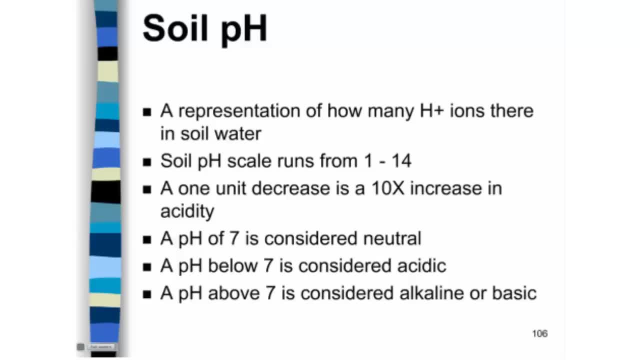 or a certain number of bushels. we're talking about so many inches of product laid over the top of the ground and then worked into that root zone. So what, Who cares? I showed you there was a great big breadth of organic products that could be applied. 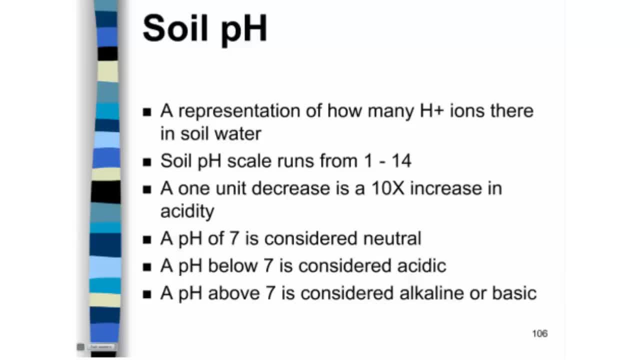 Why do we care about that though? Well, one reason is if you look at slide number 126, some of those products will require the addition of nitrogen. In particular, if you look at the next slide, some of those products that are a little more woody in nature. 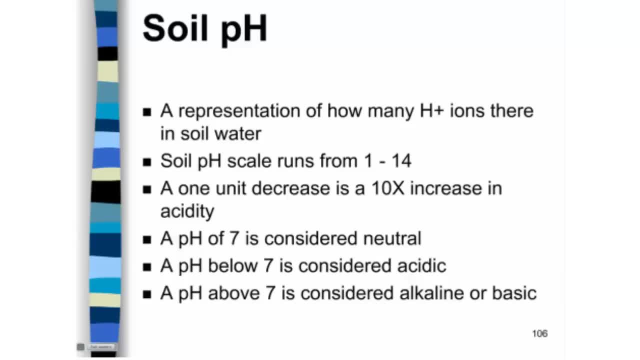 will require the addition of some nitrogen so that they can break down. You know, woody stuff takes a lot to break down. It's microorganisms that do that work of breaking stuff down. If we don't have enough nitrogen there, we aren't going to have enough microorganisms. 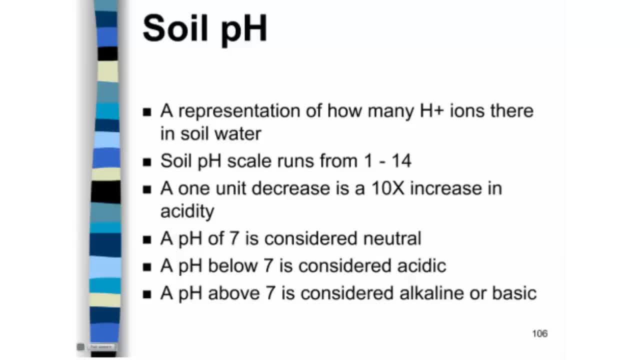 They're going to use that nitrogen to reproduce themselves to have enough workers to tear that stuff apart. If we don't have enough nitrogen and we have a woody material, those little microorganisms will start robbing nitrogen from the soil and use that nitrogen to reproduce themselves and chew up the stuff. 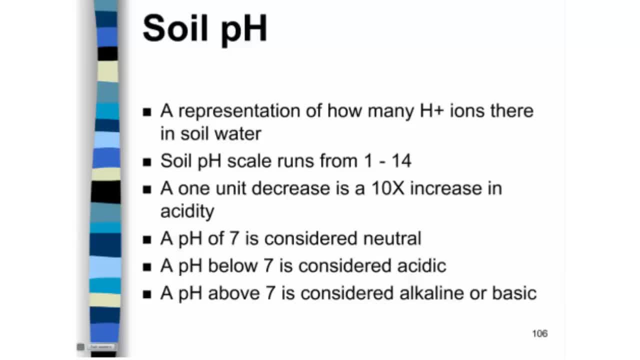 rather than your plant getting to use it. The other thing is that decomposition, releasing the nutrients that are contained within these woody materials, will really slow down if we don't add some of that nitrogen, if we don't create a situation where these little workers 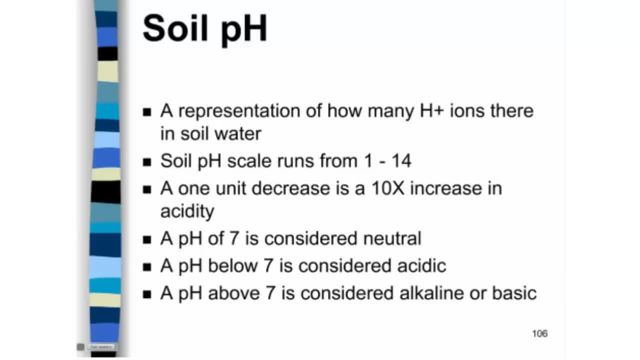 are produced in the kind of numbers needed to chew up that stuff. Any questions? Yes, Go ahead. I was wondering about foliar seedings, both the organic or inorganic, commercial, Like kelp and fish emulsion and that sort of thing. 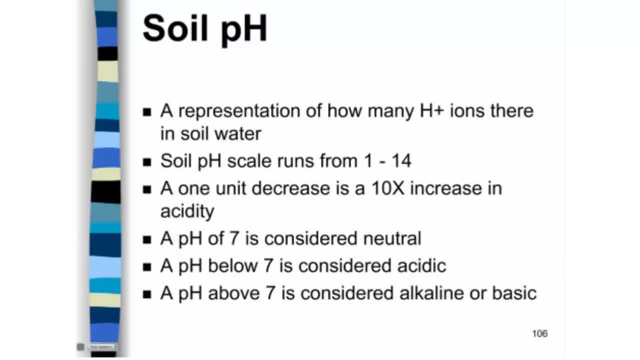 Is it safe on vegetables or not? To be honest, I'm not sure I can answer that one for you. Some of the people online right now who are more familiar with, for instance, GAP training and that kind of thing, can probably communicate that a little bit better. 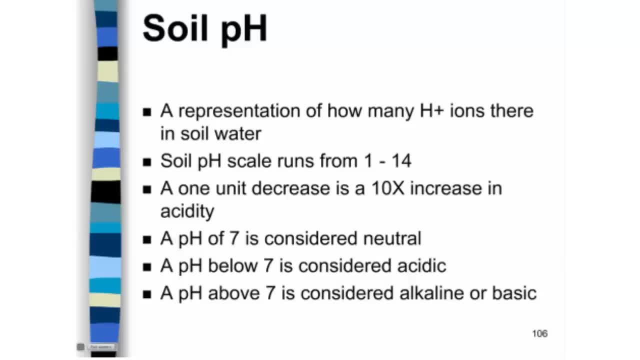 If I remember correctly, though, what you foliar feed with, you're going to have to be careful of. I think Ellen's probably on. She's up in the DeKalb area and she talks about being careful about compost teas, for instance, if it's something that could cultivate microbes. 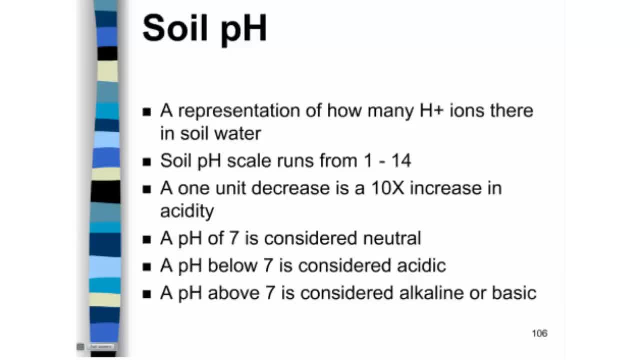 that could possibly be a problem Health-wise. you know we'd get a little bit worked up about that. Right, I wondered about those, But I meant the commercial ones, like the kelp and the fish emulsion. I wondered about those two, the commercial ones. 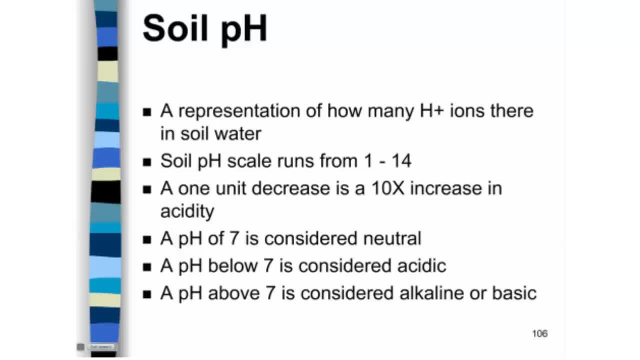 Yeah, Now, those I've heard of people using and they're perfectly effective. Like I said, I think you keep in mind your situation. you know if you need a quick fix on something, that's probably not what you're shooting for. 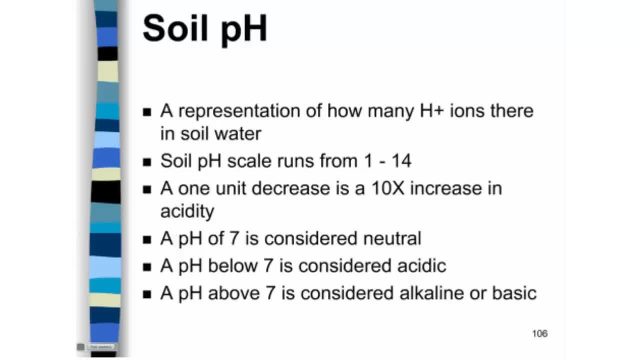 But you know, if you're not looking for a quick fix, those can be perfectly fine products to use Well. I've used them in the past in the large garden and it did seem to be helpful. but I just wondered about the safety on those for sure. 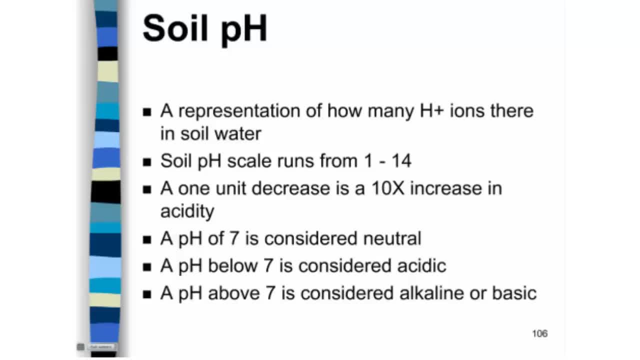 Yeah, And, like I said, I don't think that there's a health issue associated with that. But, to be honest, I probably need to double-check for you on that one. Okay, It's probably not an area that I'm as schooled in. 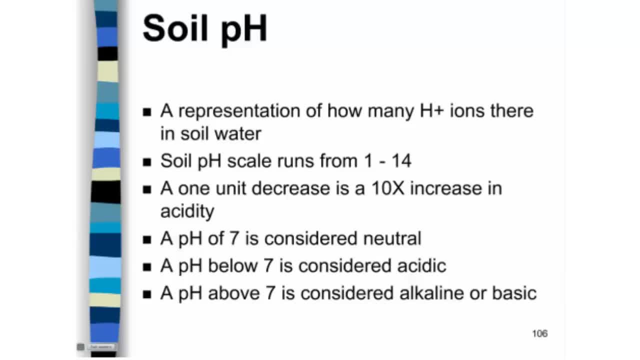 especially on the organic amendments. I'm probably not as schooled as some other people are. Matt, I can just respond a little bit in that. yes, when we, as far as the soil amendment goes, things like manure and so forth are excellent for improving soil. 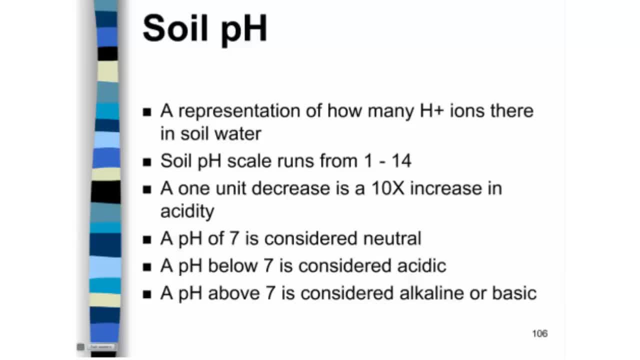 But when we do get into another topic- it was covered just a week ago, so- on good agricultural practices, where we're trying to keep microbial contamination out of our vegetables and fruit production areas, then that becomes more of a concern And the general guideline is that if you're going to use something you know, 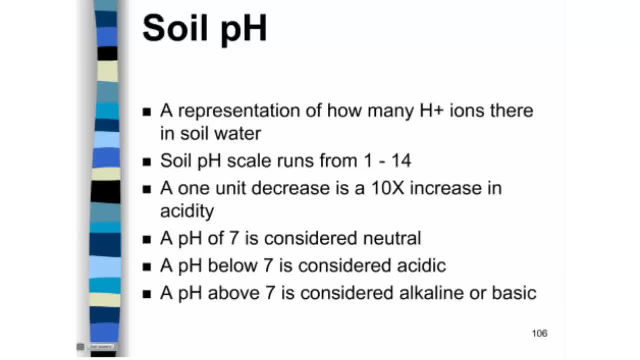 like manures and other things that have not been sterilized or, at least you know, treated well, even compost. if you're not sure it was hot composted, you know if it was only cold composted, then general guidelines are to incorporate that always, rather than putting it. 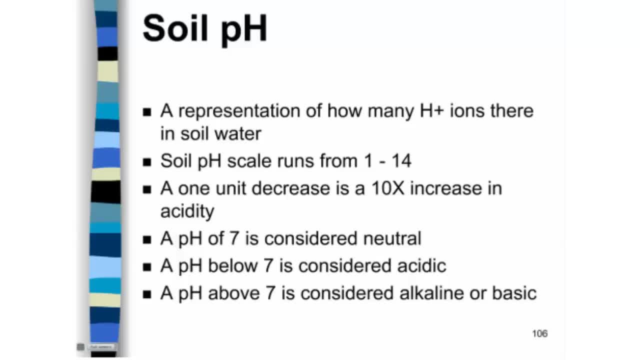 on the plant and to put it down 120 days prior to when you're going to harvest anything out of that garden that is edible, And at least 90 days prior to if you're going to harvest something that is, you know, further up the plant and not exposed to any soil splash. 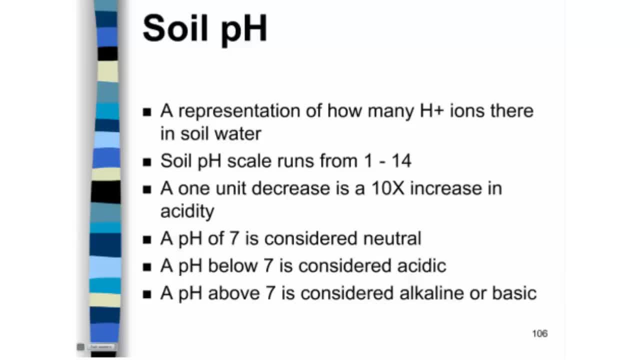 So those are the general guidelines on using any organic amendments in production. Okay, Thank you. Other questions And thank you Ellen. Ellen is probably the best person to reference or, at least in my experience, is one of the better people to reference on that topic. 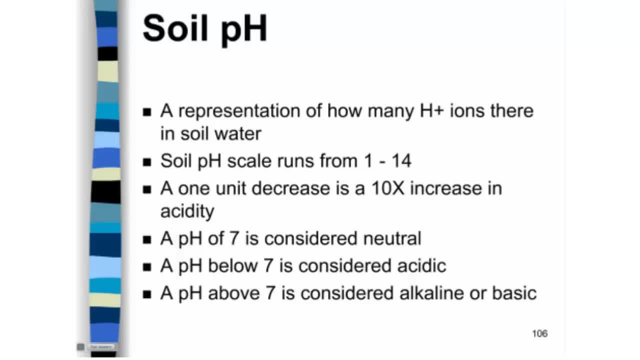 Hey Matt. Yes sir, Is biochar a nutrient? Yeah, Maybe you want to comment on that. And, in particular, what are you thinking on biochar James? What kind of questions are you thinking of there? Application just for soil fertility? 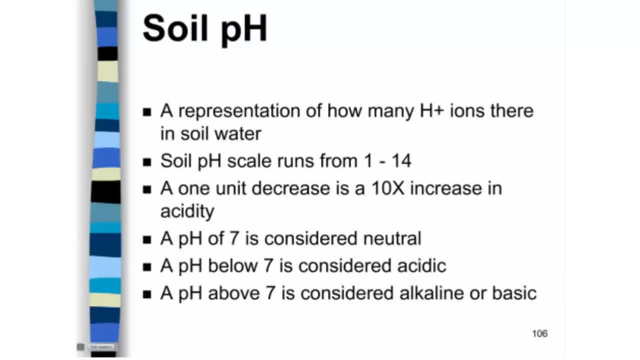 Is it one of the nutrients that we? is it a source of nutrients? Yeah, Now I think, one thing to keep in mind with biochar. I do think it can be a source of nutrient holding capacity, I might say, because it is going to add some of those little negative spots in the soil. 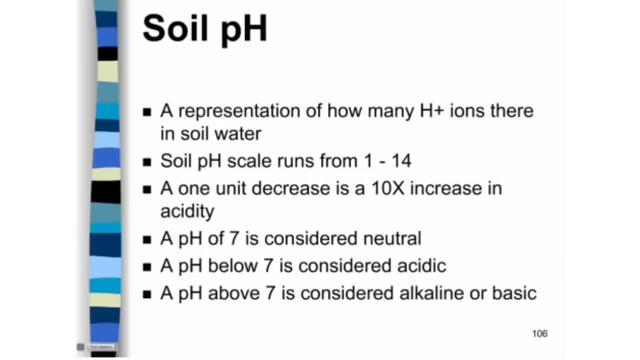 It can in some cases adjust CEC that we talked about earlier. I'll reference here maybe some, as I'm kind of going down the CEC route. I'm going to reference some work that Dwayne Friend from Jacksonville did on our irrigated growers plot. 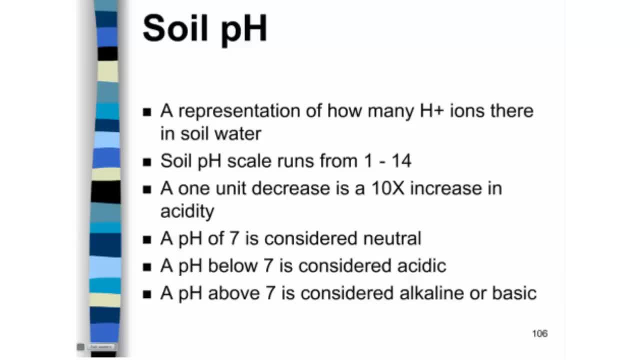 I do think there are cases where you can use an organic amendment to adjust your CEC, but I usually think those are in smaller areas. For instance, Dwayne Friend did composting. I know composting is not exactly like biochar, but there would be some parallels here. 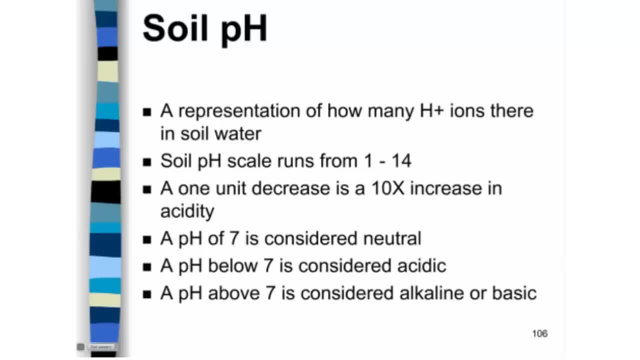 You know Dwayne did a composting study for a few years on our central Illinois irrigated growers plot and they basically applied that material again and again and again and all be they got organic matter levels to creep upward which means they saw some CEC benefit and that kind of thing. 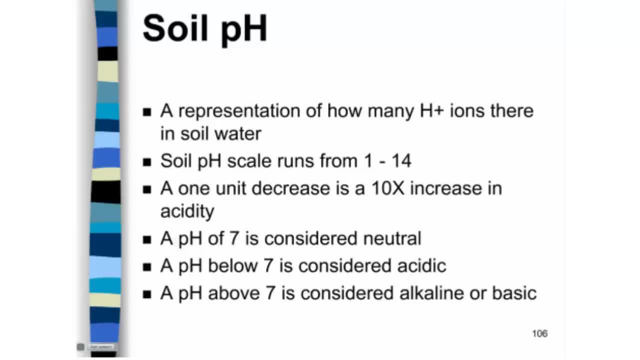 As soon as they stopped doing that, though, there was oxidation and the compost did degrade, I mean, the organic material did degrade back to normal. So I guess one of the things I would say- and I know this wasn't necessarily quite the direction maybe that you're going, James. 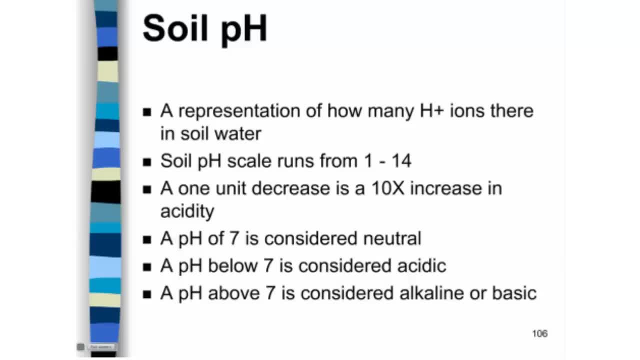 is when we're talking about adjusting organic matter levels. if you're going to create your own soil in a raised bed, yeah, you can do all you want there with an organic matter level. If you're going to add, maybe, some organic material, 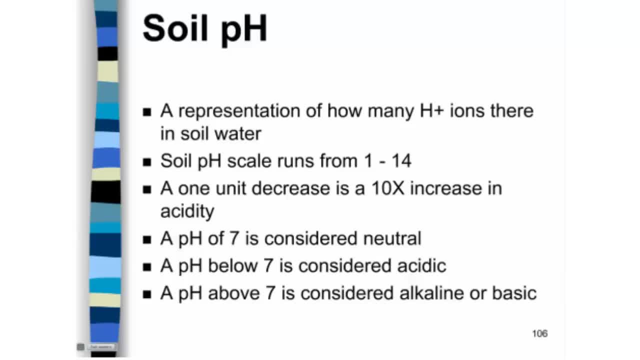 to a flower garden-sized area or maybe even a small garden. maybe you can do some things to adjust that organic matter and CEC level. I think on a larger field-wide basis, which is some of the people attending today, that sometimes becomes a little harder to do. 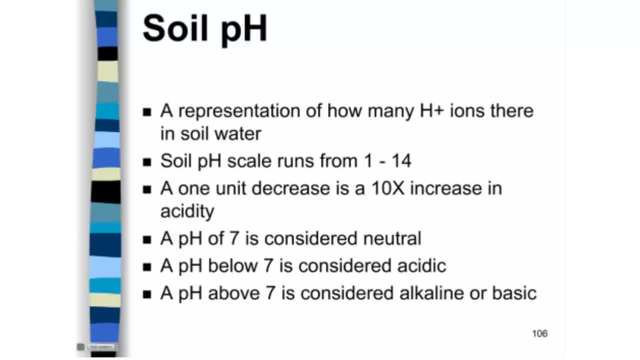 and we sometimes see this tendency to have things oxidized back down to normal after we stop applying that product. Incidentally, we are going to be doing a biochar study over the next few weeks, a study over here in Mason County. Dwayne Friend, who I mentioned, that did the composting work. 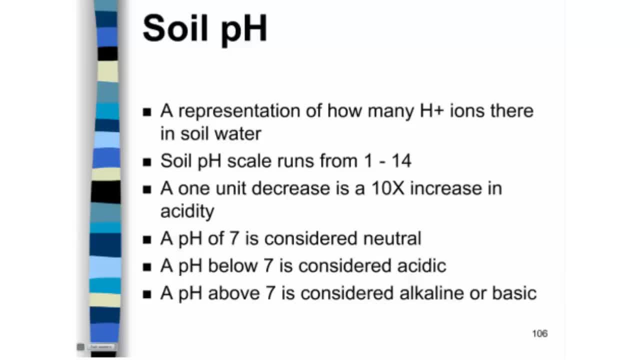 is going to be doing something on our irrigated growers plot on that. Thank you. Other questions? Yeah, is there a text that you could recommend for further information? Wow, you know, let me put a plug in for a good program. 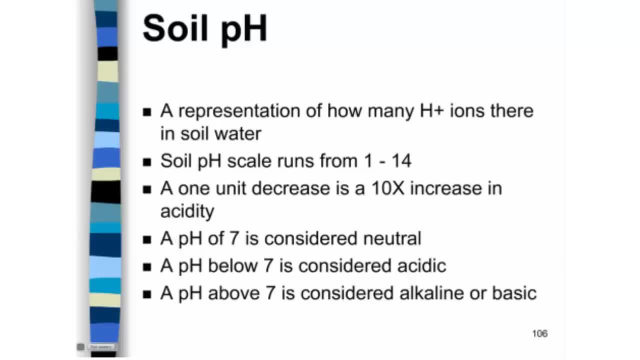 And then I'll try to think up a text here that would be a good one I would recommend to anybody maybe that's interested in this topic, or even local foods. I've noticed this in our area with some of our local food producers. 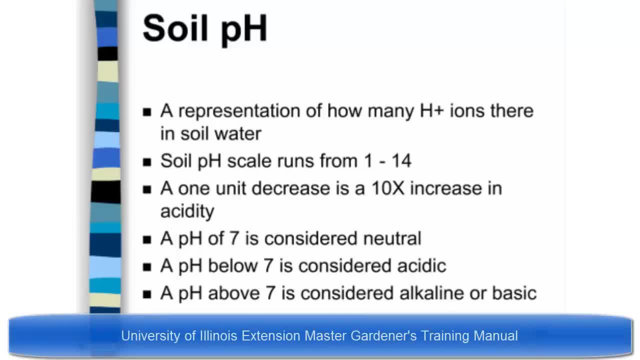 that they seriously consider the University of Illinois Master Gardener Program. You know, what I presented to you today is kind of an abbreviated version of what I tend to present at Master Gardener training, And that manual is a great resource. Now you only get the manual by being a Master Gardener in most cases. 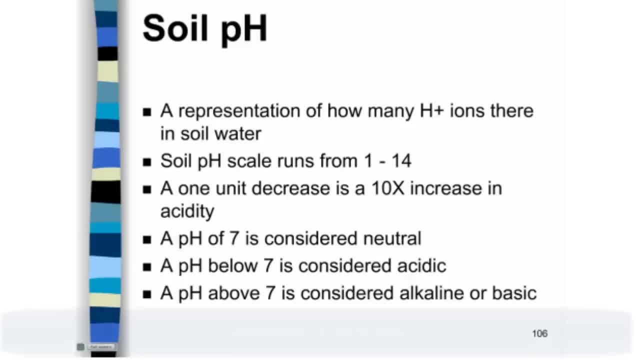 That would be one thing I would recommend. I do have a booklet in my office related to this. I think it's Fundamentals of Soil Science. It's not too hard to follow. I can't remember my author on that, though. Matt. 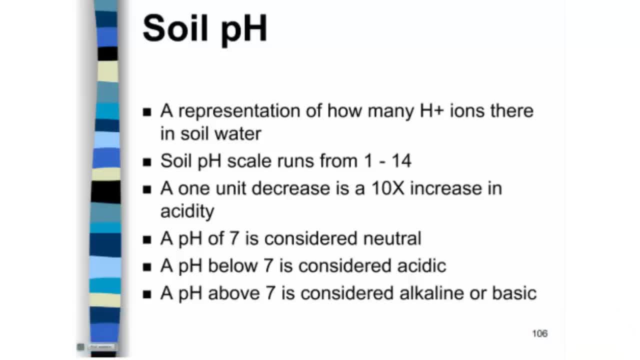 Yes, sir, Can I throw out another one? Yes, sir, There's a book called Building Soils for Better Crops- Sustainable Soil Management, And you can order that online from SARE, the Sustainable Agriculture, Research and Education. So if you just go to wwwsareorg, it's called Building Soils for Better Crops. 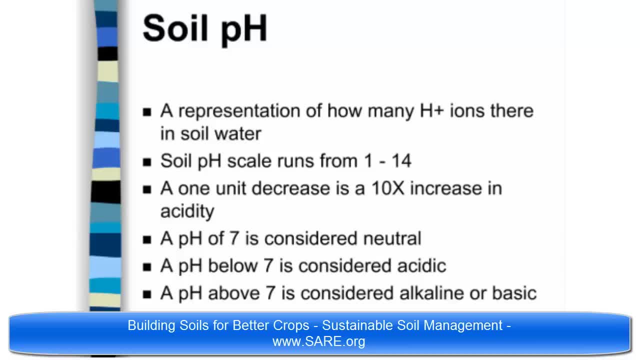 It's a great one, Okay, And what was the organization? again, SARE, S-A-R-E. Okay, The other extension publication, as excellent as University of Wisconsin, has a series on soil management. If you go to the University of Wisconsin publication website, it's a series of publications and it's really excellent. 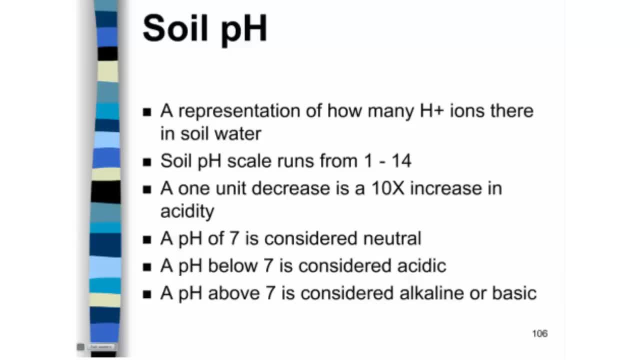 And Wisconsin soils aren't that much different, at least of Illinois soils, at least in the northern portion of Illinois, But the management principles there are described really well. Thank you, Are there some other questions? Yeah, May I have another one from Knox County. 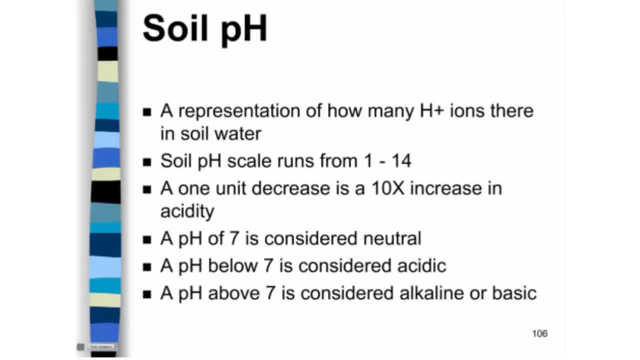 Yes, I was kind of wondering about particular P levels and K levels in certain vegetables. Do you have a recommendation there? Yeah, You know I think about the Midwest Vegetable Production Guide is a great resource for that one for how much P and K you need to apply. 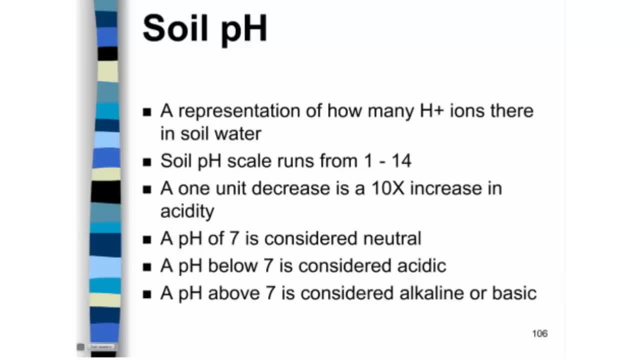 I'm trying to think: if I wrote down, I'm going to try to write down. I'm going to try to write down a few numbers here, just in case we got some questions. I don't have any right here with me, but that would be probably the better resource to go to. 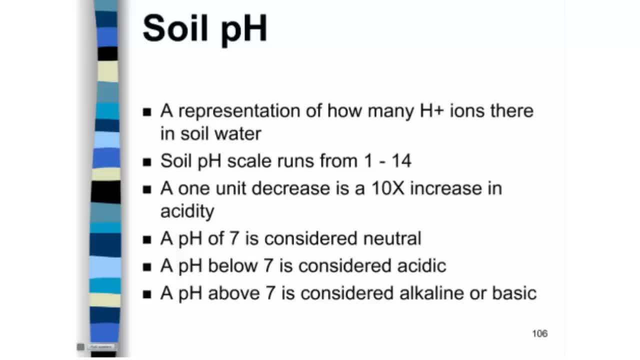 So it's going to be kind of specific from crop to crop about what you need to do, But you can't get too much P or too much K on Oh. okay, There's a good question: Too much P or too much K? 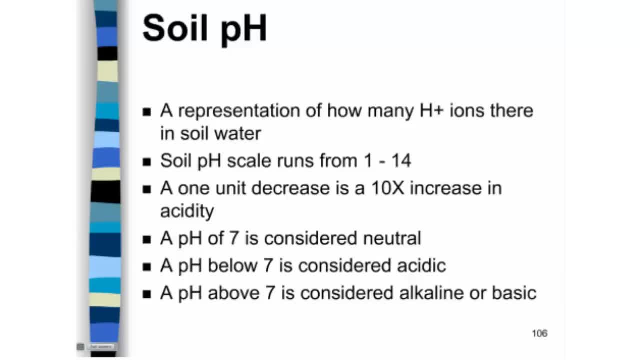 And what does the soil test need to look like? Okay, You know our P1 tests and that's usually the one that we look at for phosphorus. I know there's a little bit of a range there depending upon where you are in the state of Illinois. 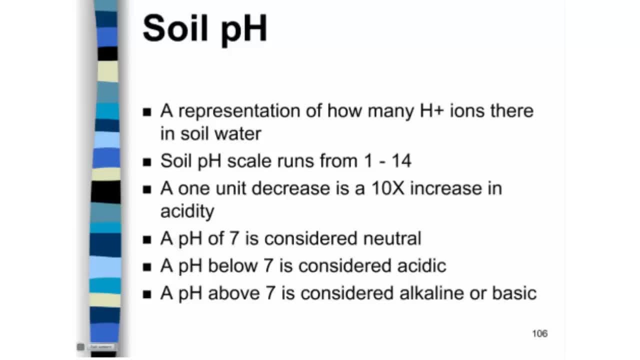 But in general if you're shooting for something in that 35 range, I usually think you're fine for your soil test level. Now it varies a little depending upon your location in the state. Your K test if you're shooting. 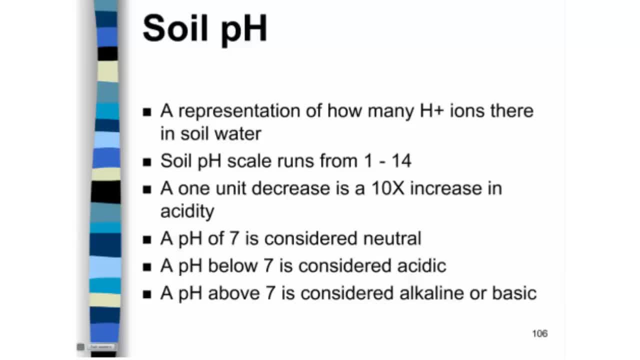 I'm talking pounds per acre folks, so forgive me on that one. So you'll need to adjust it a little bit. But your pounds per acre of potash usually like 250, maybe something in that range is usually pretty good. 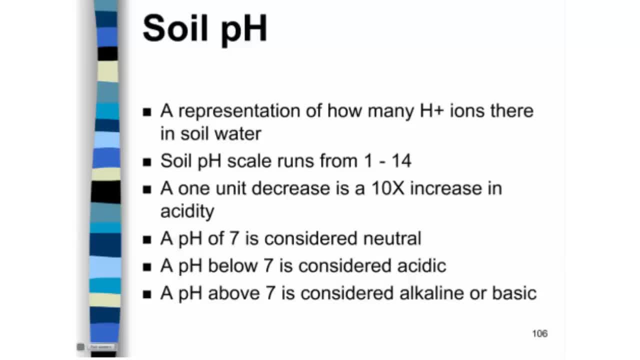 Can you get too much of either one? Too much phosphorus or too much potash? Now you can get. There are cases where we can apply too much of a nutrient. You can wind up with salt buildups. You can cause a problem with raising a crop. 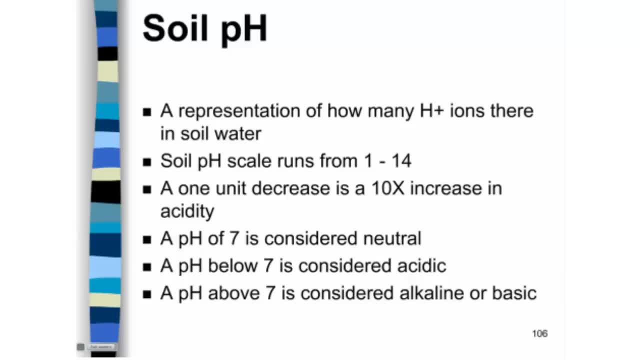 You get too much salt in the soil and it starts robbing the soil from that plant from access to water. It also can start robbing the plant itself of water. A good example of that: several years back I remember going and looking at a yard down in Springfield. 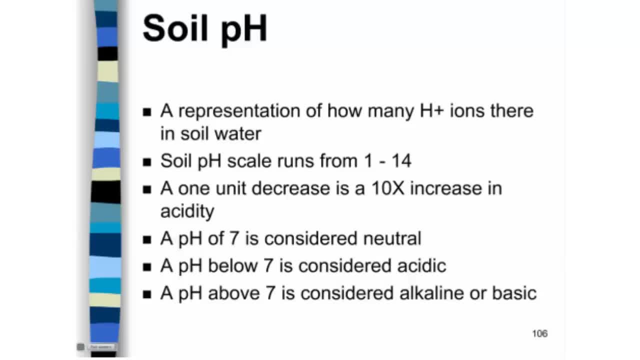 And the individual they were talking about. they thought it was a herbicide drift from the farmer's field And when we got out to look at their garden, it was a potash. It was a perfect dead square And they were picking up bucket loads- a couple bucket loads every year- of fertilizer from the dealership right across the way and just dumping it on that area. 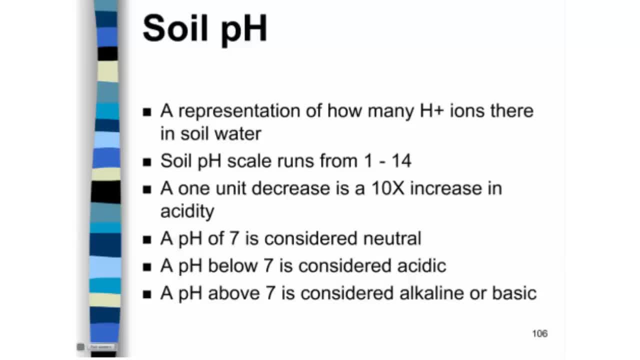 And that's kind of a reiteration of the point I made earlier- that you really want to use the soil test to guide what you do, because you can create some problems. Now are there some other issues with P and K? Can you have too much environmentally? 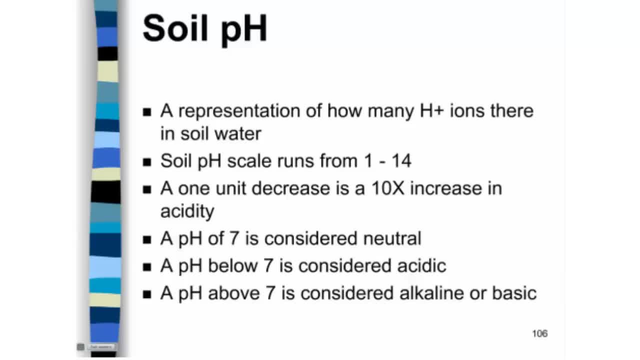 Yeah, you can. You know, with phosphorus in particular, you can load up the soil to a point that sometimes you can see some of that wash off with water. Most of the time we talk about phosphorus loss and contamination of water bodies really being through erosion and that kind of thing as a big way. 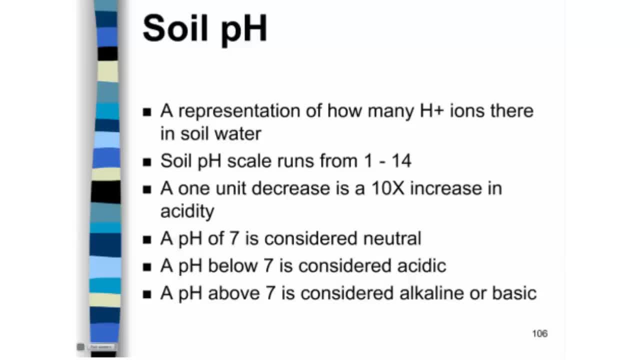 Potash. there are some people that get worked up about ratios of one nutrient to another. I think most of you in the audience are going to have a hard time screwing up those ratios. If you follow the soil test, in particular Potash, usually we don't see the environmental concerns that maybe we see with phosphorus. 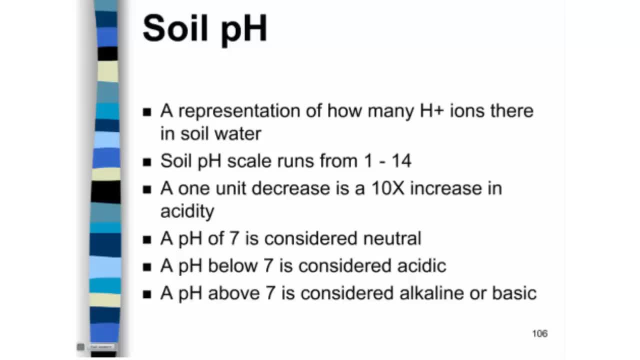 Hey Matt. Yes sir, If I want to grow blueberries that require a pH of 4.67 or something like that, I can keep adding leaf litter and stuff like that. Well, I would say that leaf litter would be a method by which you could acidify the soil. 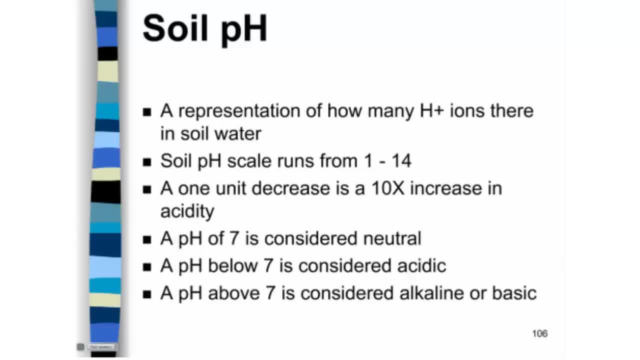 What I would say, though, is that soil test- Soil test- becomes important to figure out whether you're getting to that point that you want. Folks may or may not remember that blueberries and a few other crops are kind of an exception to our rule. 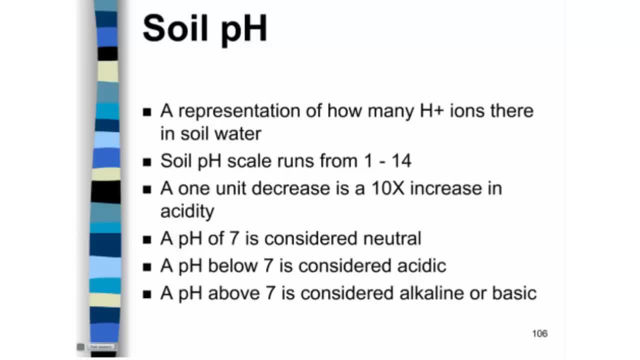 They like a little bit more acidic soil, And so you're going to have to acidify the soil to actually raise blueberries Inorganically. that can be done through sulfur compounds, And the soil testing company will actually give you an amount. 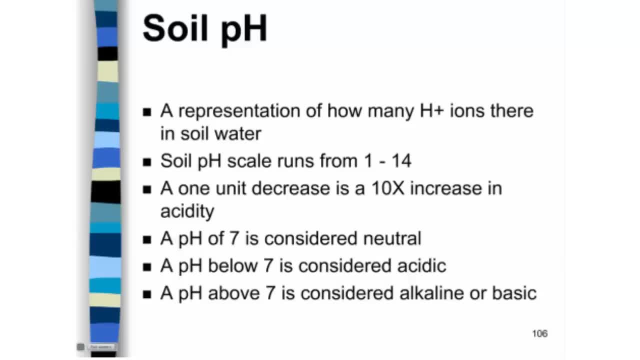 This is how much sulfur you need to apply. If you're going to try to do that with leaf material, it will take a long time to get it there. number one And then number two. you're going to make sure you monitor it. 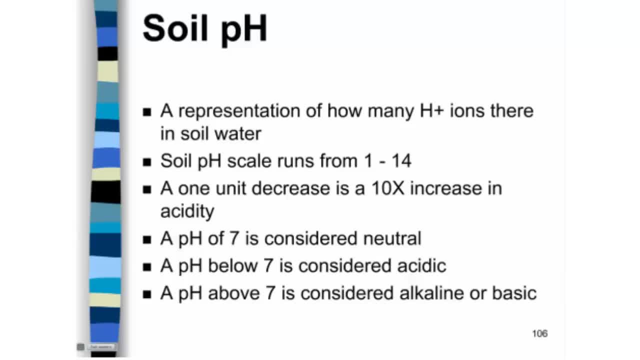 And I'd be monitoring it, I think, every couple years, few years- just to see if you're getting there Easier- unfortunately a little easier to get it real quick to that level of acidity with an inorganic material than maybe you can with just straight leaf material. 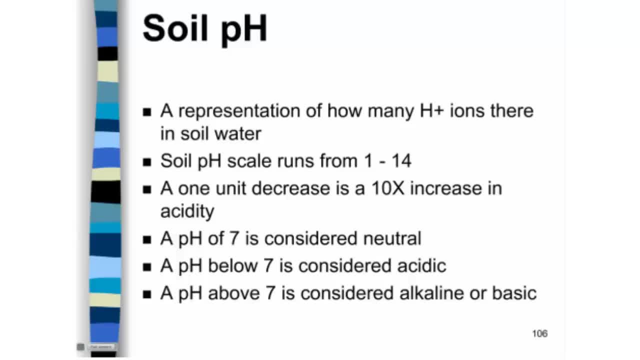 I see some other people have done this. Other people have mentioned. Deborah mentioned some things here. I think some of you may see this online about another good publication being Soil Biology Primer, And wwwswcsorg would be the location for that one if you wanted to find out more. 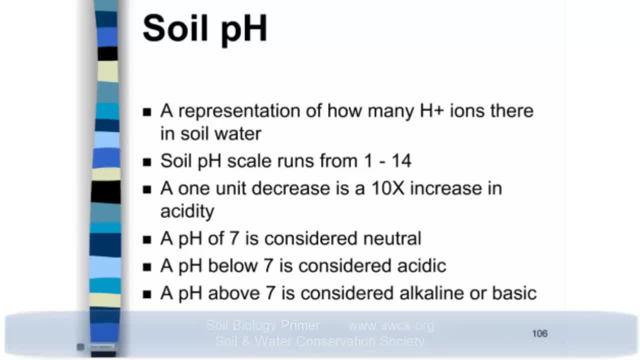 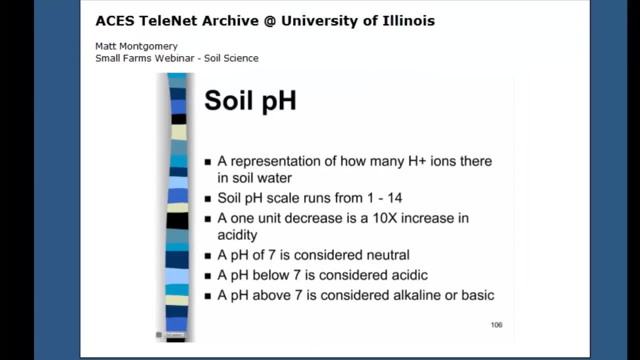 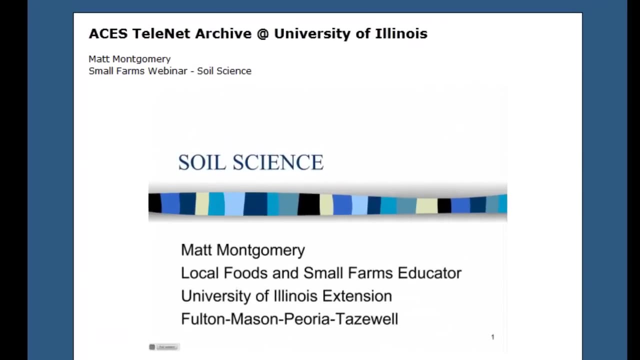 And that would be another good reference on soil science in general. Well, if no more questions, I guess I'm going to tell everybody a big thank you. I always appreciate the chance to get to visit with folks about topics like this. Not a lot of people around the office tend to sit around and let me talk about these kind of topics. 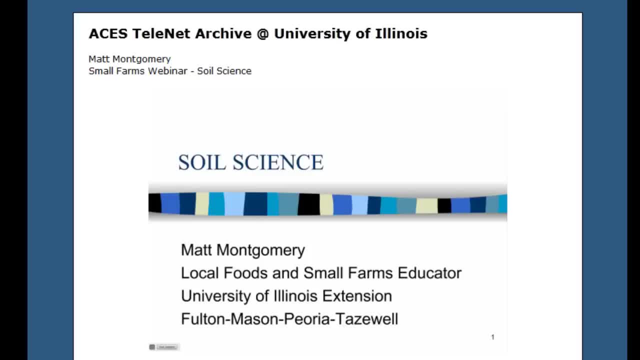 So thanks for giving me a little bit of time to visit with all of you. I hope it gave you maybe a little more of a picture of why things are the way they are with soil science, why we talk about PK and pH being what's important.